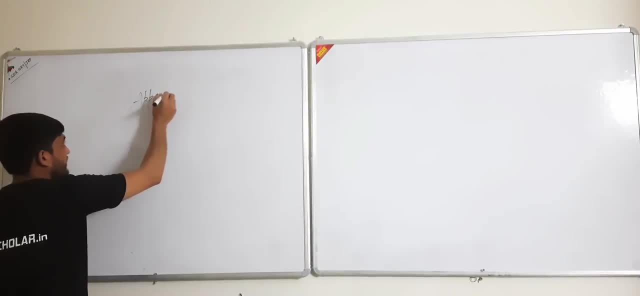 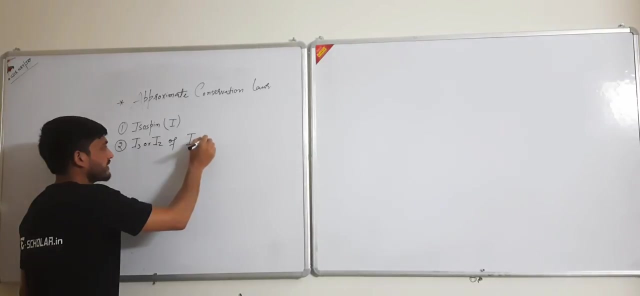 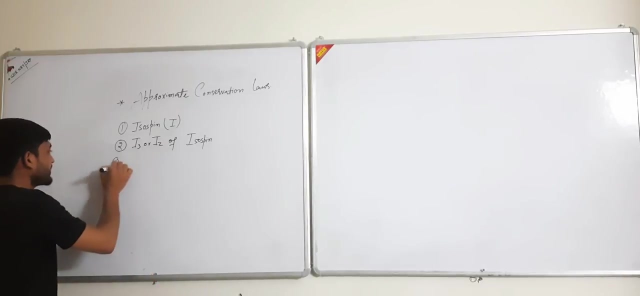 Approximate conservation laws, in which today I am going to discuss. First one is the isospin, isospin, which one is noted by I. Second one is the I3 component, I3 or Iz component of isospin, or we can say this is the third component of the isospin. Okay, now, after that strangeness, 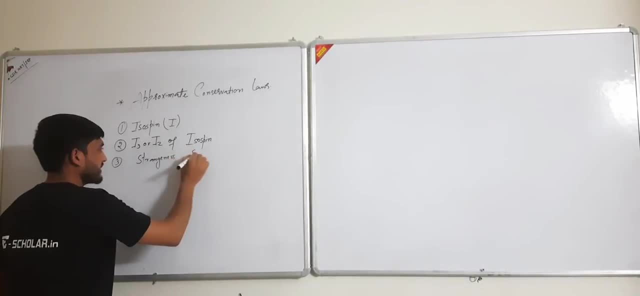 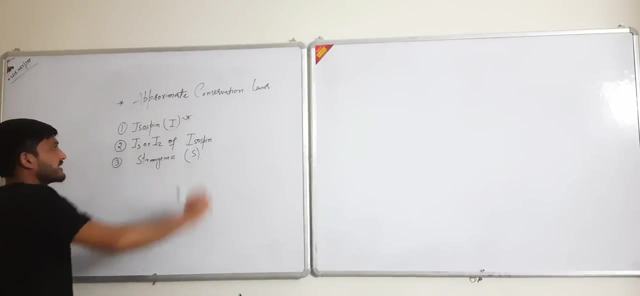 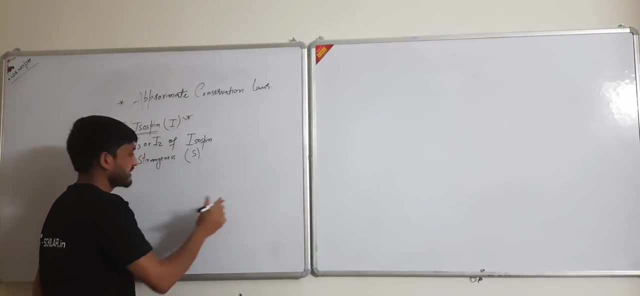 Strangeness is noted by capital S. Okay, so first of all, I will discuss about the isospin. Isospin- Before start this, I am. I will discuss about the nucleons. Okay, when we talk about nucleons, The idea of the isospin comes out when these nucleons in the nucleus 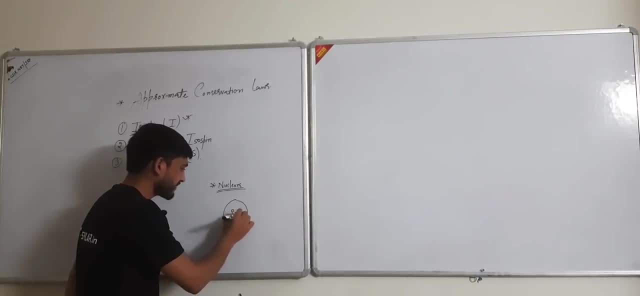 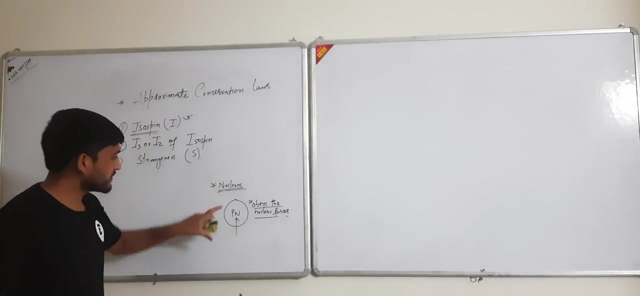 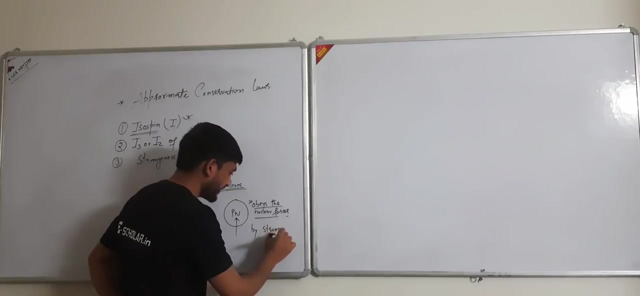 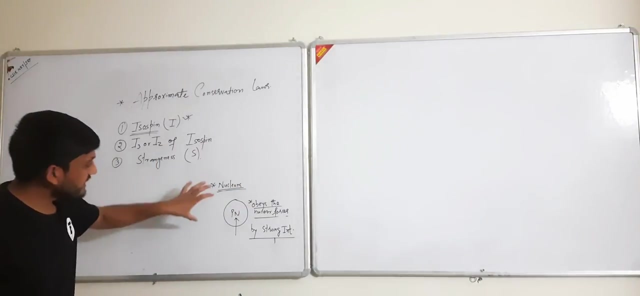 When these nucleons within the nucleus, just like in the nucleus, protons and neutrons- are the nucleons within the nucleus and these Nucleons obeys the nuclear forces and which are interacted within the nucleus by strong interaction, by strong interaction. ok, when these are interacted by the strong interactions. and 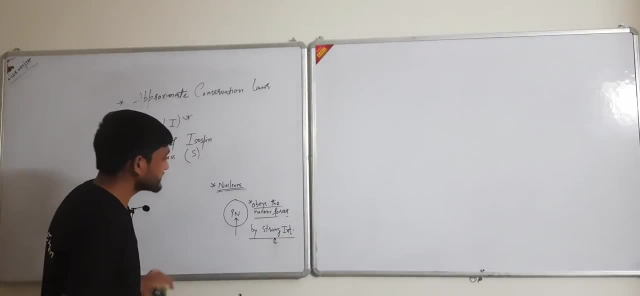 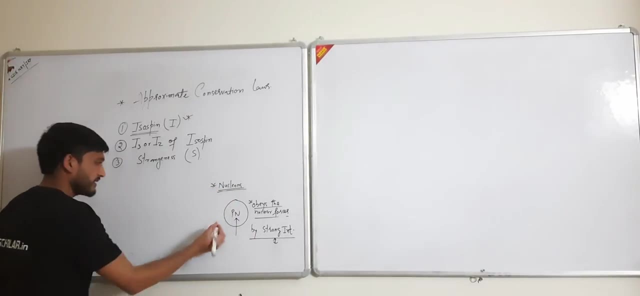 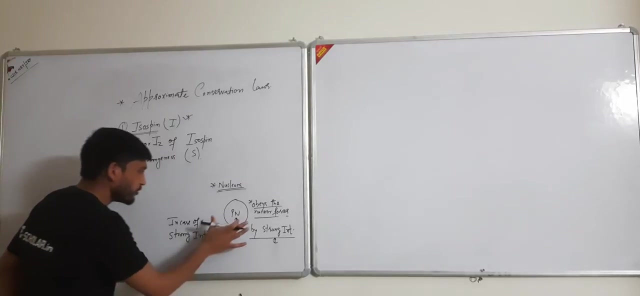 in this time, both these nucleons are of same entity. ok, when, in case of strong interactions- strong interactions- both these nucleons are of same nature. both these nucleons are of same nature are of same nature, it means they are independent of the charges. 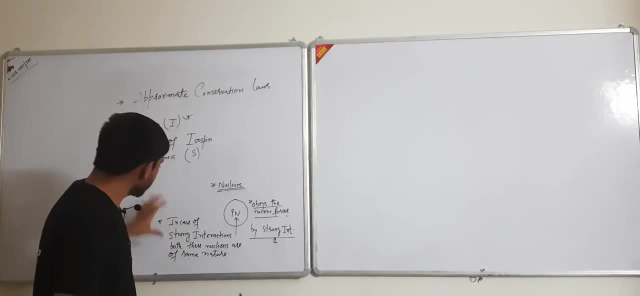 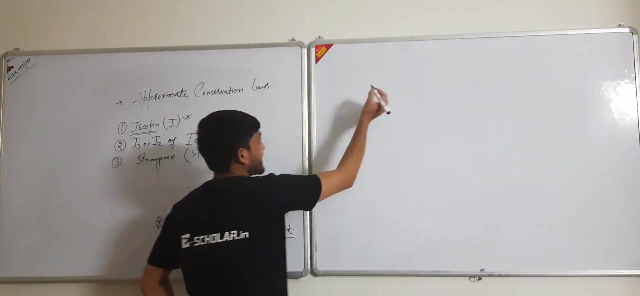 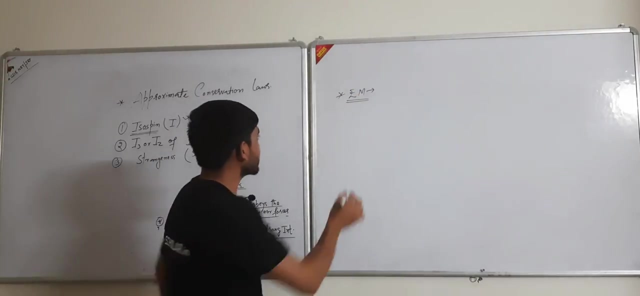 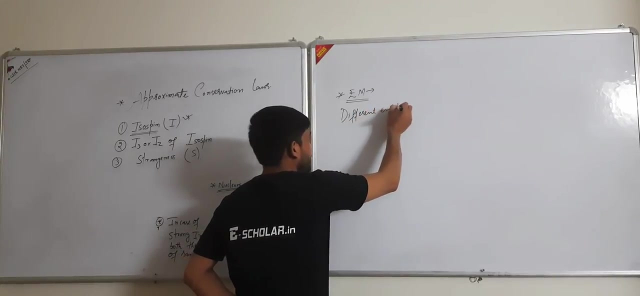 both can act as a similarity and when? when both are not. in the case of strong interactions like another is the electromagnetic interactions. in case of electromagnetic interactions, both act as a different entities, different entities on the basis of the charges. on the basis of the charges, okay. 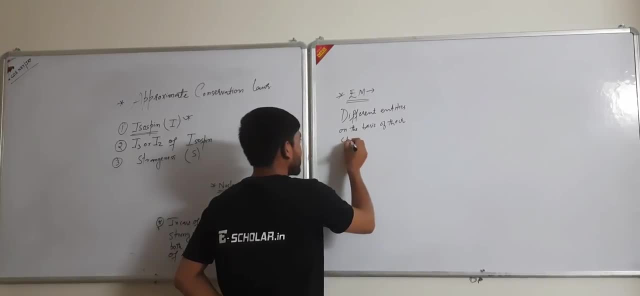 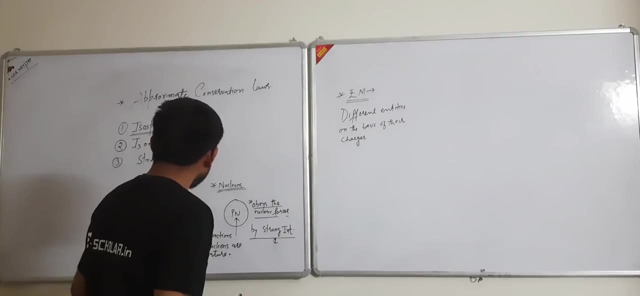 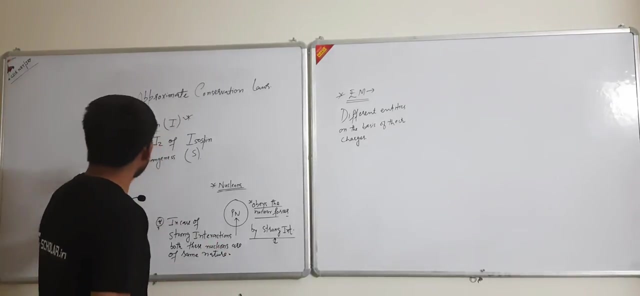 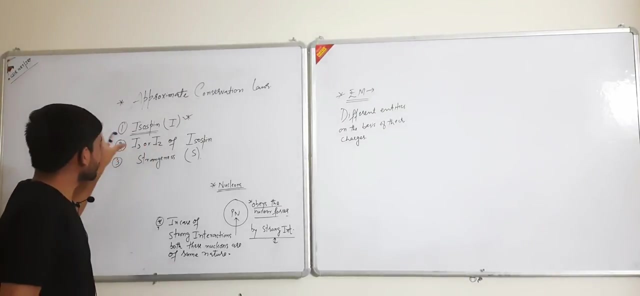 So this is the basic about the isospin: why the isospin are occurred and how, how the isospin are introduced. okay, Now next one is the method to calculate the isospin of the elementary particles. how we 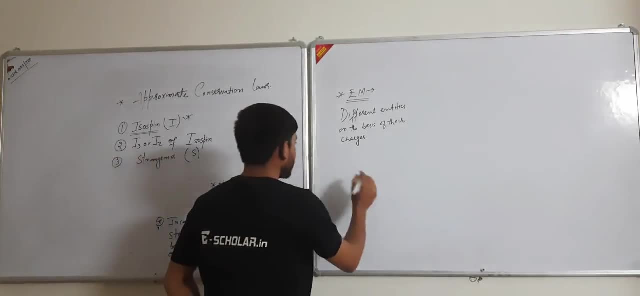 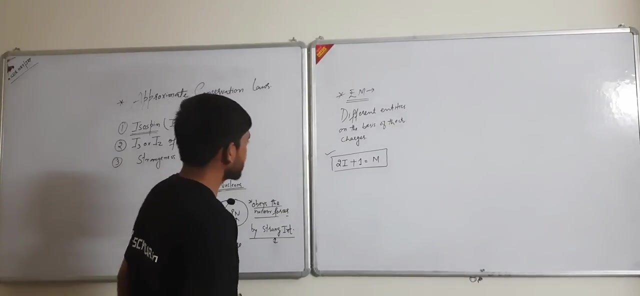 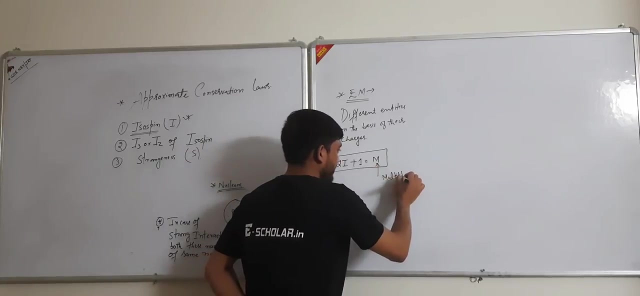 can calculate. okay, So we know that 2i plus 1 is equal to m. this is the formula to calculate the isospin of the particles. here m is the multiplicity: multiplicity of the particles, of the particles. 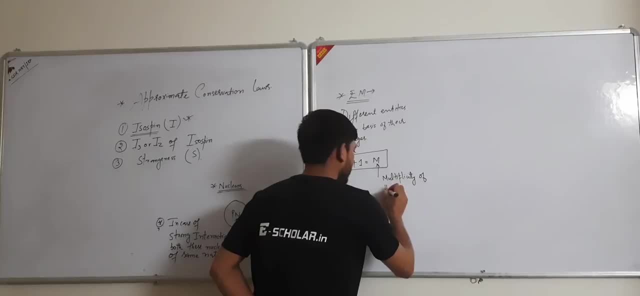 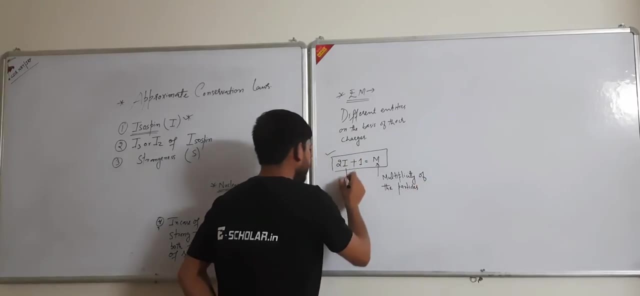 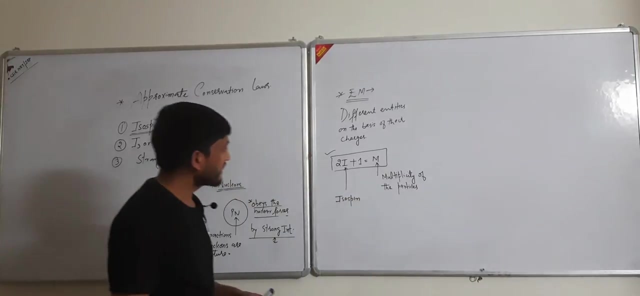 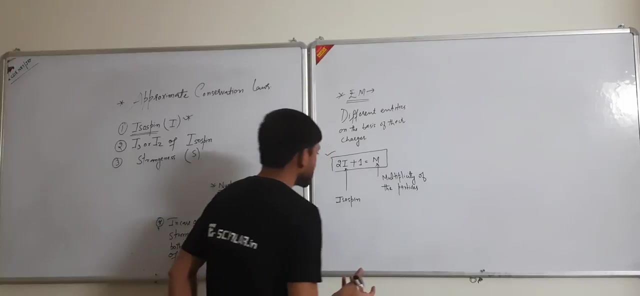 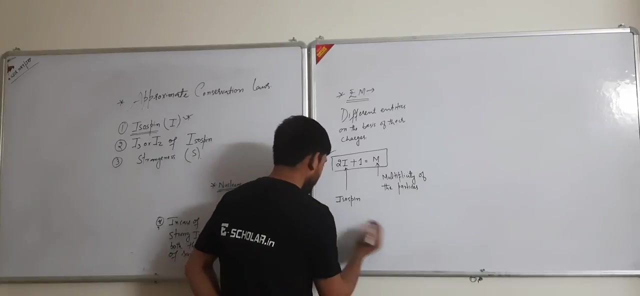 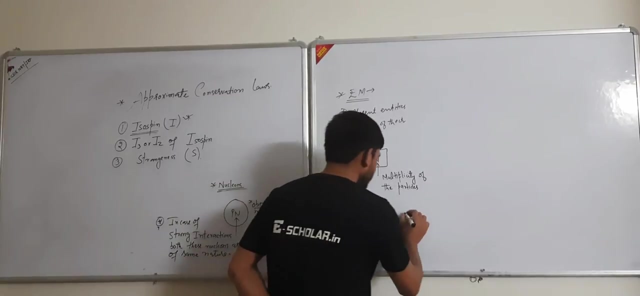 okay, Okay, Alright, Okay, and I is the isospin. okay now. next one is the how we can calculate the isospin of the different different particles. okay, like, first we will discuss about the mesons, mesons and then baryons. in mesons which type of particles are occurred, just like pions, pions, then kions, and third one is the neutrino, sorry neta. and in the baryons which type of the particles are occurred: nucleons and the hyperions. nucleons and second one is the hyperions. now let us start from the 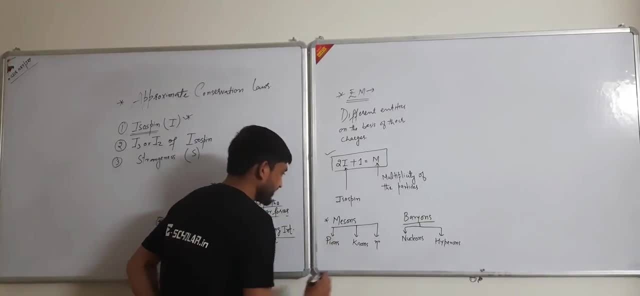 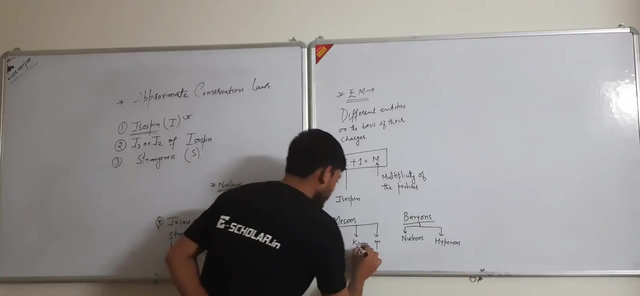 pions: how many types of pions are there? these pions are of three types: Pi poryteve, Pie negative and pie zero. kions, how many types? K positive, K zero, and this is the singlet. pions are the triplet and kiones are the duplet. 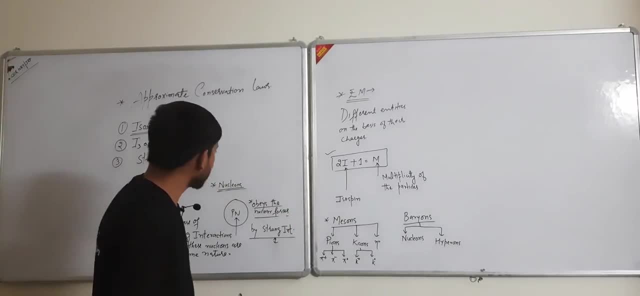 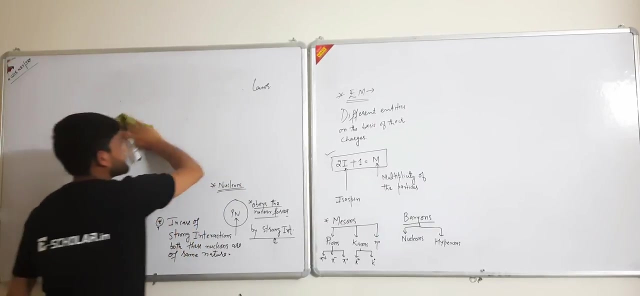 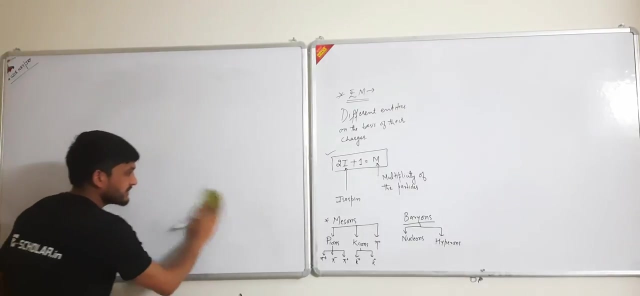 here eta is a singlet particles. Now how we can calculate the isospin of the these different elementary particles? Okay, Now let us start the start to calculate 1 by 1.. Here, first one is the mesons. 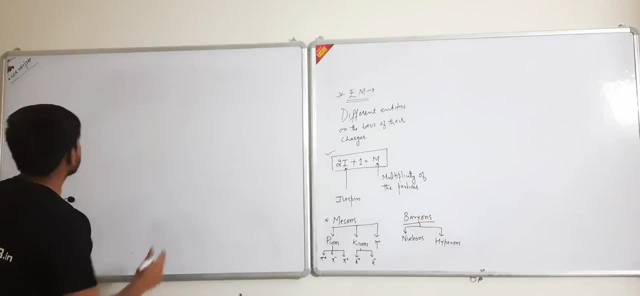 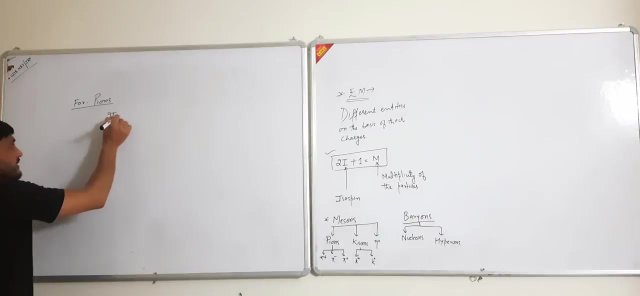 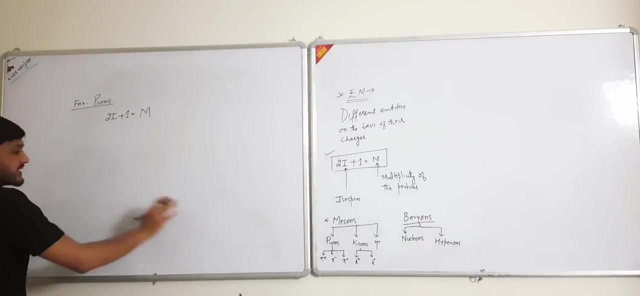 Or we can say that this is a pions for pions. For pions, 2i plus 1 is equal to m. m is the multiplicity and multiplicity of these pions. This is the triplet. For pions, 2i plus 1 is equal to 3.. So value of i will become: 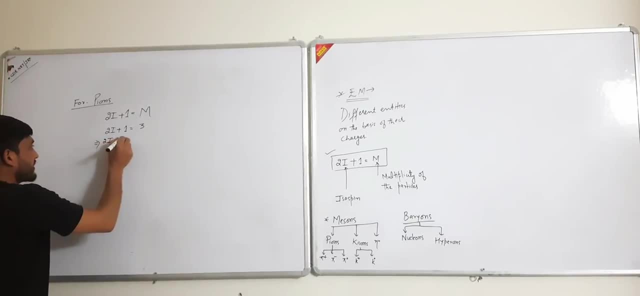 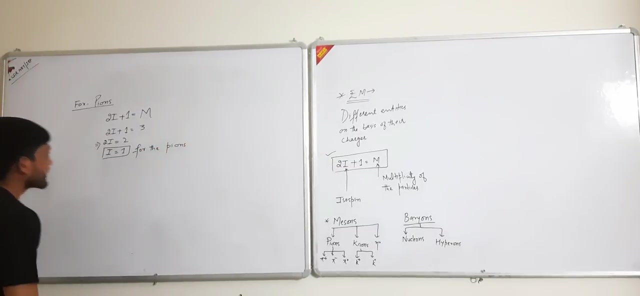 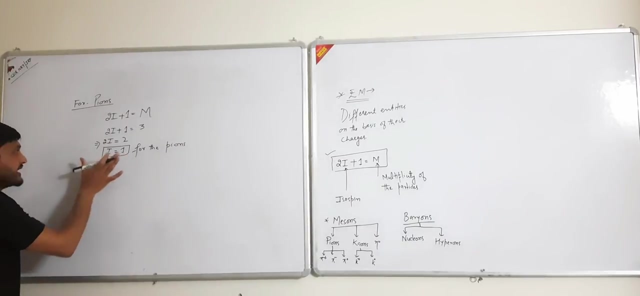 2 and i is equal to 1.. For all the pions- Okay. That means value of i. this is the isospin. i is nothing but isospin, and value of i will remain same for all the pions. Okay. And next one is the kaons. For kaons. 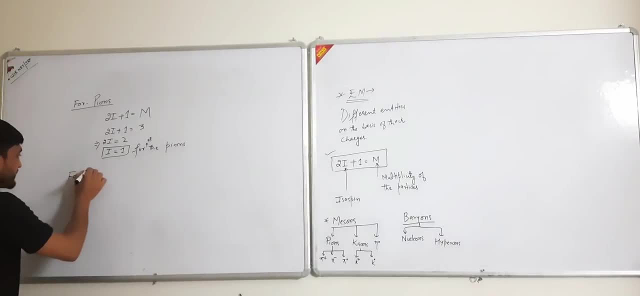 how we can calculate the isospin For kaons. value of 2i plus 1 is equal to m, where kaons are duplicate. What is this Duplicate? and here is the triplet. Okay, Now here value of m is equal to 2.. 2i plus 1 is: 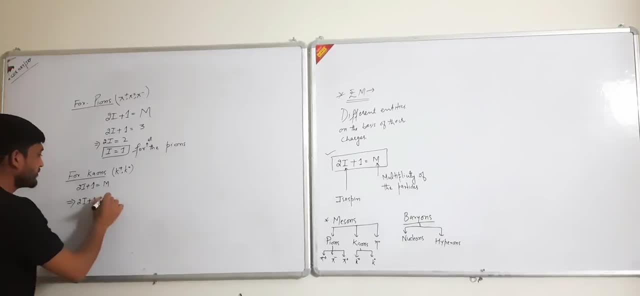 2i plus 1 is equal to 2 because this is the doublet and value of i, 1 by 2, and the isospin will remain will remain 1 by 2 for all the kaons. that means both the kaons have the same value of the isospin. okay. 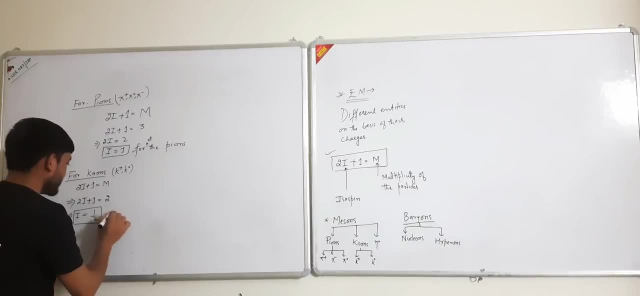 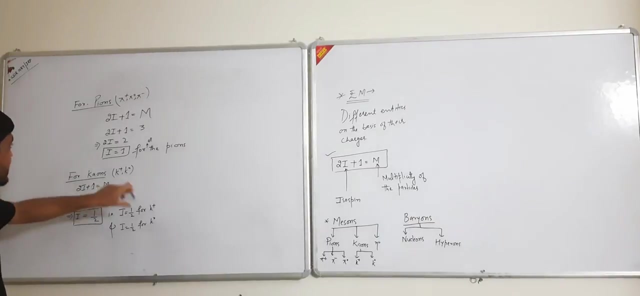 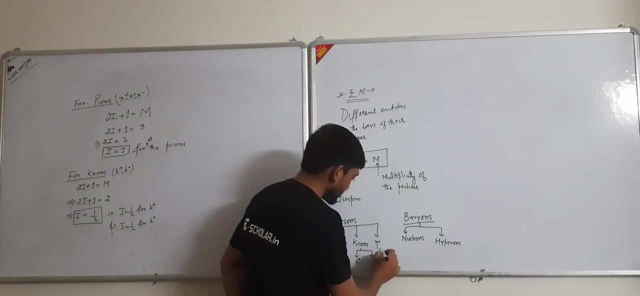 that means 1 by 2 for k positive, and i is equal to 1 by 2 for k 0. so this is the method for calculating the value of isospin. now, next one is the. just like this is the single at singlet. 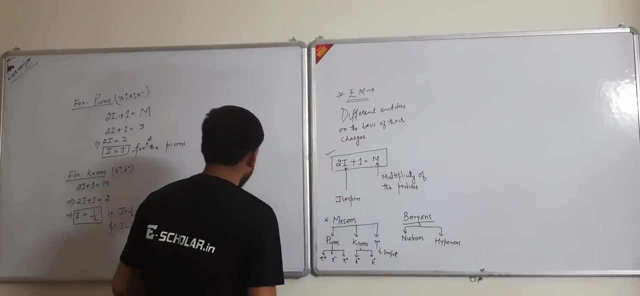 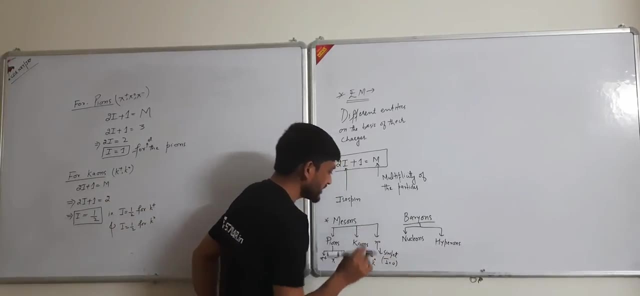 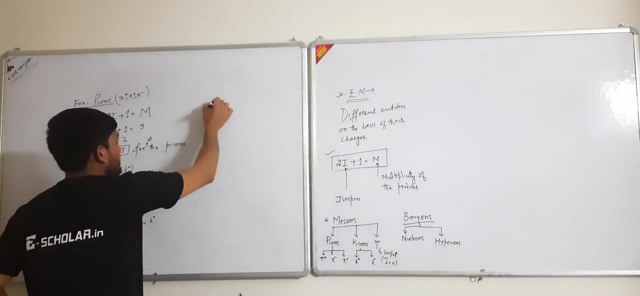 here value of m is equal to 1. then value of the isospin is equal to 0. here value of isospin is equal to 0. now i will discuss about the nucleons and the hyperions in the nucleons. for nucleons: 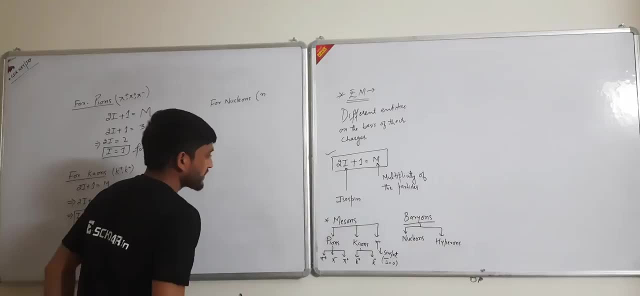 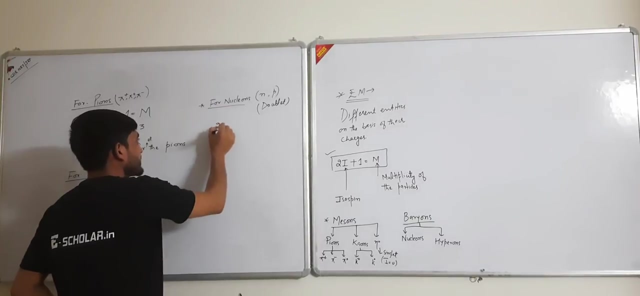 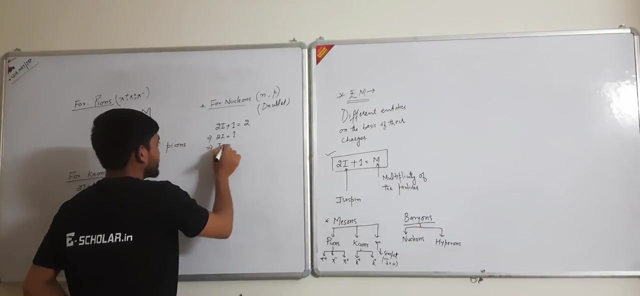 for nucleus. that means type of particles are occurred in the nucleus, neutrons and the protons. this is the doublet. doublet. okay for this, 2i plus 1 is equal to 2. then value of 1 and i is equal to 1 by 2. 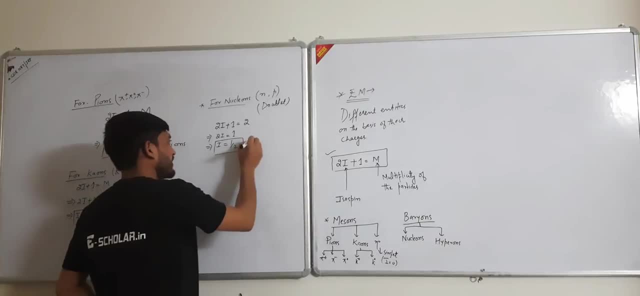 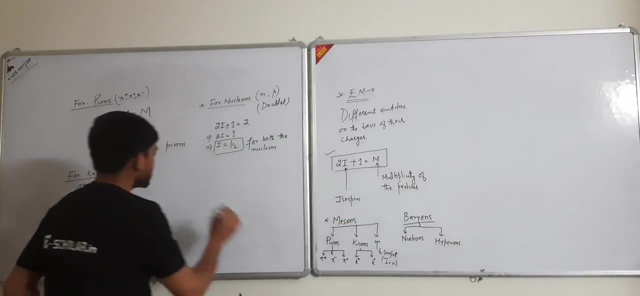 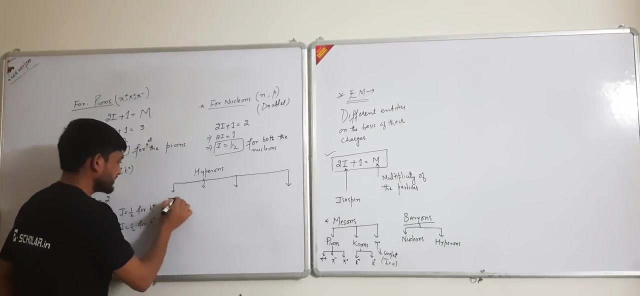 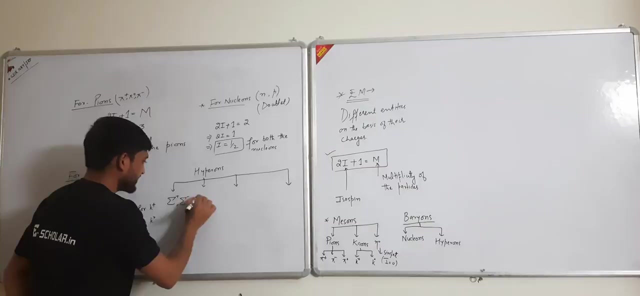 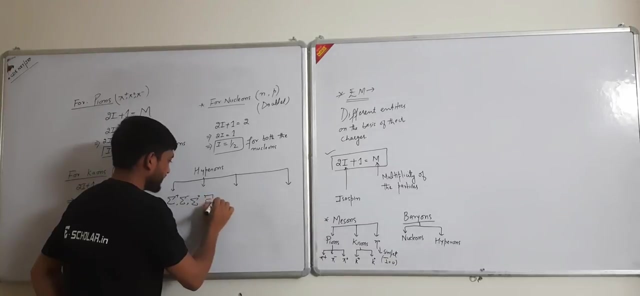 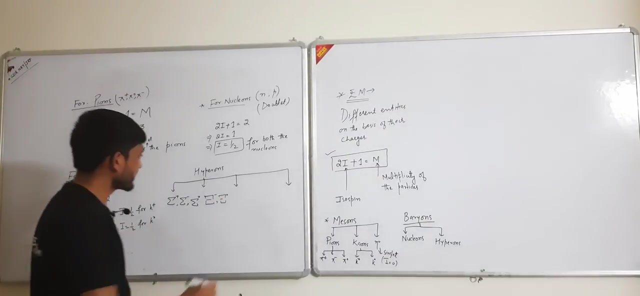 for both the nucleons, for both the nucleons. okay, so then for hyperions in hyperions in hyperions, which type of particles are in? hyperions are divided into four types. first one is the sigma positive, sigma negative and third one is the sigma zero, and then cascade negative and cascade zero. third one is the lambda and fourth one is the 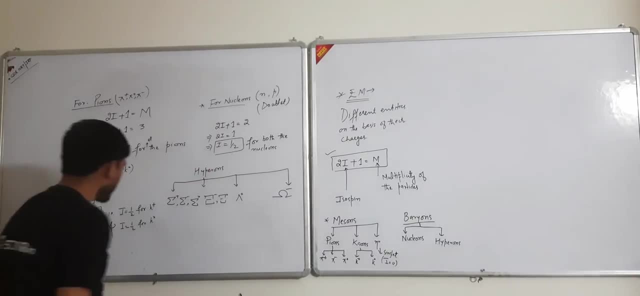 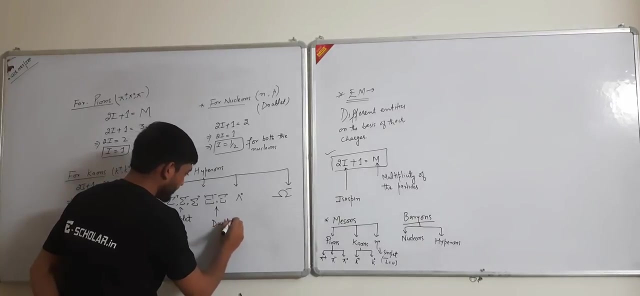 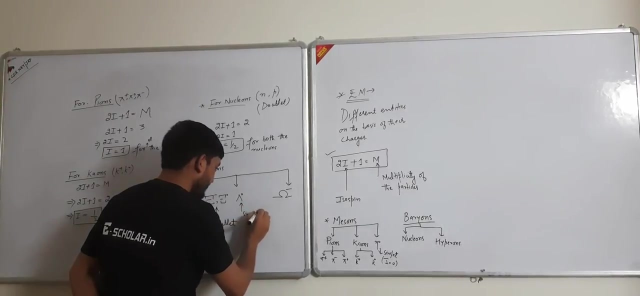 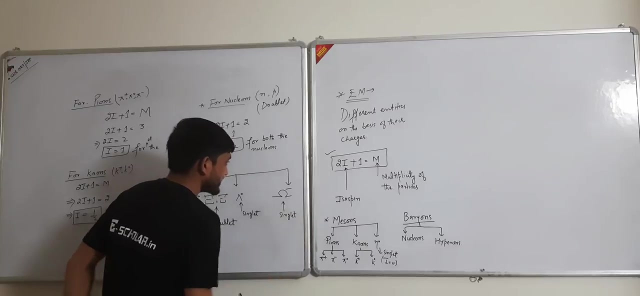 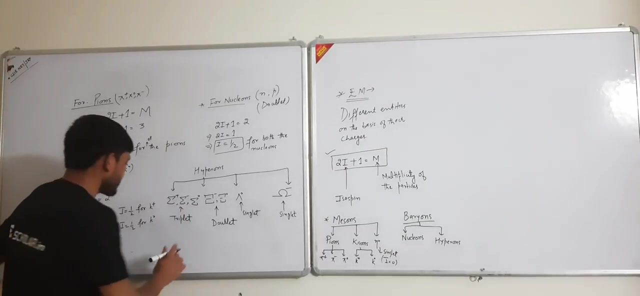 Omega negative. okay, so this is that triplet here. triplet cascade is the doublet, and this is a singlet. and 4th one is also a singlet singlet. okay now how we can calculate the isosepins for these particles too. I plus one is equal. 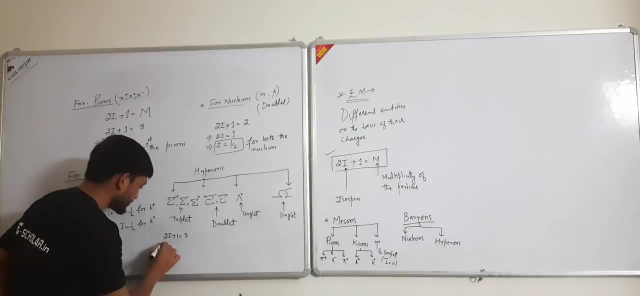 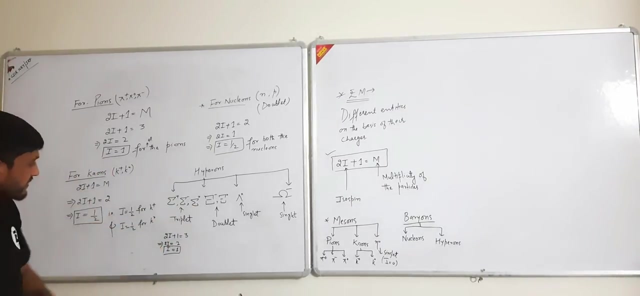 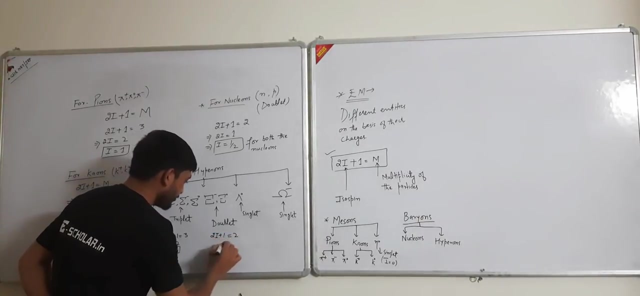 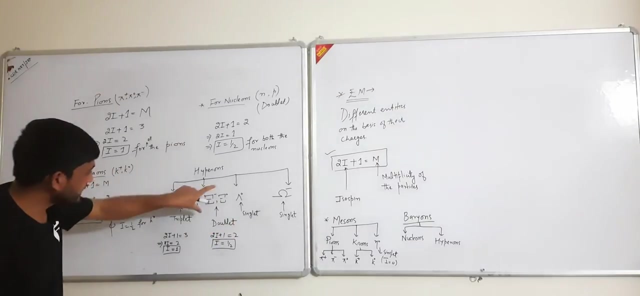 3, because this is the triplet and value of isospin 2i is equal to 2 and i is equal to 1 for all the these sigma particles and for cascade, 2i plus 1 is equal to 2 and i is equal to 1 for all these cascade particles. and 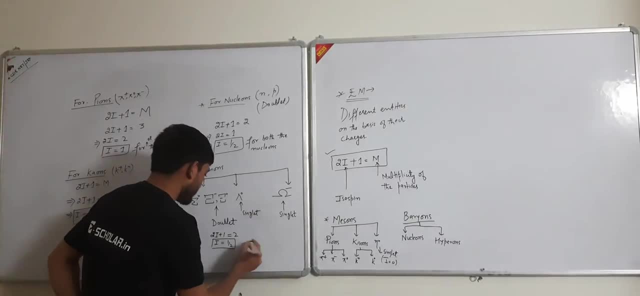 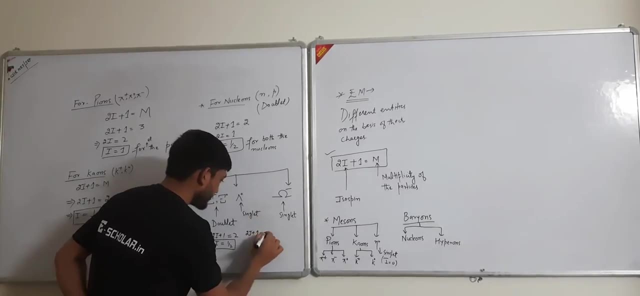 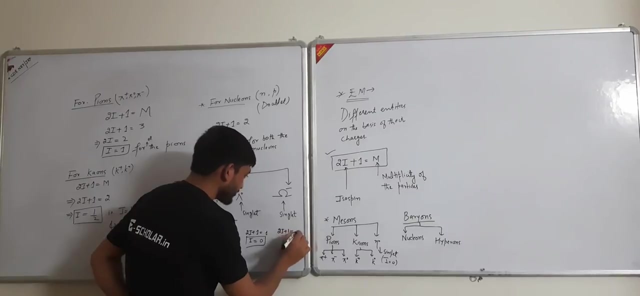 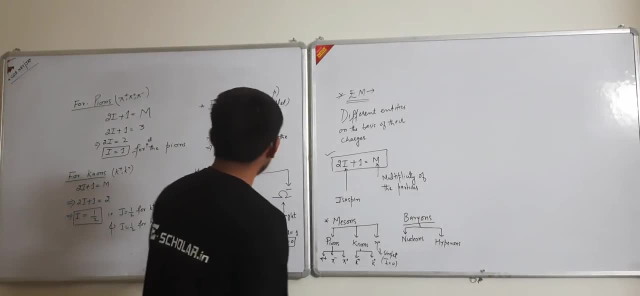 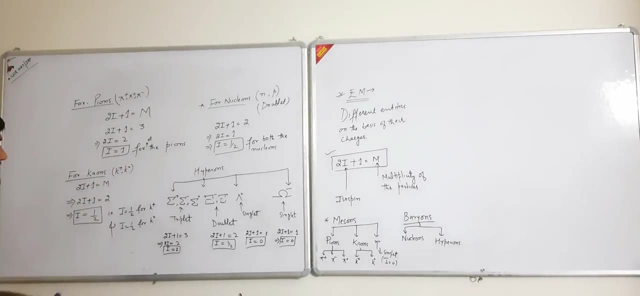 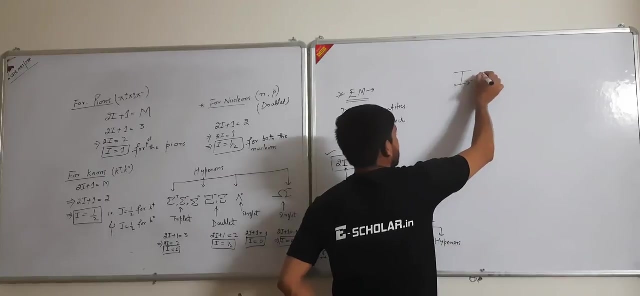 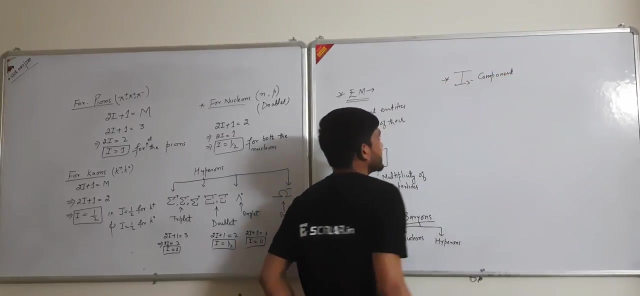 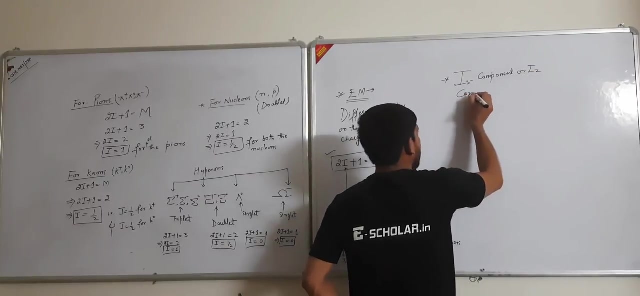 is the method how we can calculate the isospin of the elementary particles. okay now, next one is the i3 component. this is the i3 component, i3 component and how we can calculate the i3 component or iz component, iz component of the isospin. 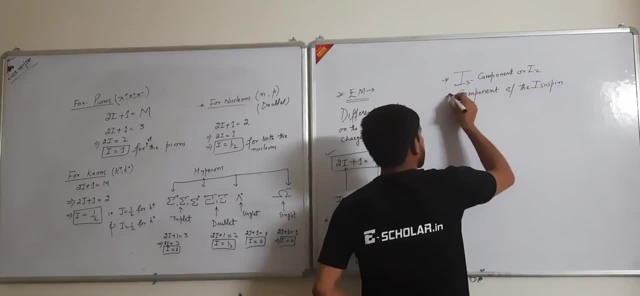 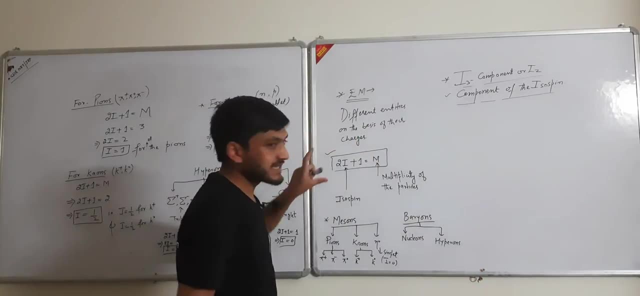 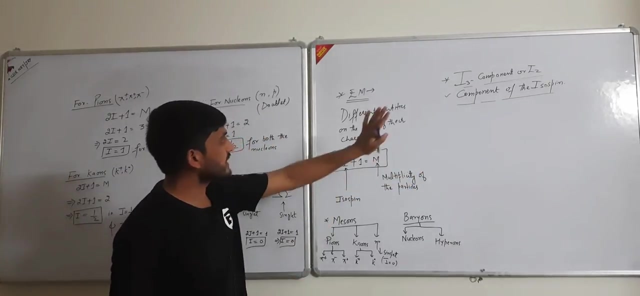 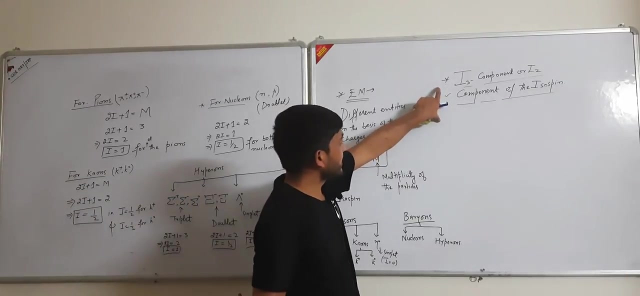 that means third component of the i4 spindle. okay, it means directions of the isospin in any particular or in any particular axis. this is the third component of the i thing related by I said and how we can collect i3 component other of these various difference between relevant particles. 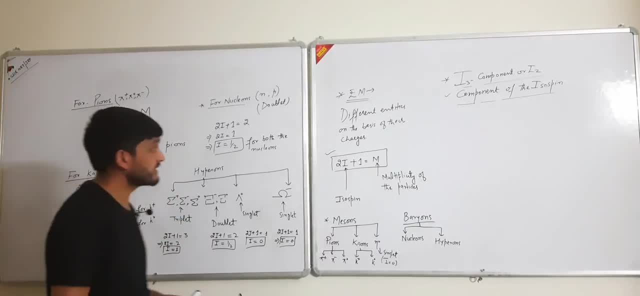 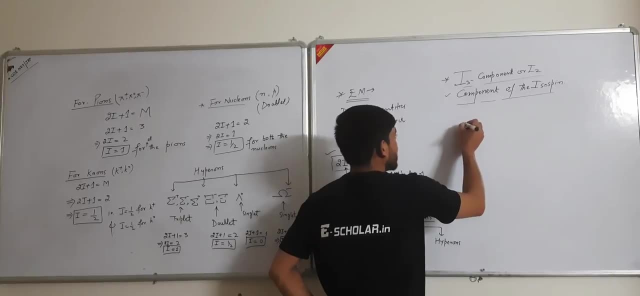 like hypraeons, nucleons, cairns and pions, and that is all. So this is the formula minus i to plus i. value of i3,. okay, This is the formula. Value was started from the minus. 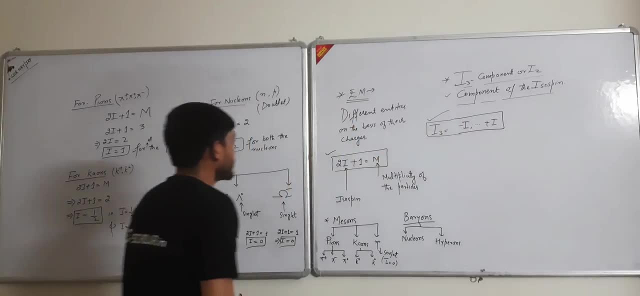 i and moved over the plus i. So from here for pions. this is the formula. So this is the formula. So from here for pions. this is the formula. So from here for pions. 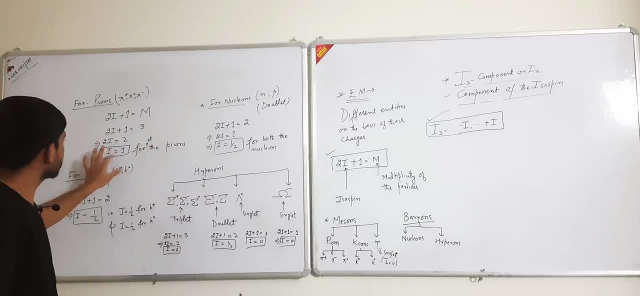 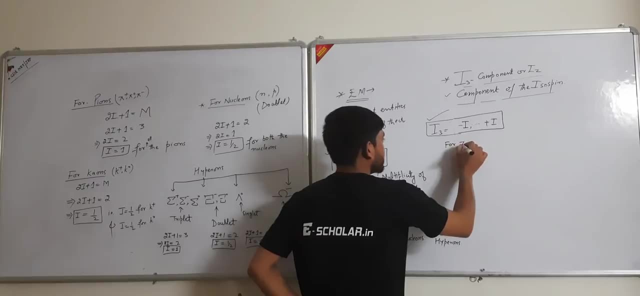 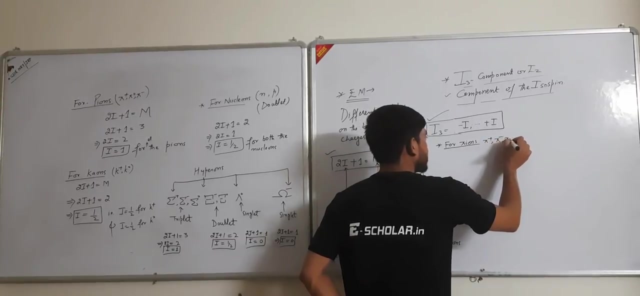 that means value of i is equal to 1. So for pions, for pions, how we can calculate the pions, like pi positive, pi negative and pi zero, the value of i3 is equal to 1. So. 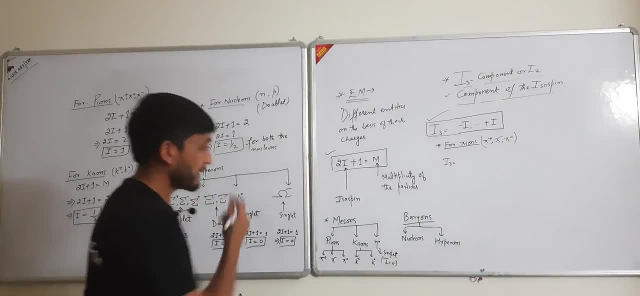 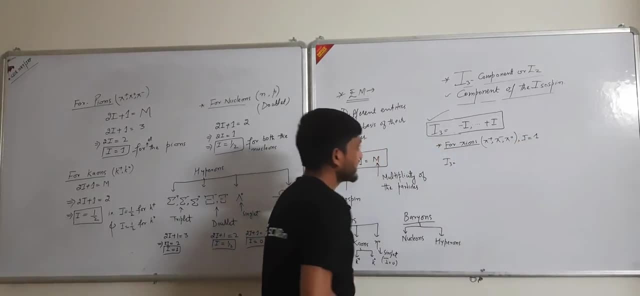 value of i is equal to. here is the value of i: i is equal to 1.. For these pions, value of i is equal to 1 and then value of i3 will become minus 1,. second one is the 0 and third. 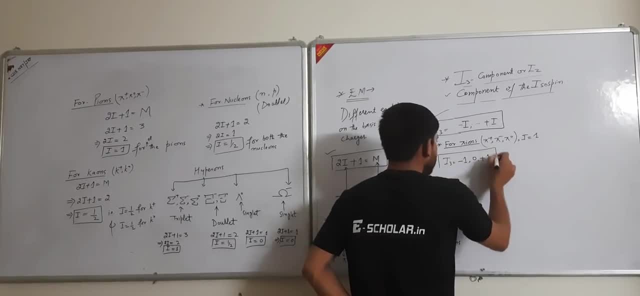 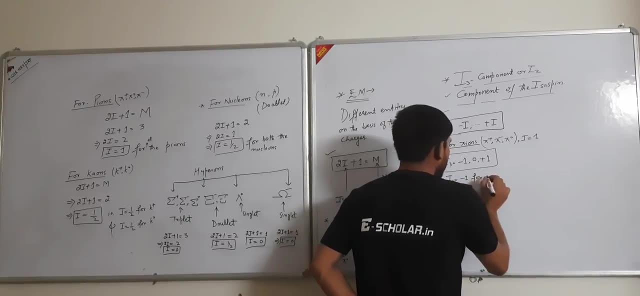 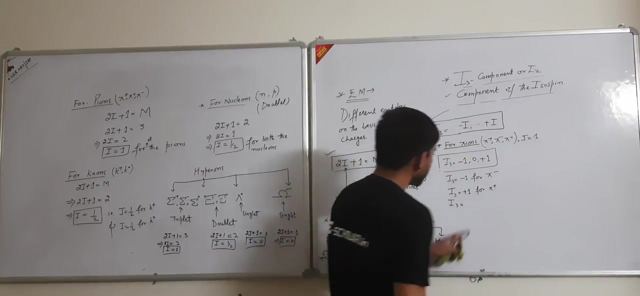 one is the plus 1.. That means value of i3 is equal to minus 1. for which type of pions? minus 1 for pi negative, i3 is equal to plus 1 for pi positive and i3 is equal to 0 for pi 0.. 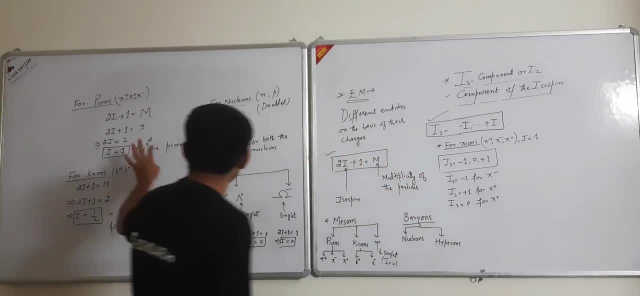 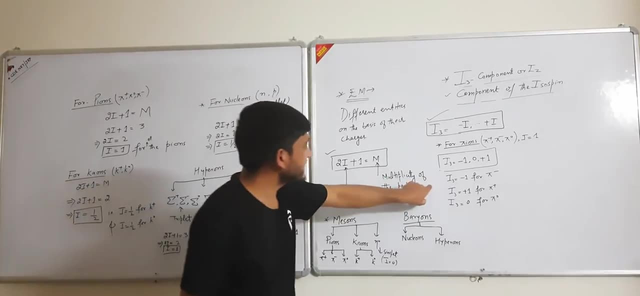 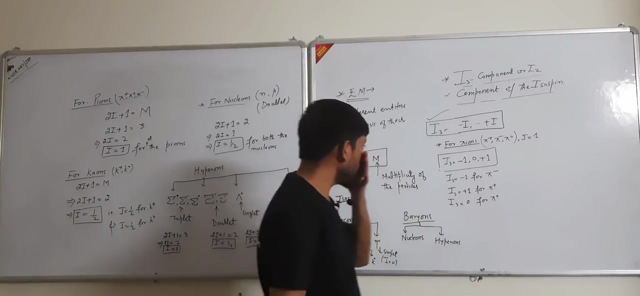 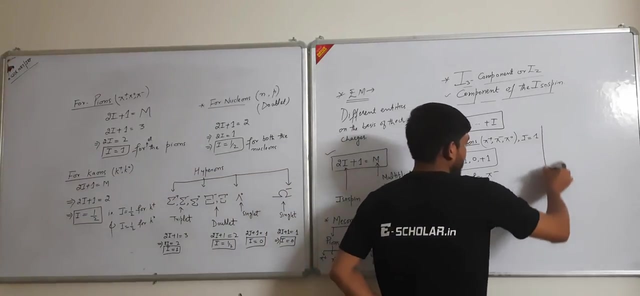 So isospin will remain same for all the these pions, but value of i3 component or iz component will become different for the different elementary particles. ok, So next one is the kions: any kions for kions for kions. 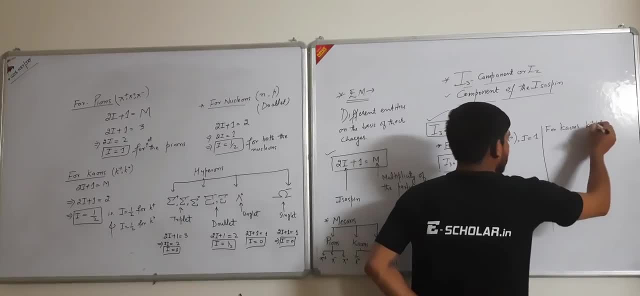 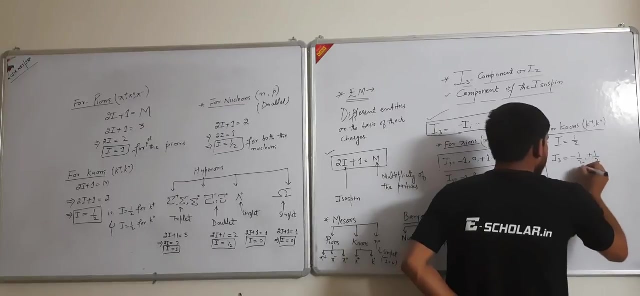 that means k positive. this is a doublet k positive and k0, ok, Isospin for these particles is equal to 1 by 2 and i3 component will become: this is the algebraically addition minus 1 by 2, and the second one is the plus 1 by 2.. 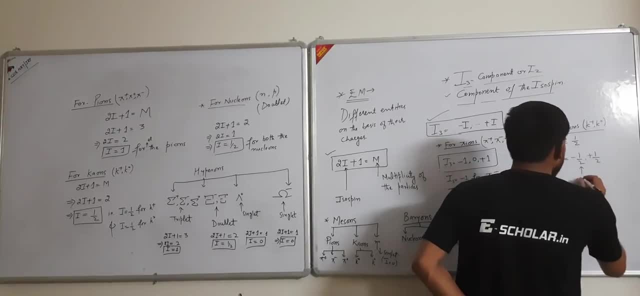 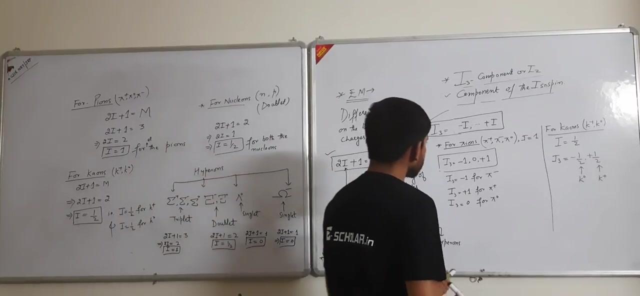 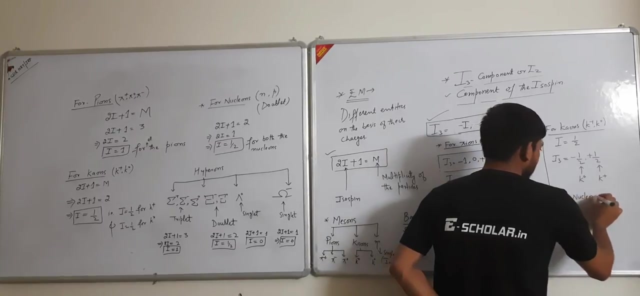 Here: minus 1 by 2. for which type of particles? k0.. and plus 1 by 2 for k positive. ok, now next one is the nucleons. for nucleons, how we can calculate for nucleons? proton and neutron value of I is equal to 1 by 2 and I 3 value. 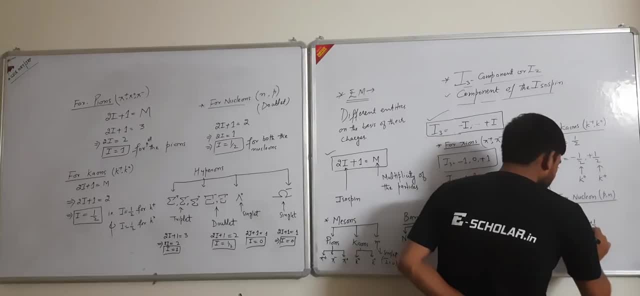 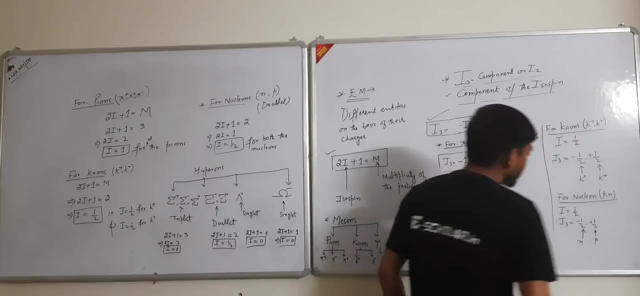 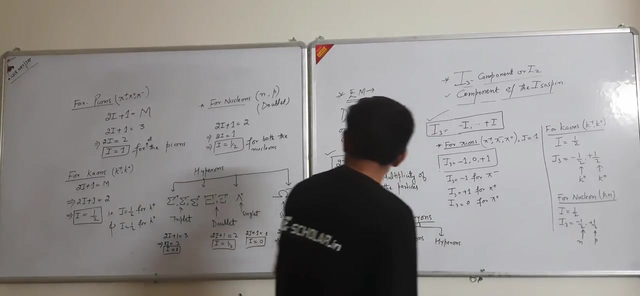 minus 1 by 2 and second one is the plus 1 by 2. that means minus 1 by 2 for neutron and plus 1 by 2 for the proton, And then we will calculate the I3 component for the hyperions. these are the hyperions. 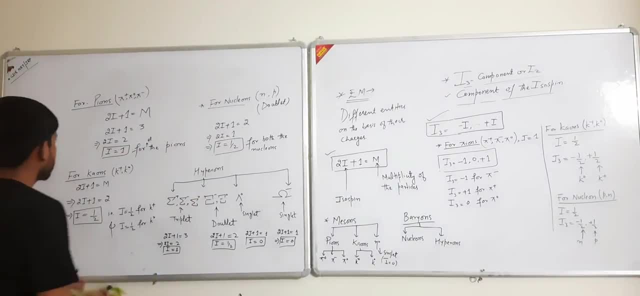 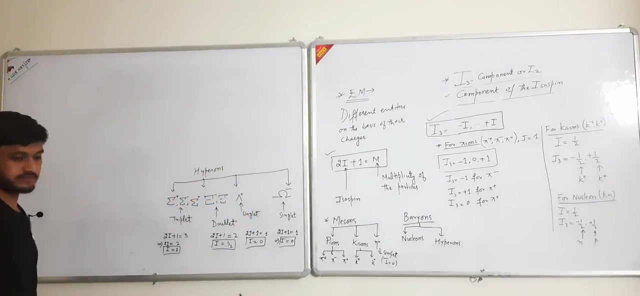 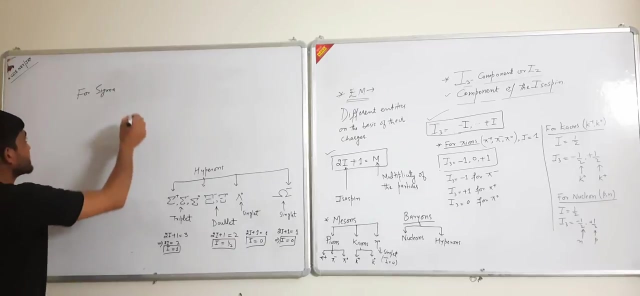 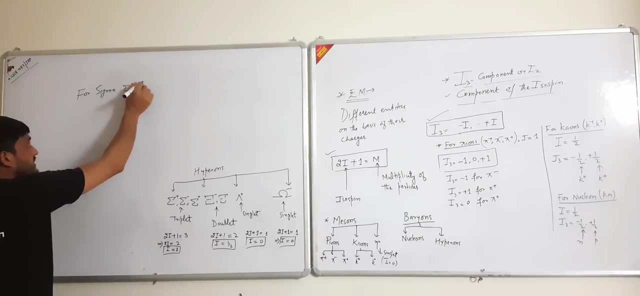 and then let us see how we can calculate: for hyperions, For sigma, for sigma type of the elementary particles. sigma type, this is the triplet: sigma positive, sigma negative, and third one is the sigma 0. ok, and here value of I is equal to 1. this is the isosceles spin, 1.. 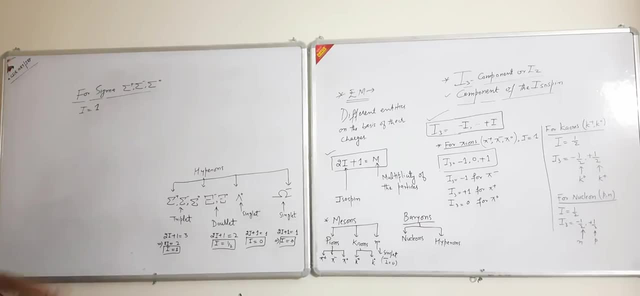 1. Which will remain same for all these particles. ok, and value of I3 will become minus 1. second one is the 0 and third one is the plus 1. it means minus 1 for sigma negative, 0 for sigma 0.. 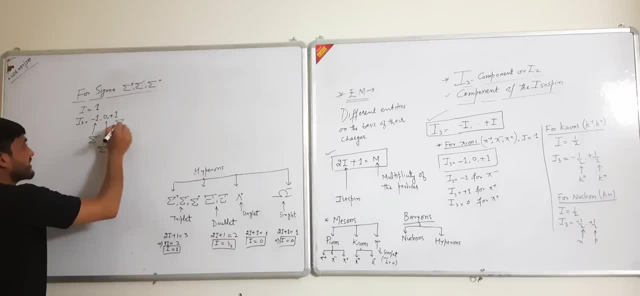 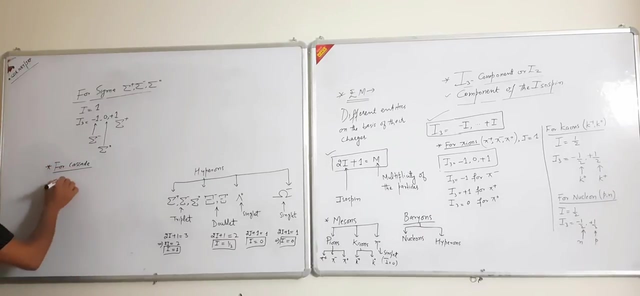 And third one is the plus 1.. And third one is the plus 1 for sigma positive. ok, so this is the I3 component for sigma particles. now then, next one is the cascade for cascade. for cascade, this is the doublet, and value of I is equal to 1 by 2.. 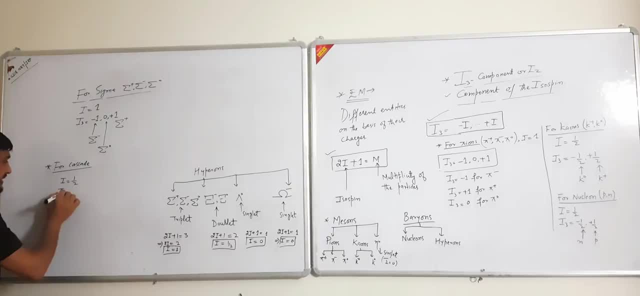 And I3 component And I3 component And I3 component, I3 component- Minus 1 by 2 and second one is the plus 1 by 2. so this one for the cascade negative and this one for the cascade 0. ok, now, next one is the next one is the lambda for lambda. 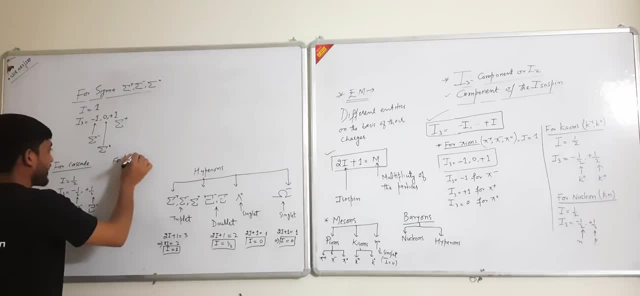 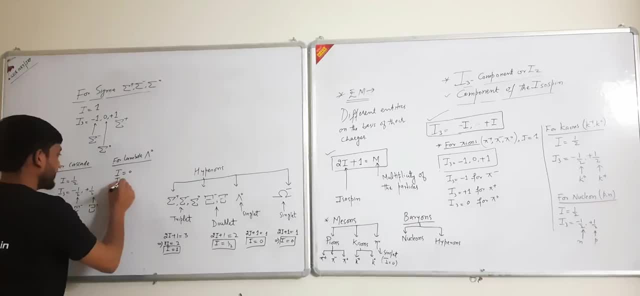 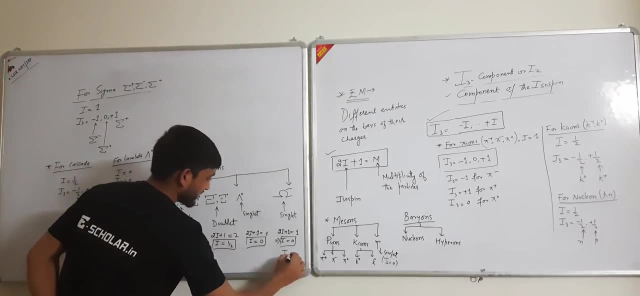 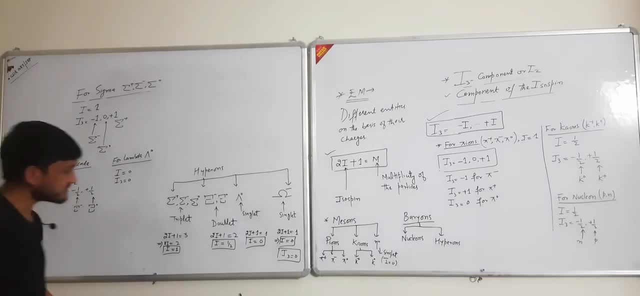 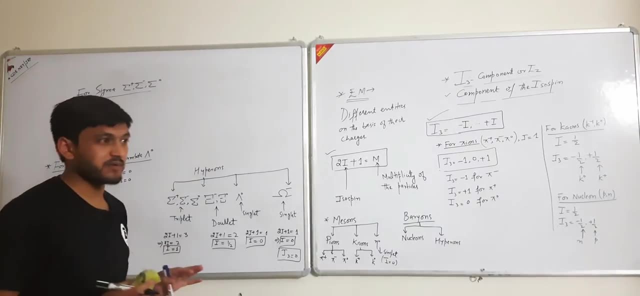 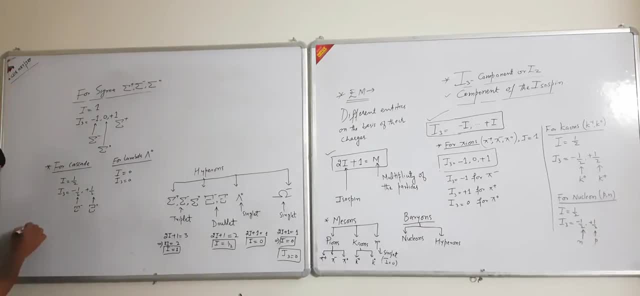 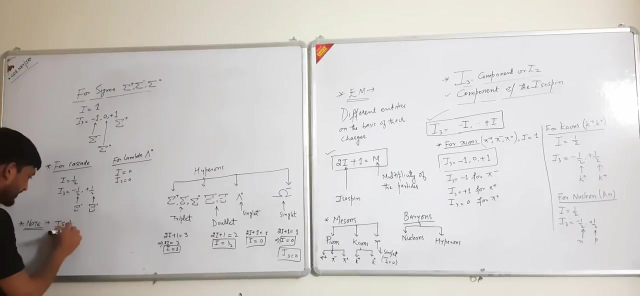 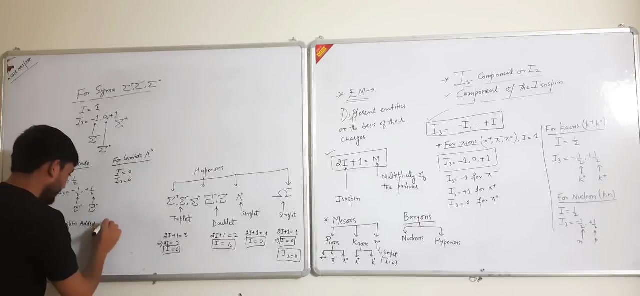 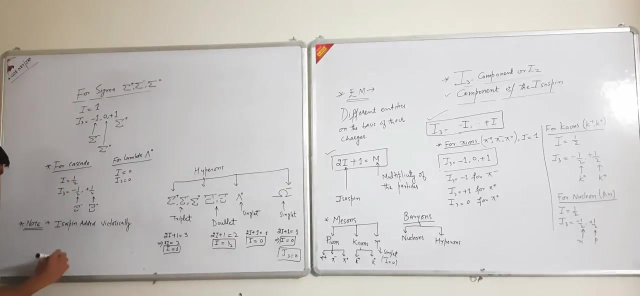 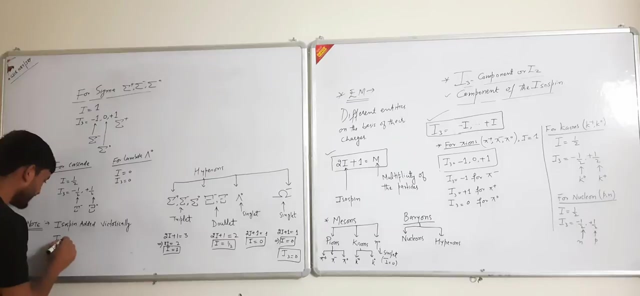 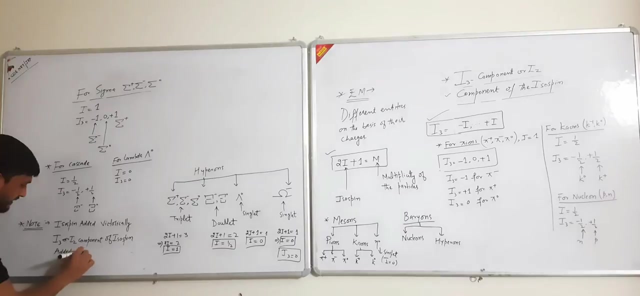 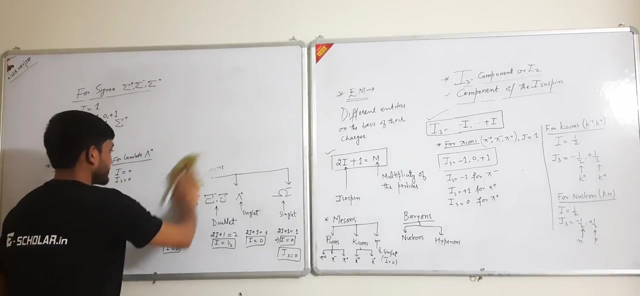 And I3 component And I3 component. note: isospin added vectorically and I3 that means I3 component will be added or Iz component, component of isospin Will be added algebraically added. algebraically added- algebraically. ok, so next is the new thing. 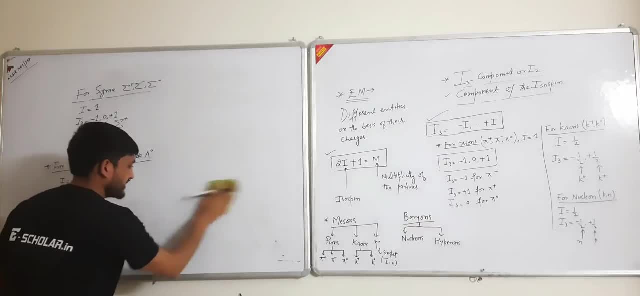 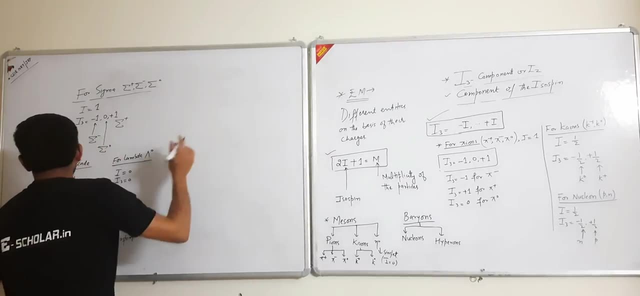 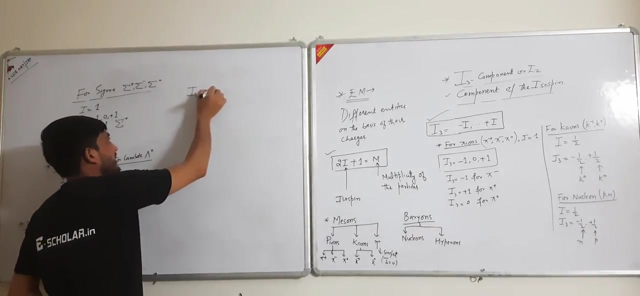 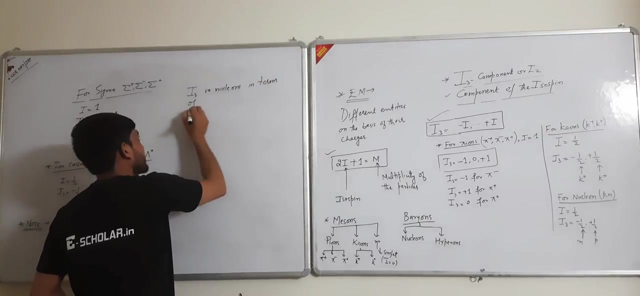 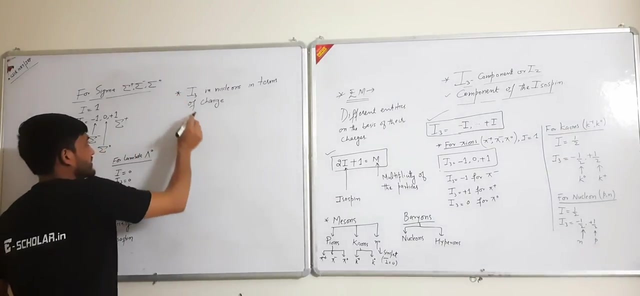 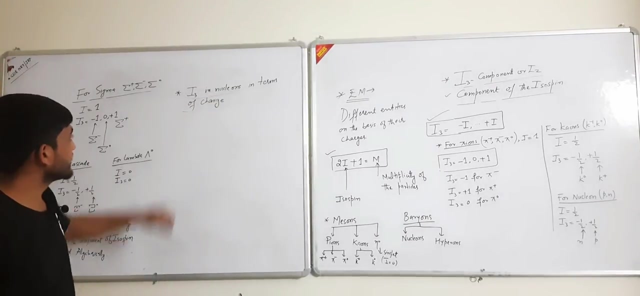 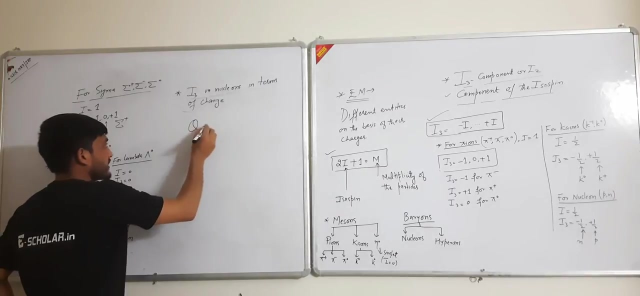 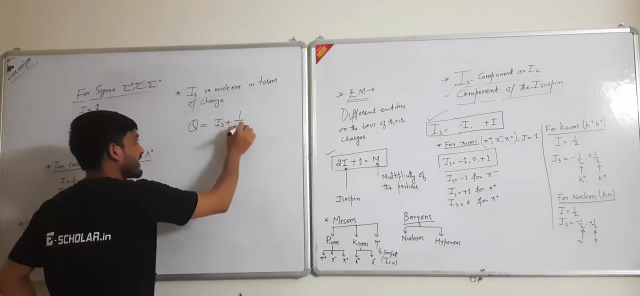 I3 in terms of charge for the nucleons. ok, here new thing are also introduced here: I3 in nucleons in terms of charge. In terms of charge and how we can calculate the charge from the I3 component of this nucleons. ok, so here is the formula: q is the charge is equal to I3 plus 1 by 2.. 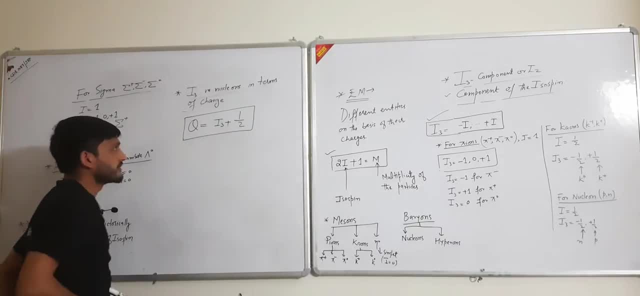 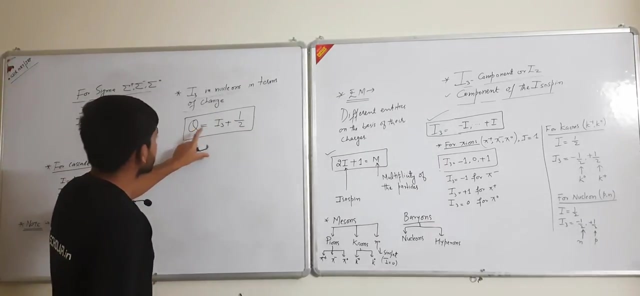 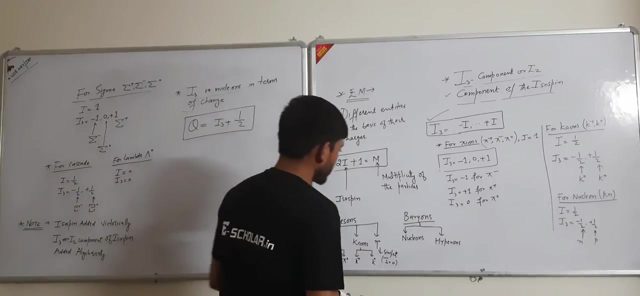 By the using of this formula we can calculate the charge of the different particles. here is the nucleons. now how we can calculate the charge of nucleons. ok, so nucleons is the doublet. so first of all, check the I3 component. where is the nucleons? that means for the nucleons. 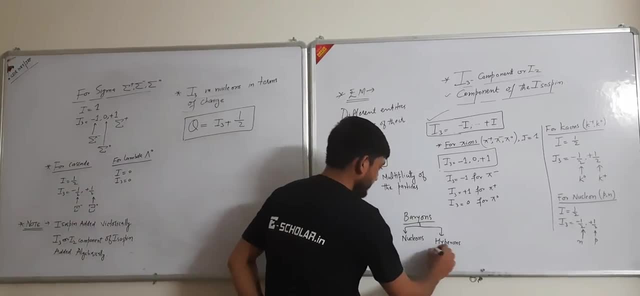 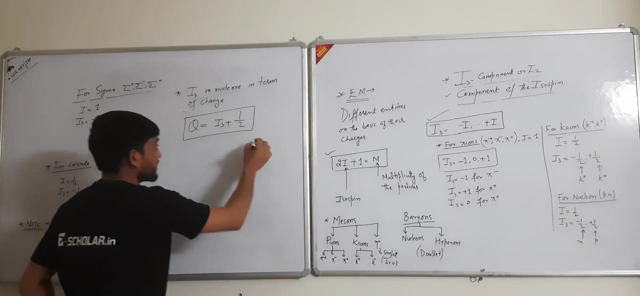 this is the doublet. Let us check for theаствores Classic. Now try to calculate 실 in I2 angle by using the inversions factor, which is good. social write says that I3, Adventure 3, and the intersection of the resultant is equal to. 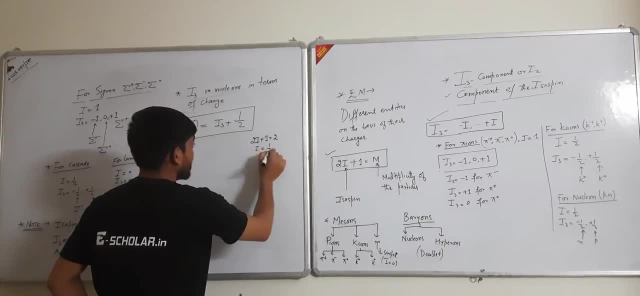 this angle, Then I of and right becomes Ií at valley, and then the intersection is equal to And isospin ile will become 2. I plus 1 is equal to 2. i is equal to 1 by 2. that means: 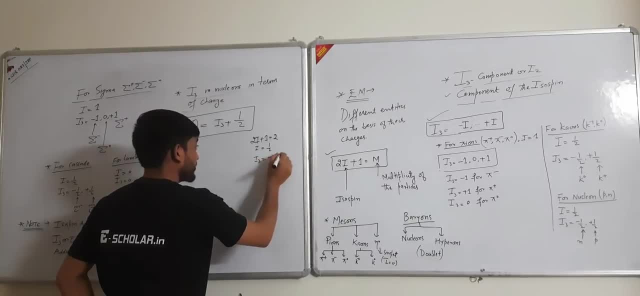 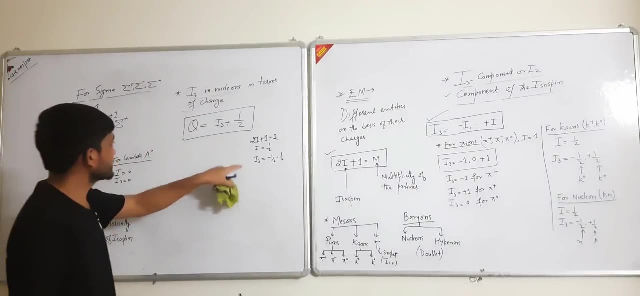 I3 minus 1 by 2 and plus 1 by 2, minus 1 by 2 for the neutrons and 1 by 2 for the proton. so here is the For. let us see for neutrons and customer two: frick demonry. 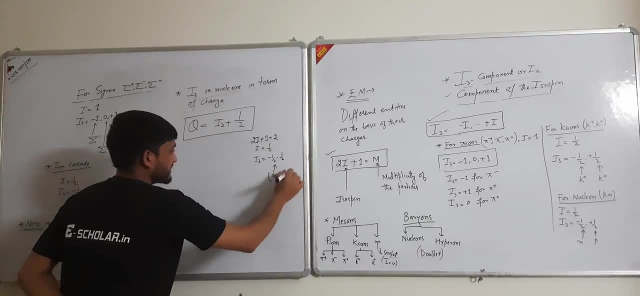 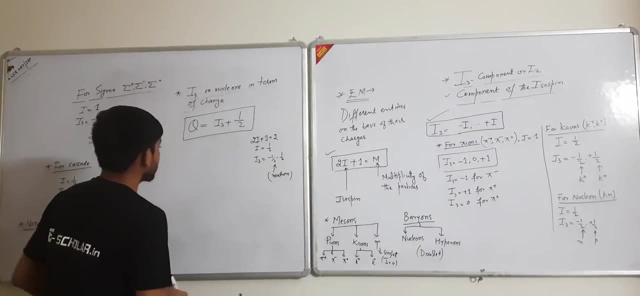 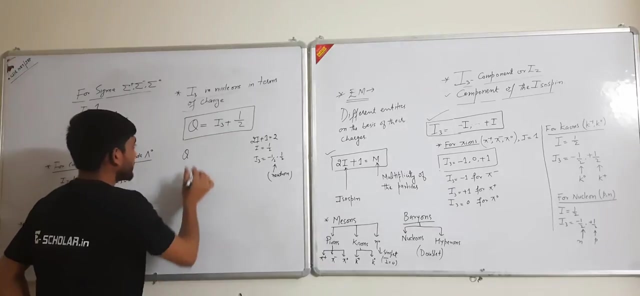 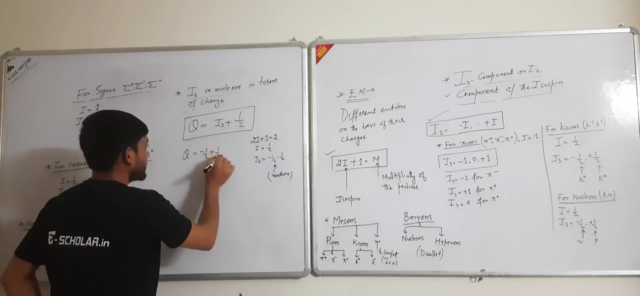 I will take the first: Newton, then charge of the Newton. which type of the charge of Newton we can calculate by using this formula: I3 for Newton is equal to minus 1 by 2, and this is the 1 by 2 according to formula. so here is the value of Q is equal to 0 for neutrons. 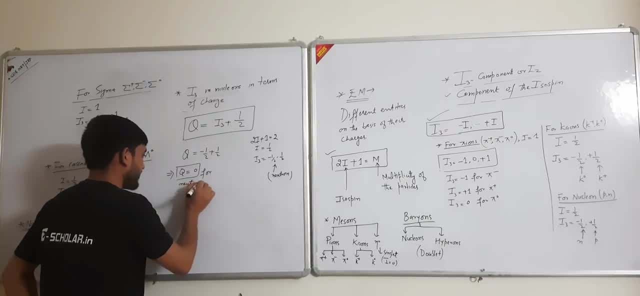 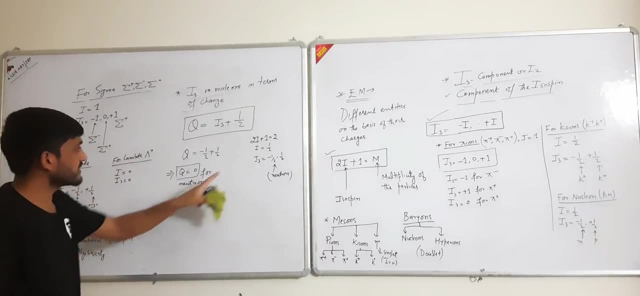 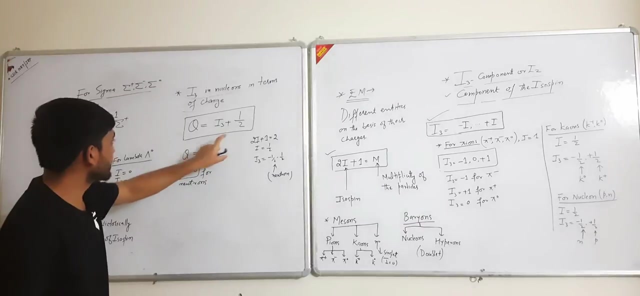 okay, this is the formula for the nucleons. now next formula and same method for the proton. here value of I3 is equal to 1 by 2, and then 1 by 2 plus 1 by 2 is equal to 1, then charge. 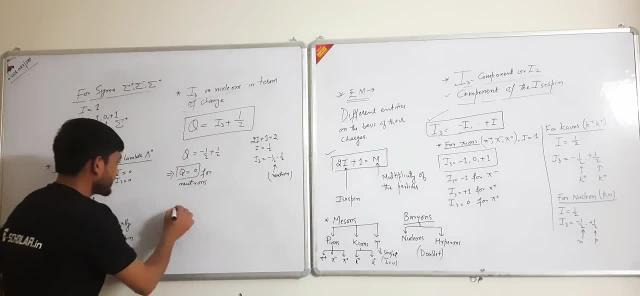 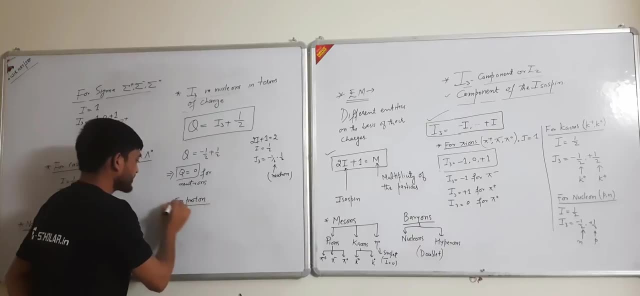 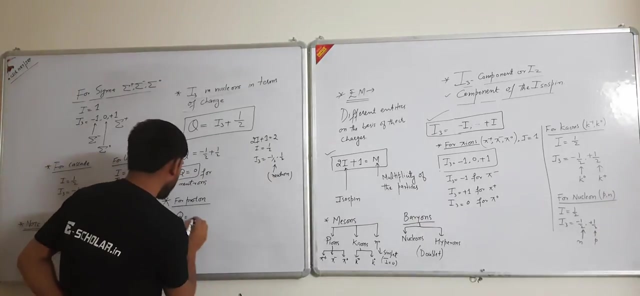 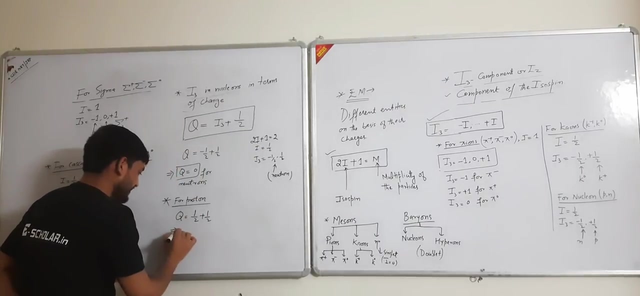 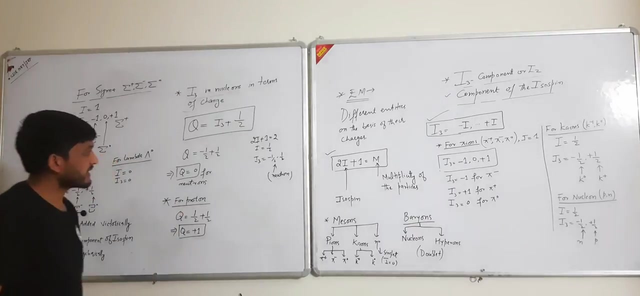 of the proton will become for proton. how we can calculate the charge? Q is equal to I3, I3, 1 by 2 plus 1 by 2 according to formula. then charge of the proton is equal to plus 1 according to this formula. 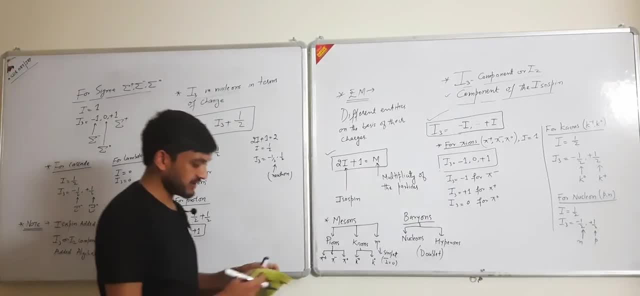 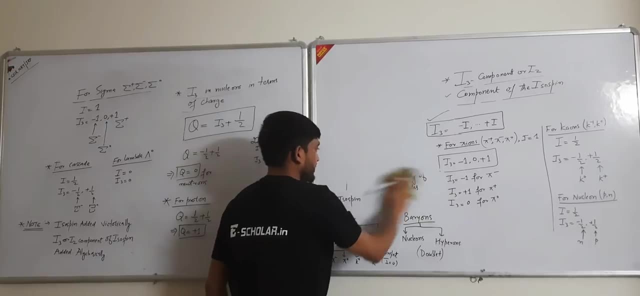 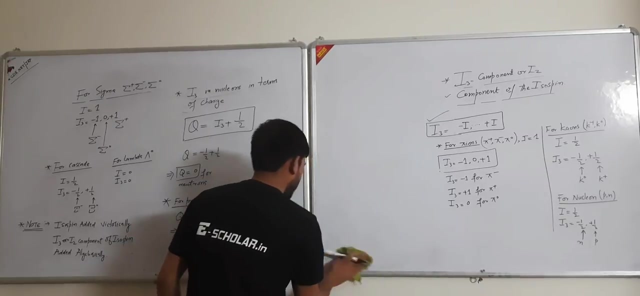 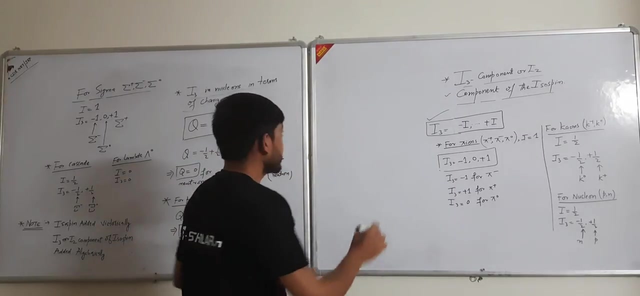 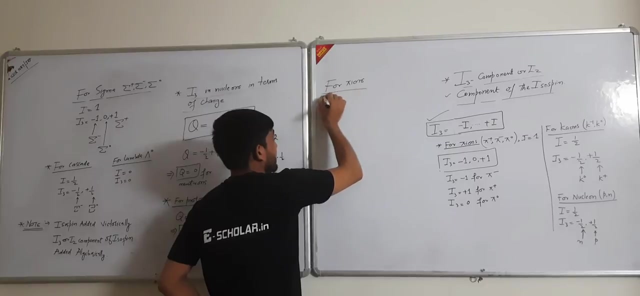 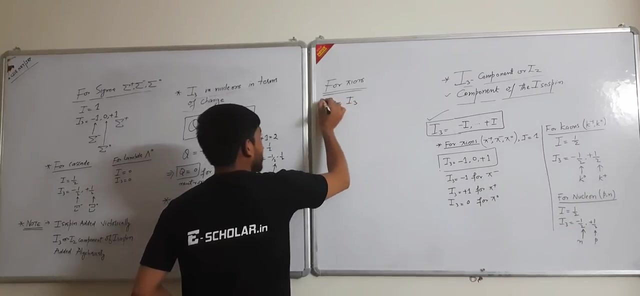 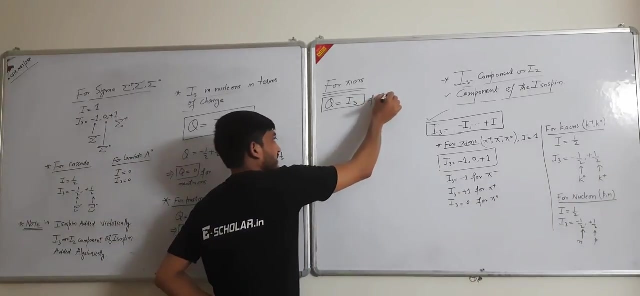 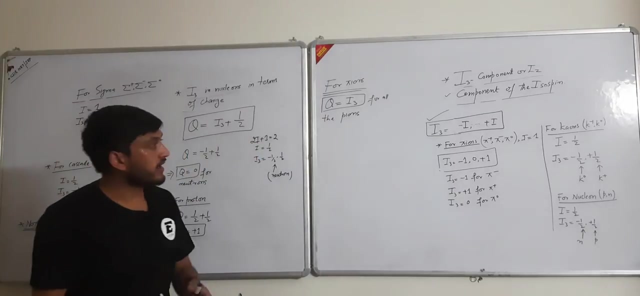 and for the pions. for pions, how we can, we can calculate the charge. now see here. for pions, another formula: q is equal to i3, which is applicable for all the pions, for all the pions, for all the pions. Now see here. 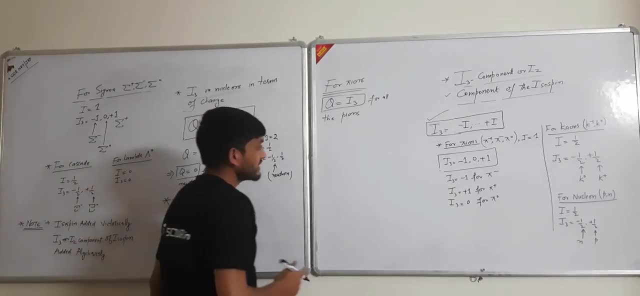 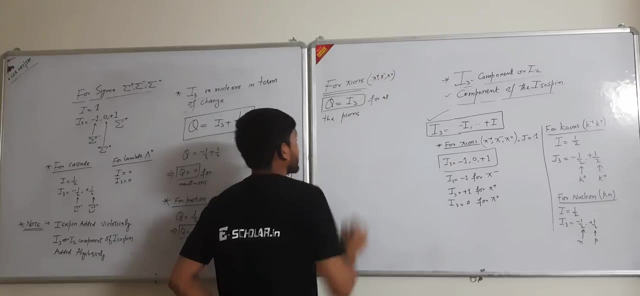 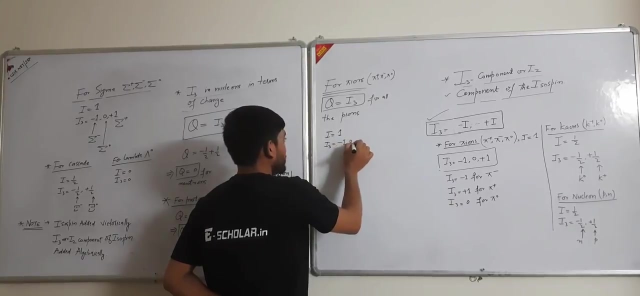 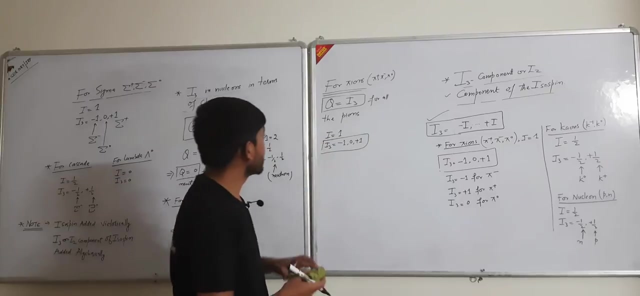 How we can the charge. So first of all pions. this is the triplet and value of isospen will become 1 and I3 will become minus 1, 0, plus 1. for all these pions that means for pi negative. 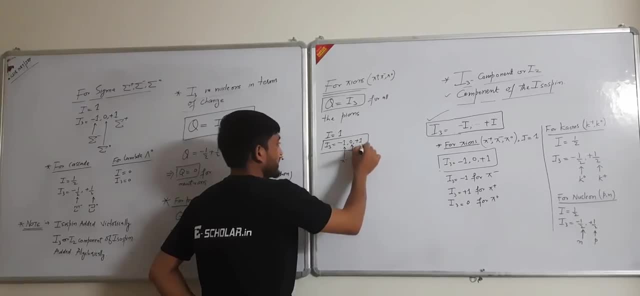 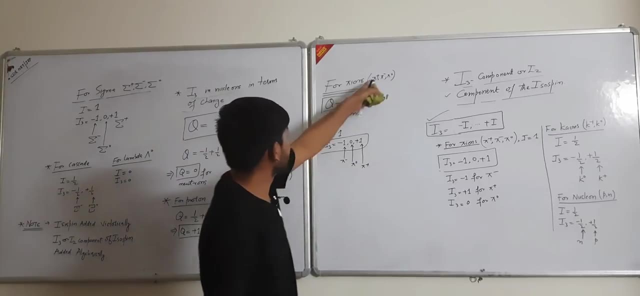 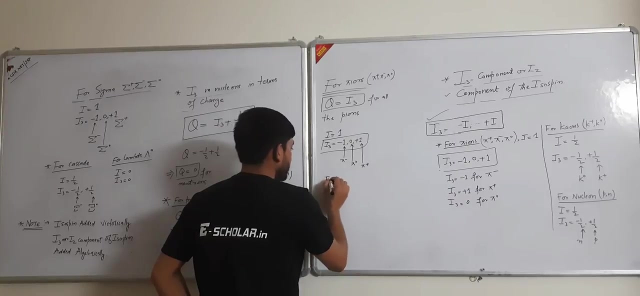 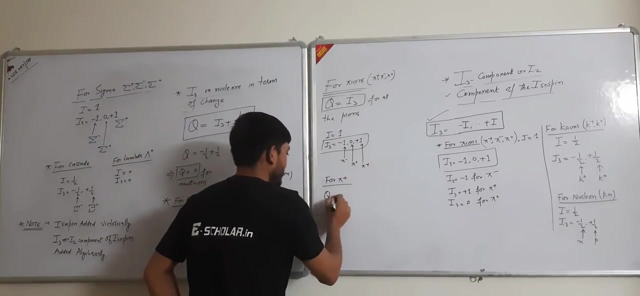 0 for pi 0. and third, one is the plus 1 for pi positive. Now calculate the charge So of the pi positive, this type of pions, here for pi positive. we will calculate the charge of pi positive. u is equal to I3, here I3, value of I3 for the pi positive plus 1, and same. 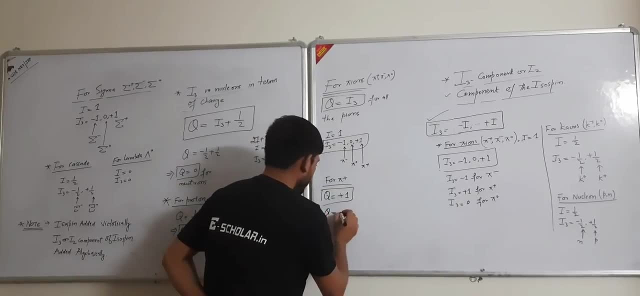 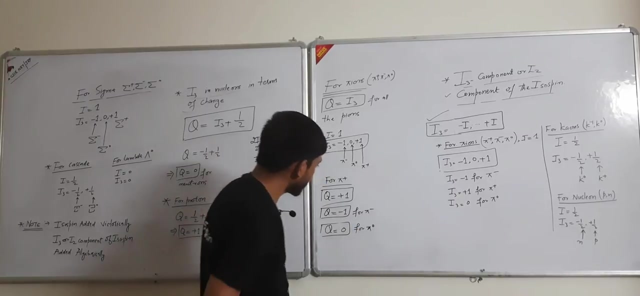 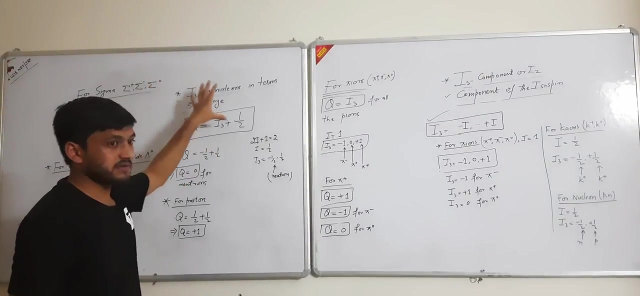 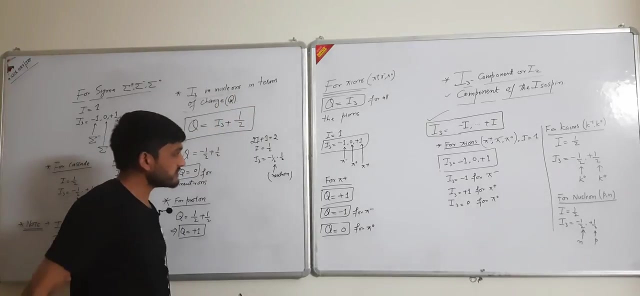 we can calculate for minus 1.. Ok, for pi negative and value of charge is equal to 0 for pi 0. so this is the method how we can calculate the charge in terms of i3. okay, this is the charge killed, and then next one. here is the: 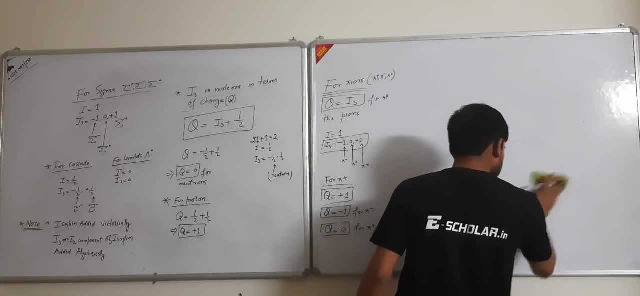 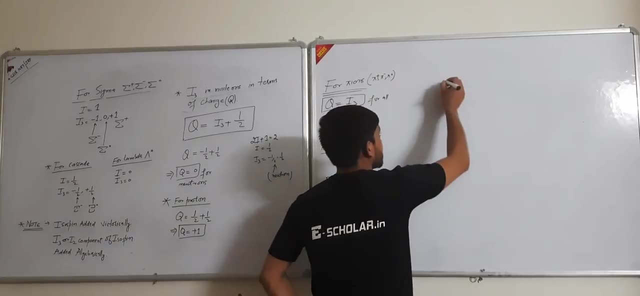 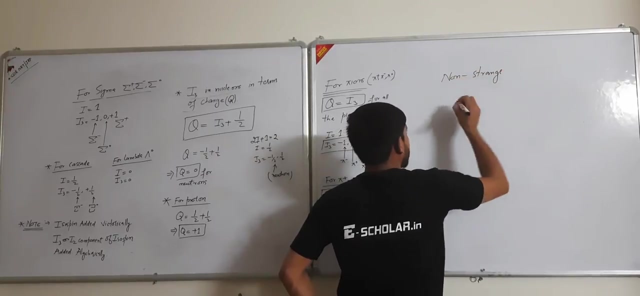 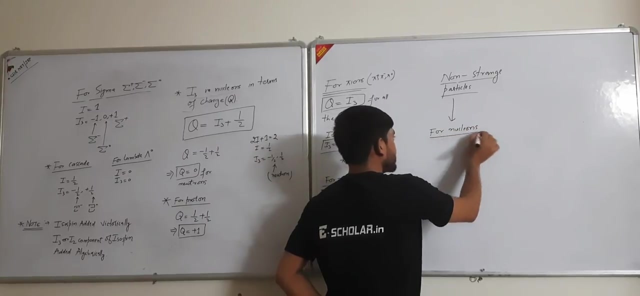 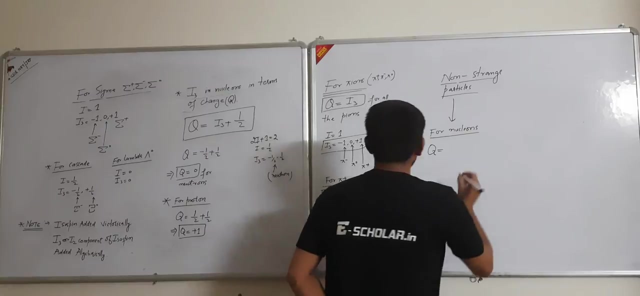 now pions and the. these nucleons are which type of the particles these particles are? the non-strange particles, non-strange particles. okay, here is another formula which is applicable for nucleons: for nucleons. for nucleons, values of charge will be calculated plus b12. this is the b, and here b is the nothing but a barrier number. 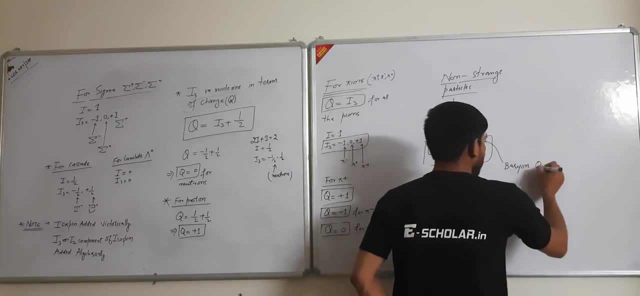 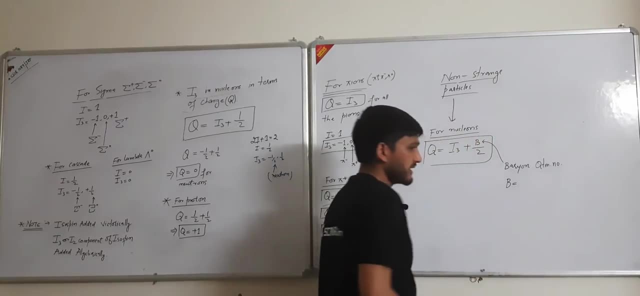 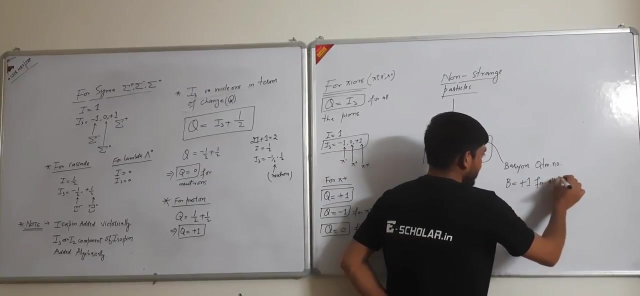 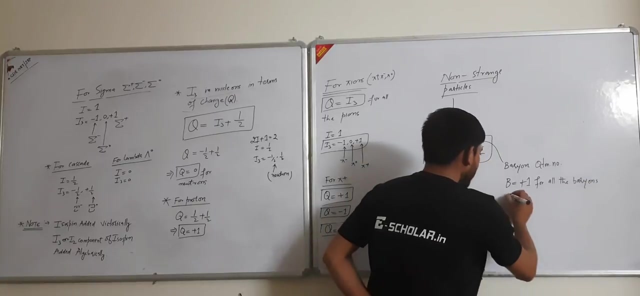 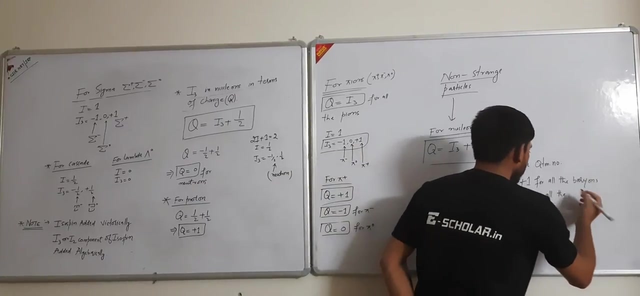 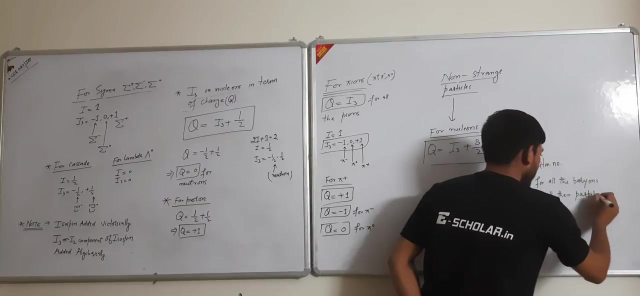 variant quantum number. okay, and the value of b will remain positive, one for all the variants, and value of b barrier number is equal to zero for all the other particles. that means means another particles which are not baryons, for all the for all other particles. okay now. 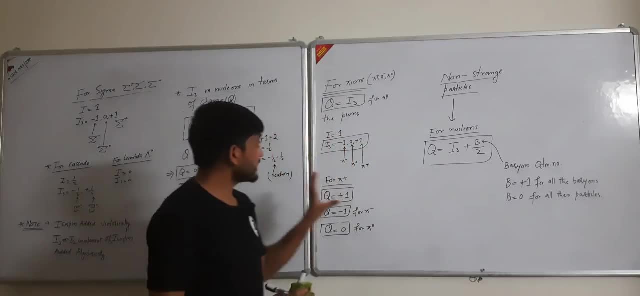 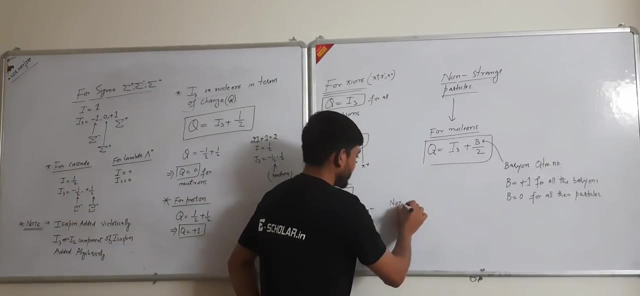 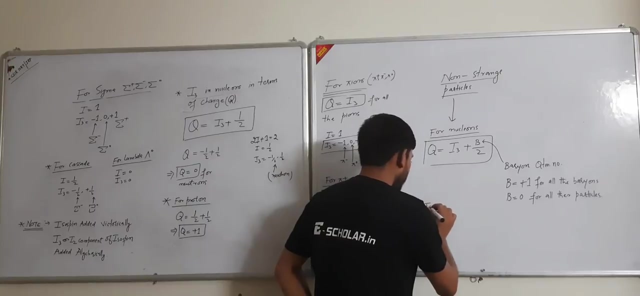 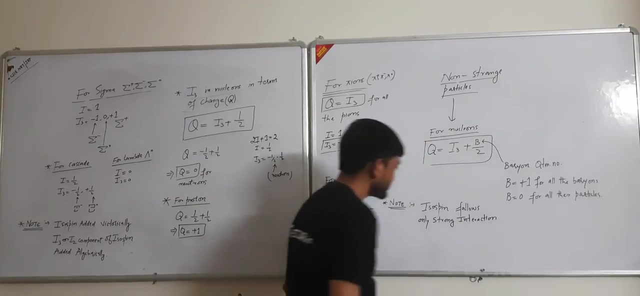 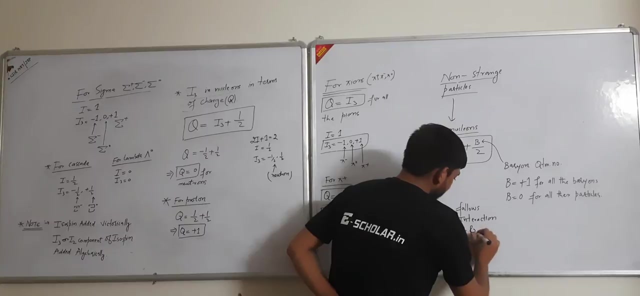 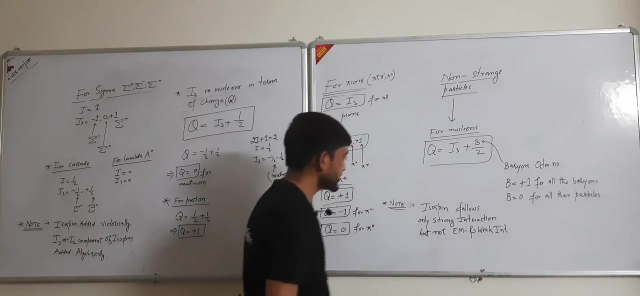 next one, these isospin and i3 component. note, note one thing here. first of all, isospin, isospin follow. which type of interaction follows? only strong interaction. strong interaction, interaction, but not electromagnetic and weak interaction. okay, this is the isospin and i3 component. this is the first one and second one is: 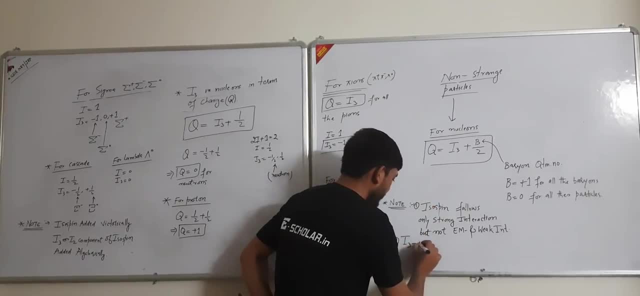 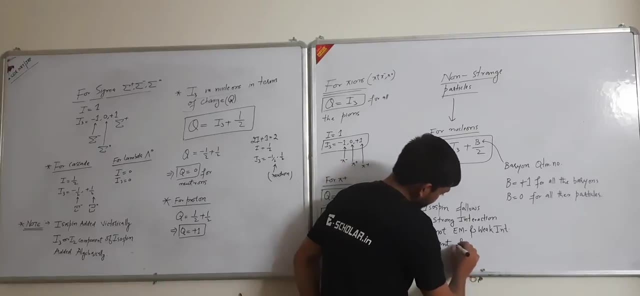 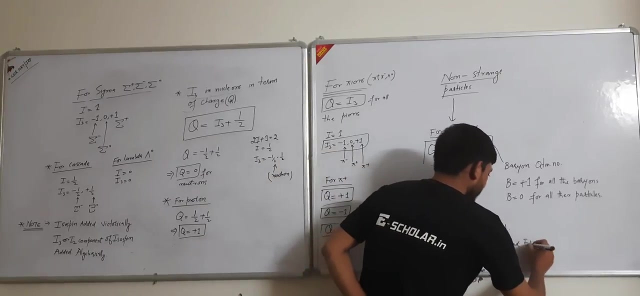 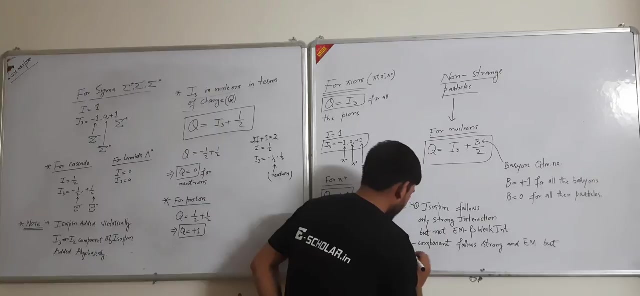 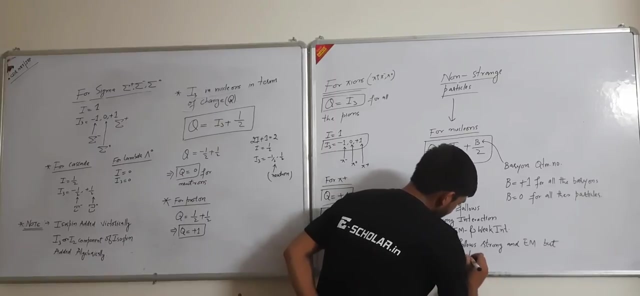 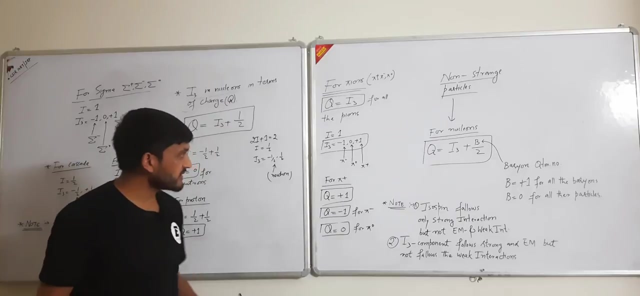 the i3 component. i3 component follows strong, follows strong and electromagnetic, but not follows the big interaction, the big interaction, big interactions. okay, so this is the method: how we can, we can calculate the value of isospin and the third component of the isospin for all. 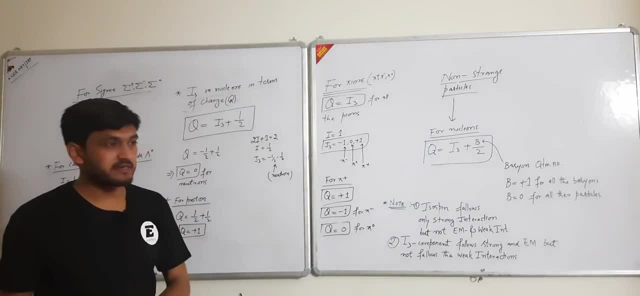 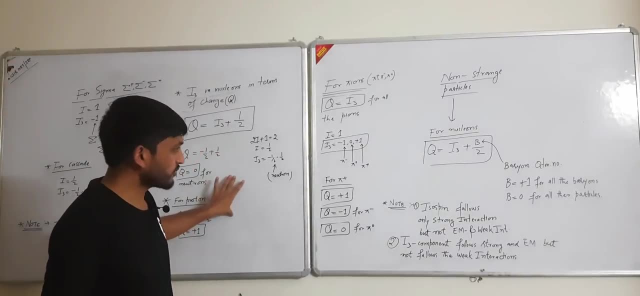 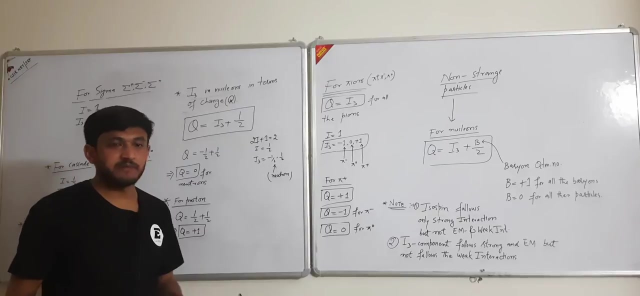 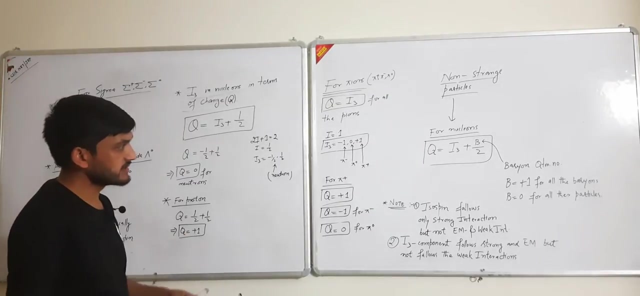 the elementary particles, like mesons and the baryons, and in the baryons will divided into two different categories. first one is the nucleons and then hypoions. and hypoions are also divided into four different categories, like lambda, sigma and etc. now next one is the strangeness: how we can calculate the strangeness of all these particles? and which type of particles are strange particles? ok now, concept of strange particles. now let us see here how we can calculate the strangeness of the particles. all the strange particles are generally formed in a pair, not formed in a single form. we know that, hypoions and kaons. first one is the strangeness. how we can calculate the strangeness. 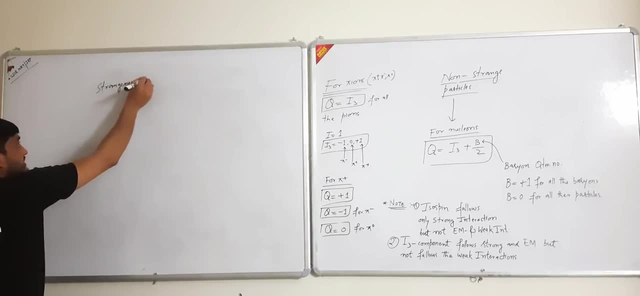 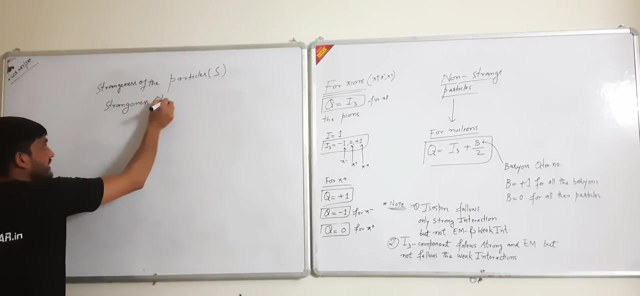 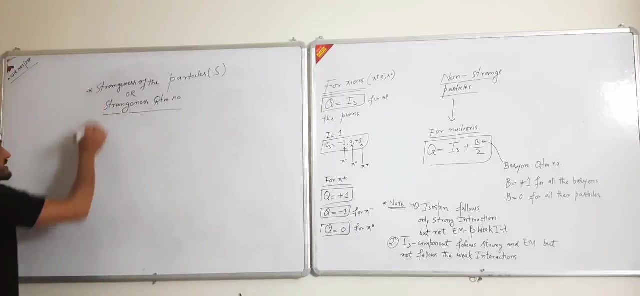 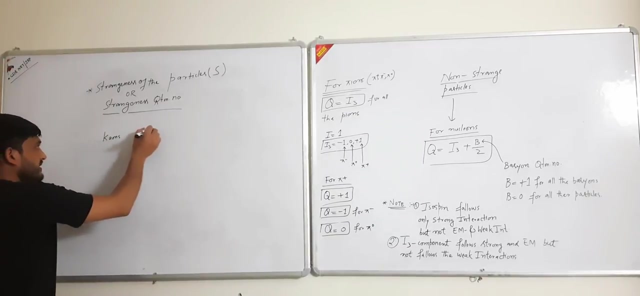 of the particles S. or we can say that this is the strangeness counter number: ok, 她, and so on, etc. we can calculate this. first of all, what is a strangeness? okay, we know that Chian's, and second one is the Hyperion's. both are strange particles. which type of particles are strange particles? and these are not decaying in a single form but a decay into in the form of pairs, and they are also called as the associated particles. which type of particles? associated type of particles? because they are not singly produced. associated type of particles. associated type of particles. type of particles, associated type of particles are divided into two forms. first one is the Chian's and second one is the Hyperion's. okay, these particles are generally. when the formations of these particles, then strong interactions are occur and when they are decaying, they will decay into. 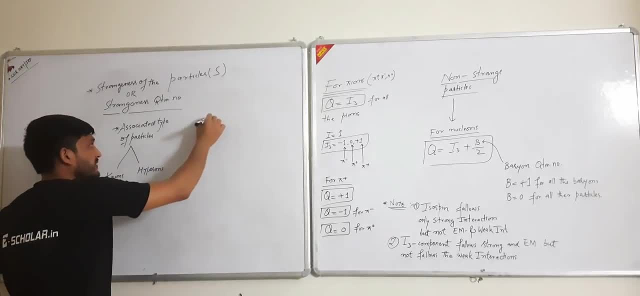 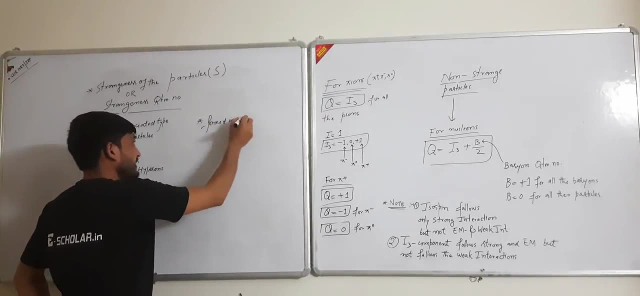 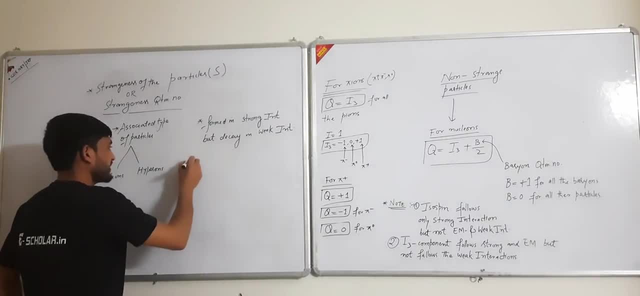 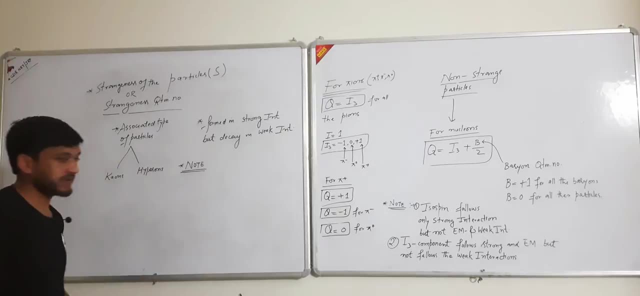 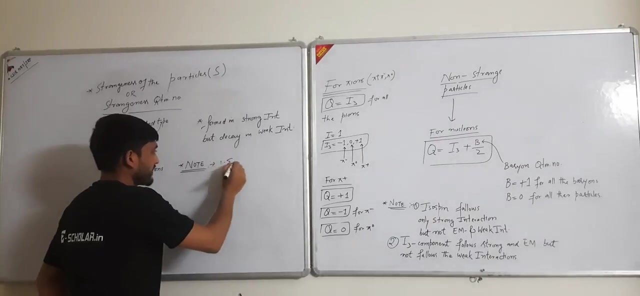 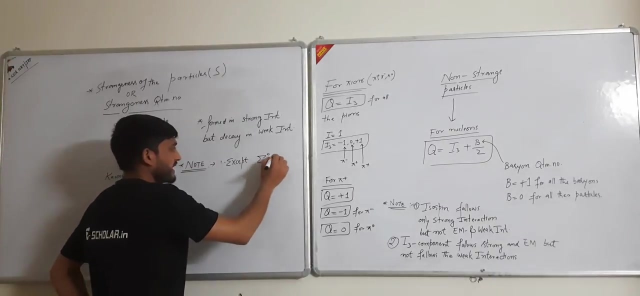 Chian's and second one is the Hyperion's. okay, these are the Chian's and second one is the. So note here one particle belonging to the family of hyperions, except sigma 0, which will decay into, which will decay in the electromagnetic interactions. okay, Electromagnetic interactions. 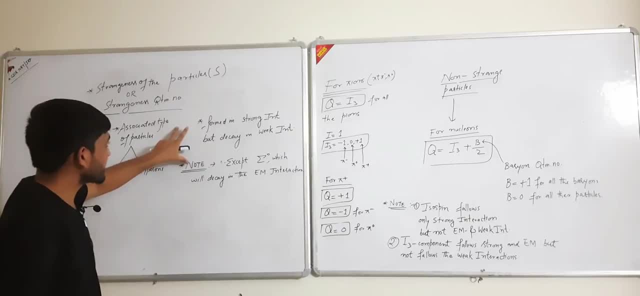 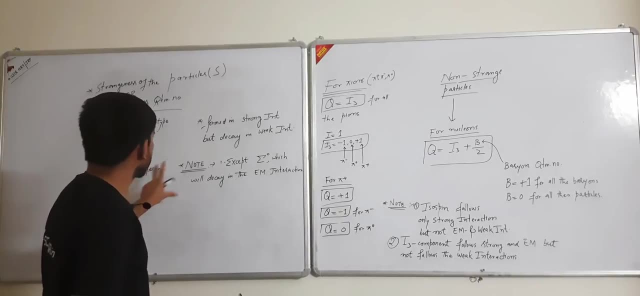 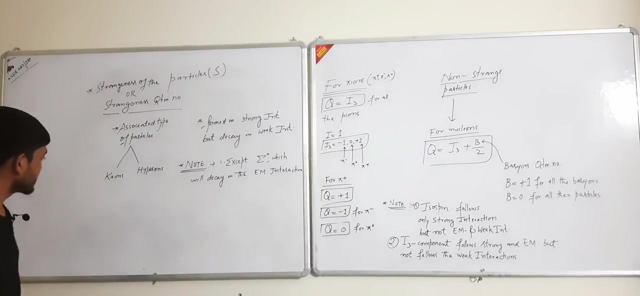 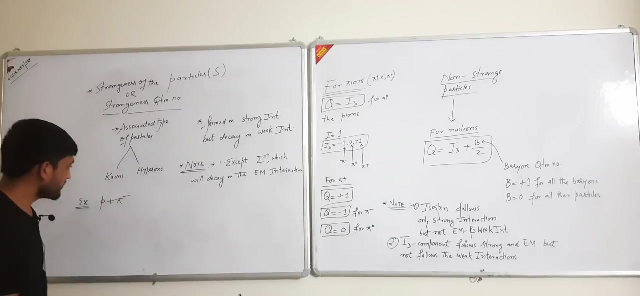 except sigma 0, all the strange particles, just like the kaons and the hyperions. Hyperions are produced in the formation of strong interactions but decay in a weak interactions. Now let us see example Example here. first one is the proton and second one is the pi negative. 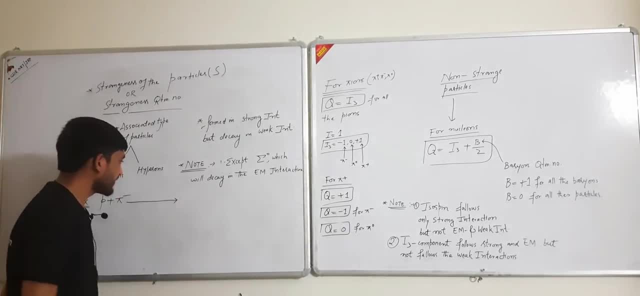 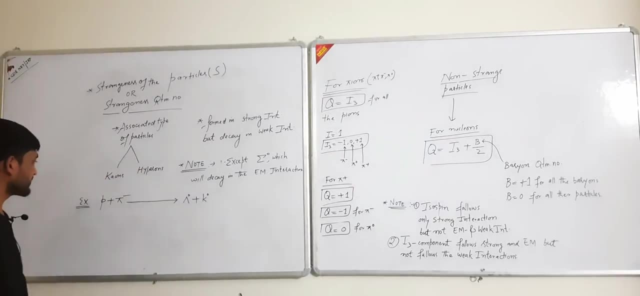 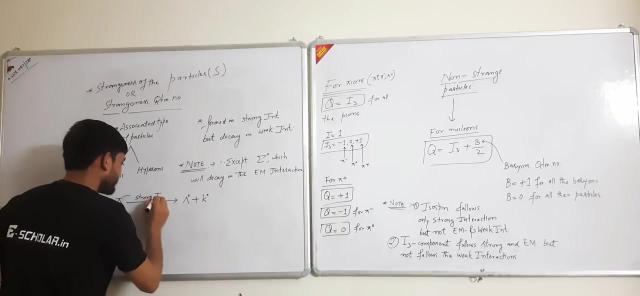 will decay into lambda 0.. Okay, Plus k0 formations of these. this is the strong interactions. which type of interactions occur here? strong interaction? okay, And when these, both the particles in the right hand side are decay into, just like this, particles decay into, which type of particles decay into k0. 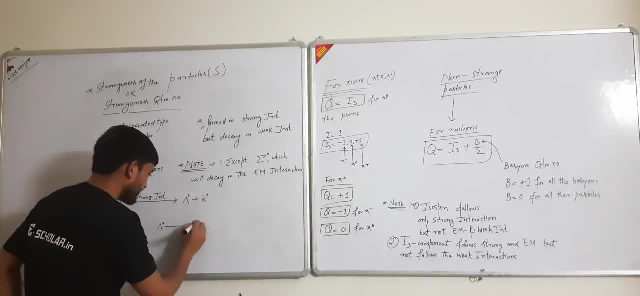 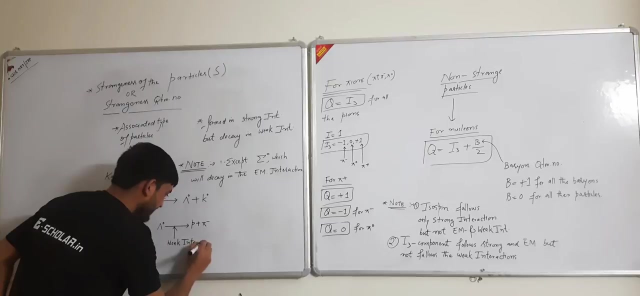 Okay, Okay, Okay, Okay, Okay, Okay, Okay. This is the weak interaction. which type of interactions are occur here? weak interaction, weak interaction. and second one is the k0, or also decay into pi positive plus k0.. Okay, Okay. 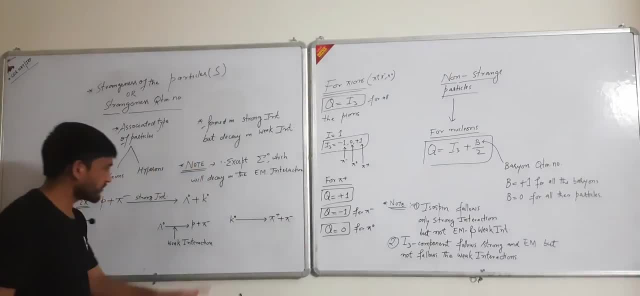 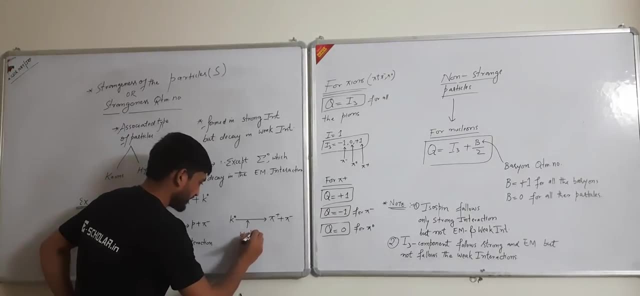 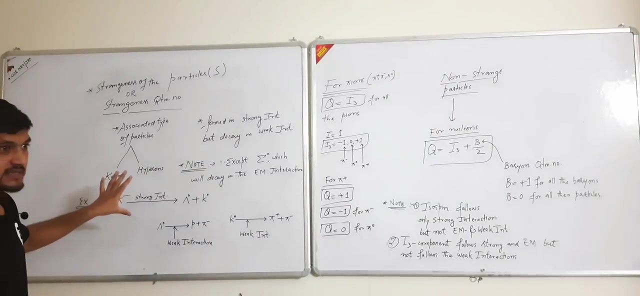 Okay, It will be interact to be equal to pi negative. this is also big contraction. big type of interactions are occur here, big contraction. so this are the 5 positive and the. so these are the strange particles. now we can easily understand which type of the particles are strange particles. 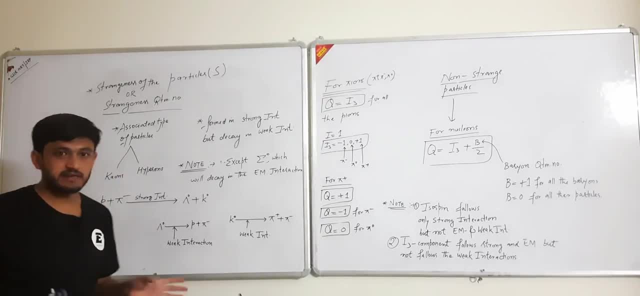 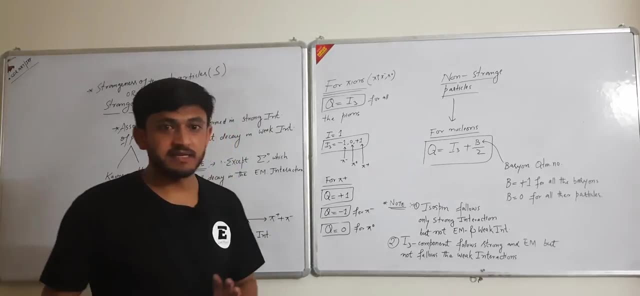 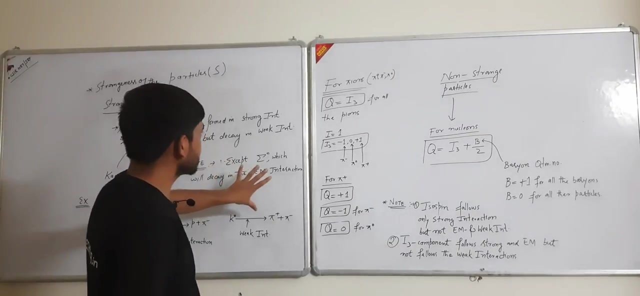 those particles which are formed in a strong type of interactions but decay in the weak interactions, Okay, interactions, and these all the particles are called the strange particles, and how we can calculate the strange or strangeness number of all the strange particles? now let us see here. 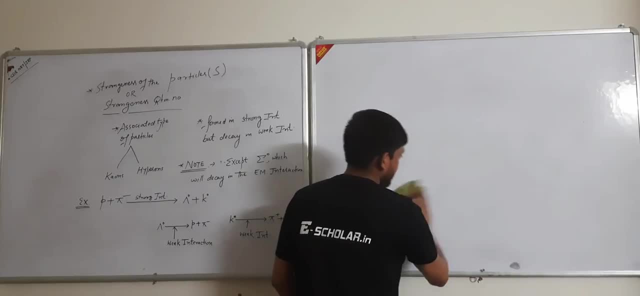 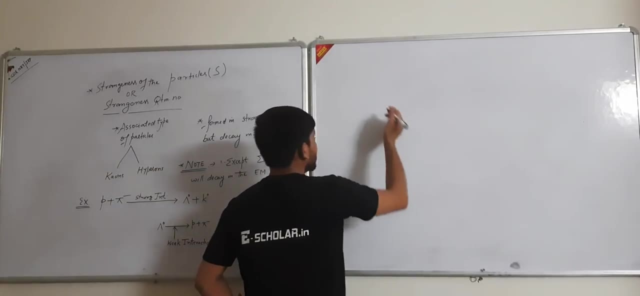 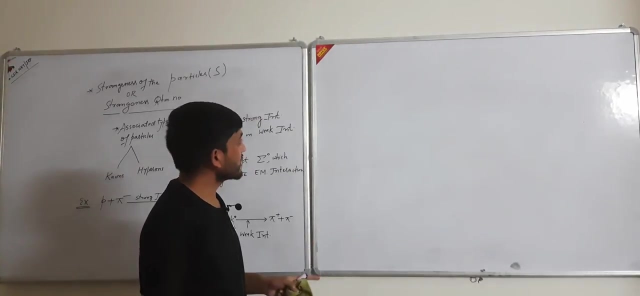 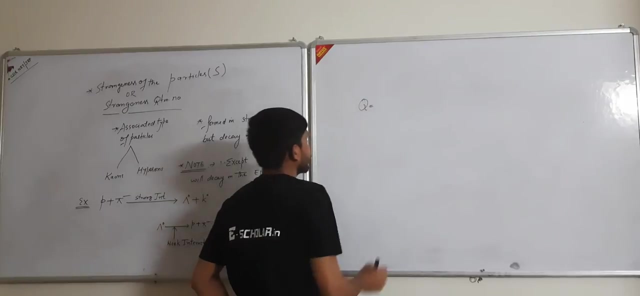 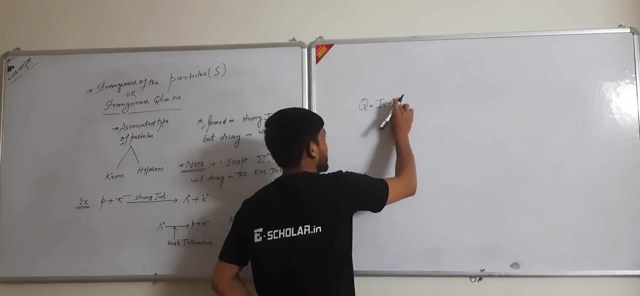 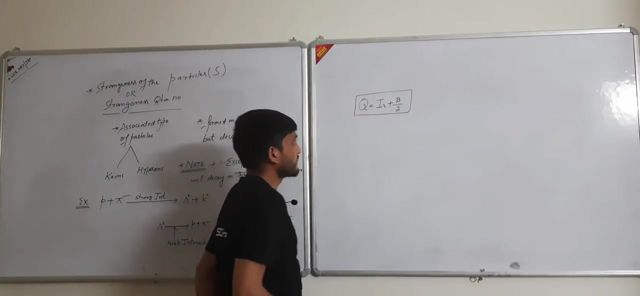 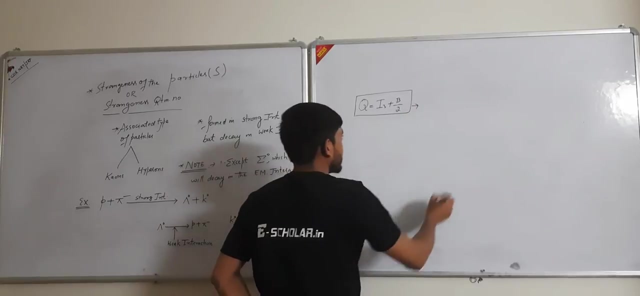 when we calculate the charge in terms of i3 component, then new type of formula will introduce for the non-strange particles, like this formula we are already discussed now: i3 plus B upon S, sorry, B upon 2. okay, this formula are already discussed. when we calculate i3 in terms of charge or charge. 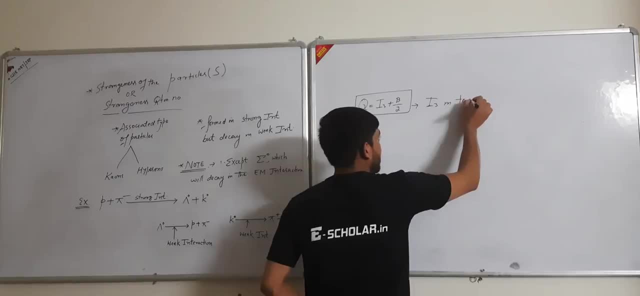 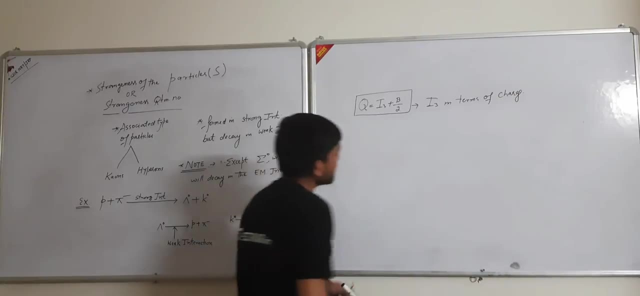 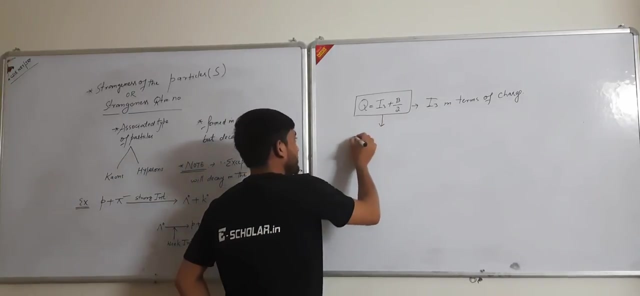 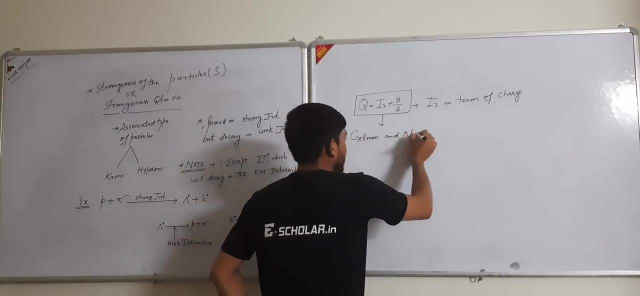 in terms of i3. i3 in terms of charge in terms of charge. okay, in terms of i3 in terms of charge. so the difference which must be organized, k or surface distance lead, comes from this, for the strangeness of this catching. okay, this is the left hand side. same thing, this is right. 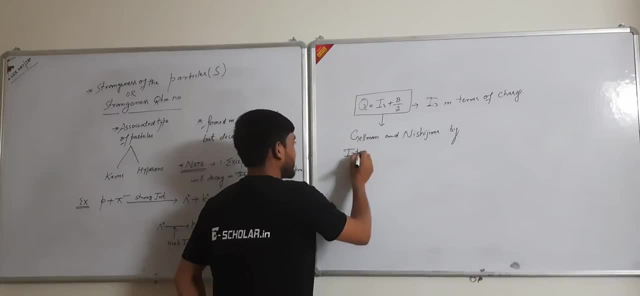 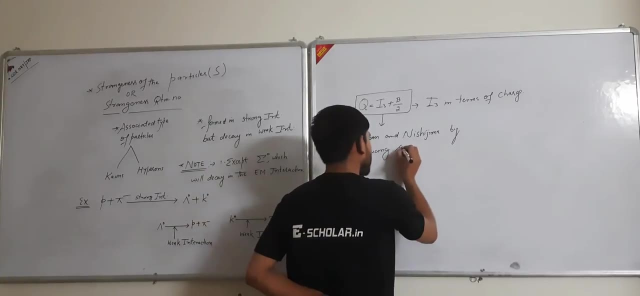 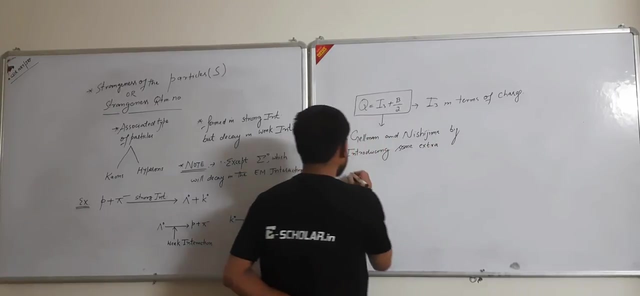 this is left hand side and this formula is generally modified by the Geleman and Nishiyama Nishiyama by introducing so b plus E, So some extra terms. extra terms in the in this formula. extra terms in this formula. 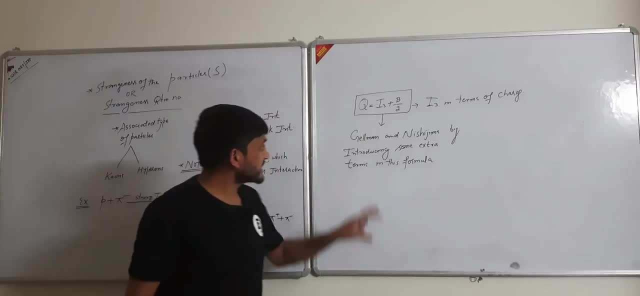 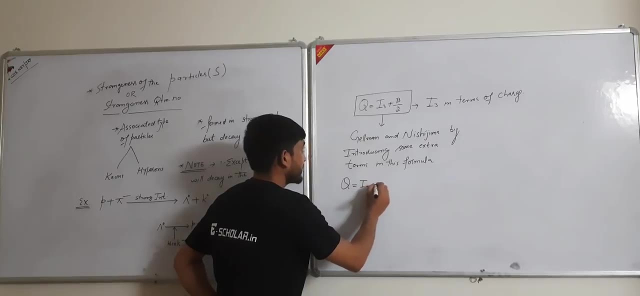 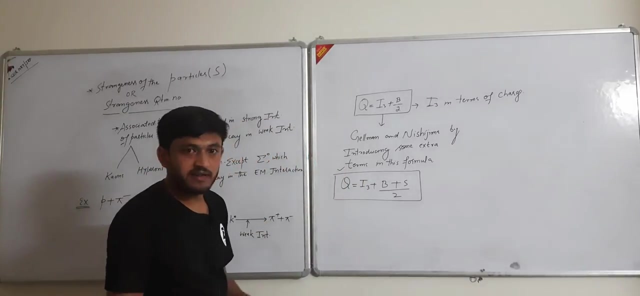 ok. Which new terms are added in this formula? I3 plus B. and new terms are introduced here S by 2, and according to this formula we can calculate the strangeness of all the strange particles. Here B is the barrier number. we have nenuble. 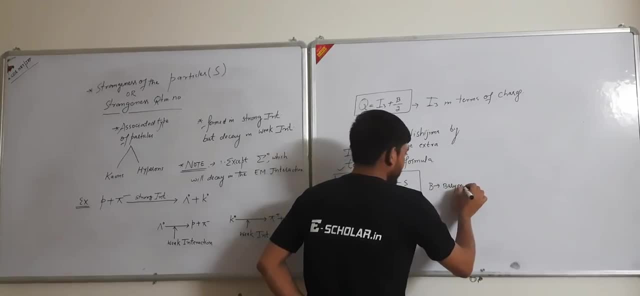 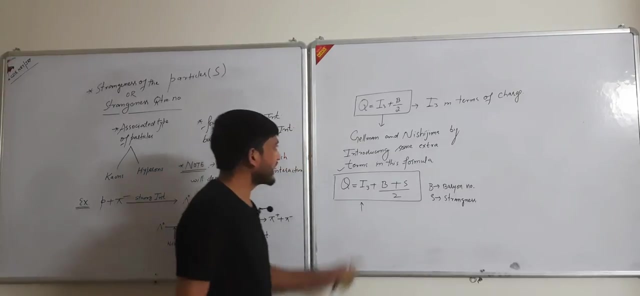 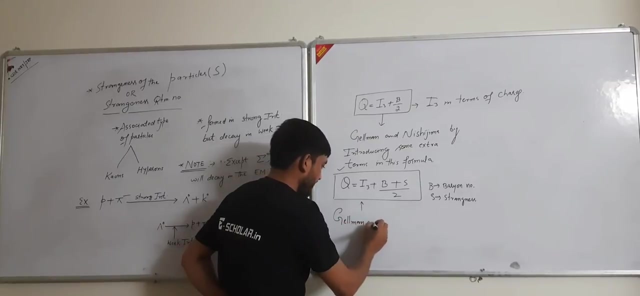 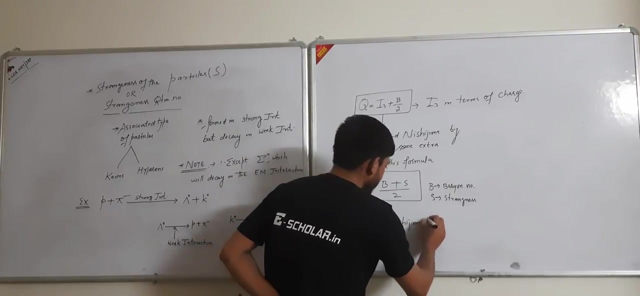 Total. So if I do this, we can calculate. the strangeness of all, the strangeness of number S is the strangeness, strangeness, And this formula called Gelman and the Nishijima formula. Which formula, Gelman and Nishijima formula. By using this formula, we can calculate. 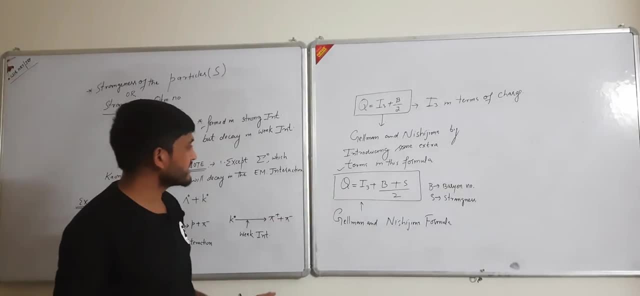 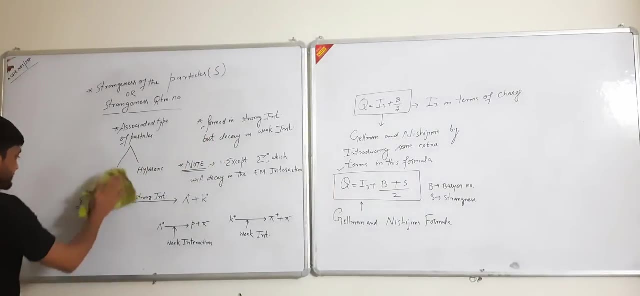 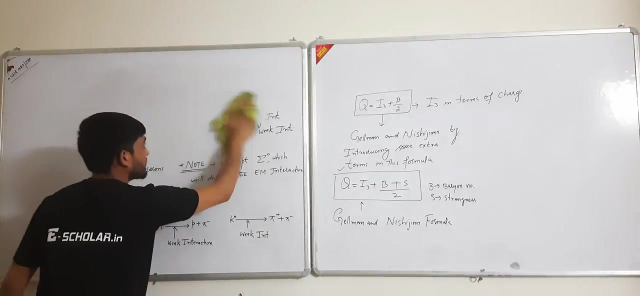 the strangeness of all the strange particles. Now let us see how we can calculate the strangeness of the different, different particles. Now see here. First of all, we have a need to know which type of the particles are strange particles. 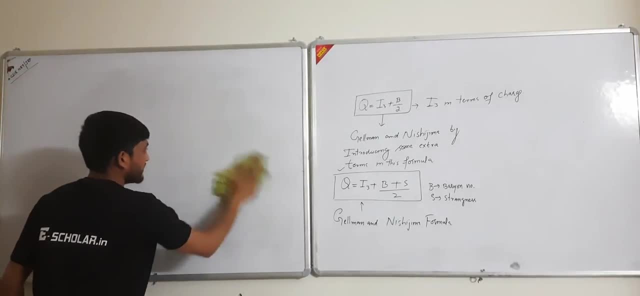 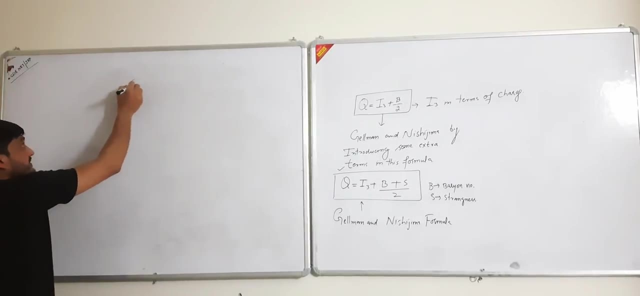 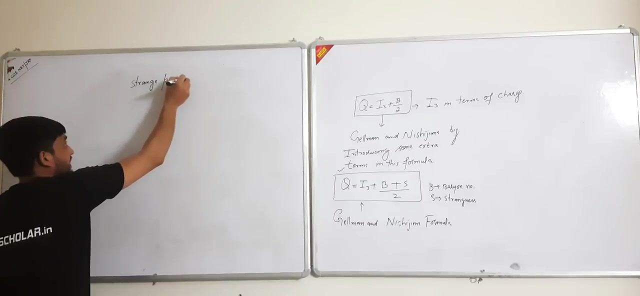 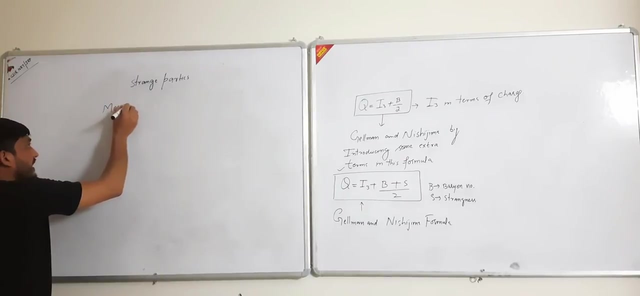 And then calculate the strangeness for all those particles. So strange particles are strange particles In mesons, only cands are the strange particles, only cands. that means k positive and k zero, this is the doublet- are the strange particles. And then variants: That is principled in basons. It is called Dinner right Diners for this. why don't not? you still know this, so you don't need to come again, But you can use it for everybody else. What was this? B 엄ko all Mu, when suddenly that means pasarne? 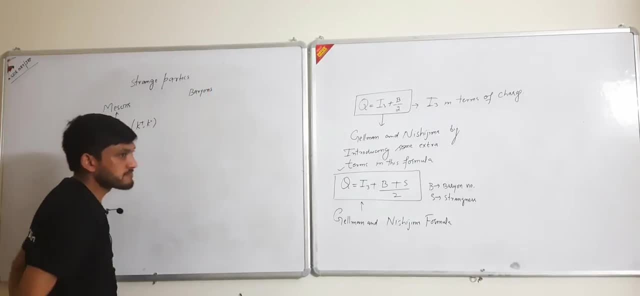 We already know that, but you can write in the columns: 하면uth demandeARA A grić, am nevertheless dir compañia ki does any. they also write in Chinese and other languages which make all these sorry hypraeons all the hypraeons are, because nucleons are not a strange particles and all. 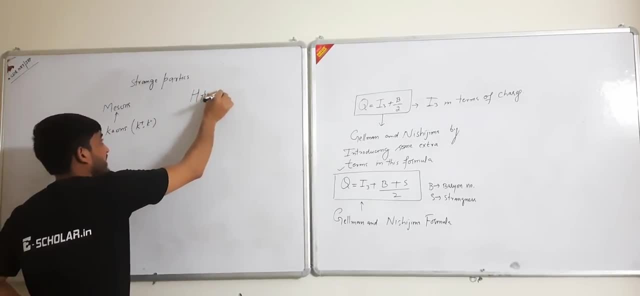 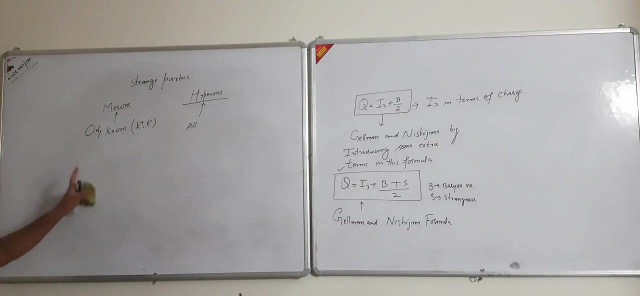 the hypraeons. second one is the hypraeons: all the hypraeons are the strange particles, all hypraeons, all. okay, now we can calculate the strangeness just like. first of all, start with the kaons strangeness for kaons. s are the value of s, value of s for kaons. 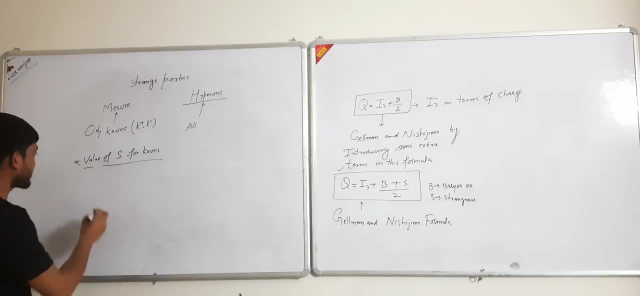 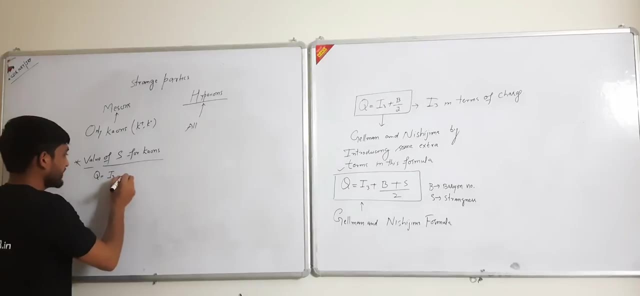 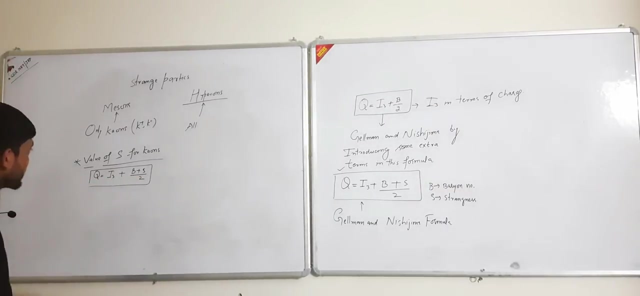 always okay by. according to this formula, ku is equal to i3 plus b plus s upon two, and here we have a need of need the value of b and i3 and then charge. so far I will taking counter Tapi 3 and then Silver 4. 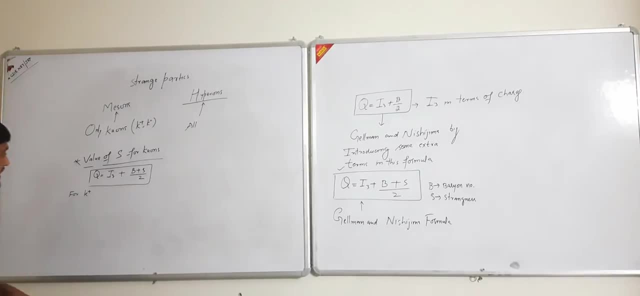 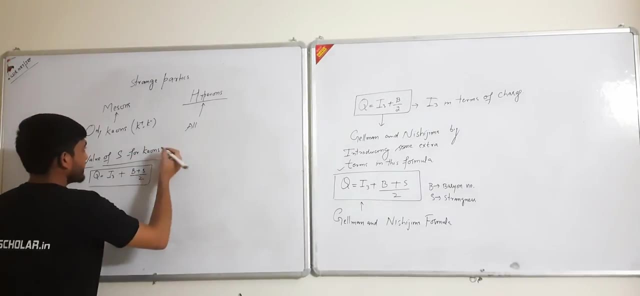 take the k positive. so first of all i have added to the value of i3 component. that means this is the doublet and this is the doublet and value of isospin 2i plus 1 is equal to 2. 2 is the multiplicity, because all the particles in the nature are in the form of multiplicity. 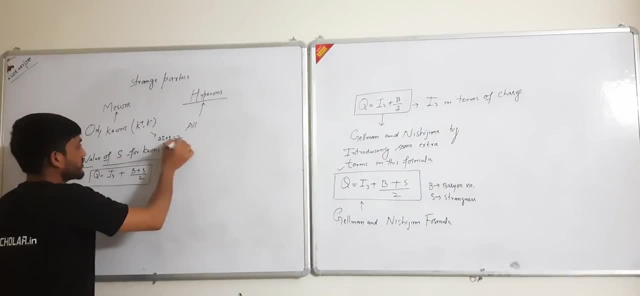 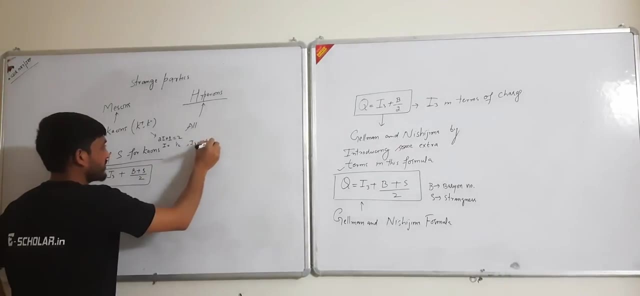 nature. so here is: value of i is equal to 1 by 2 and value of i3 is equal to plus 1 by 2 and minus 1 by 2. okay, so minus 1 by 2 for k0 and this is the k positive. then value of: 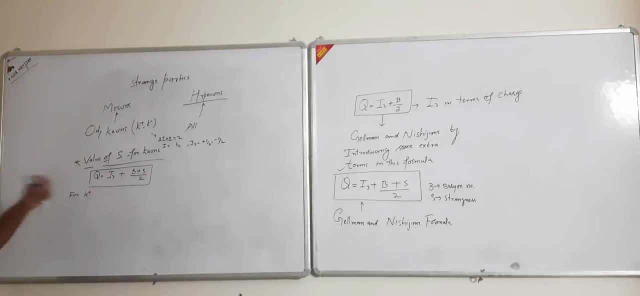 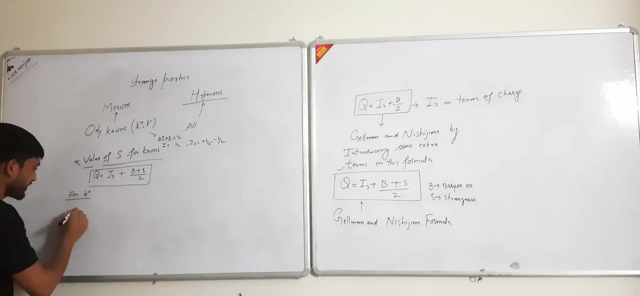 i3 will become plus 1 by 2 and value of charge- here is a charge- is the plus 1 for k positive plus 1.. So we have added to this formula is equal to value of i3 is equal to 1 by 2 plus this. 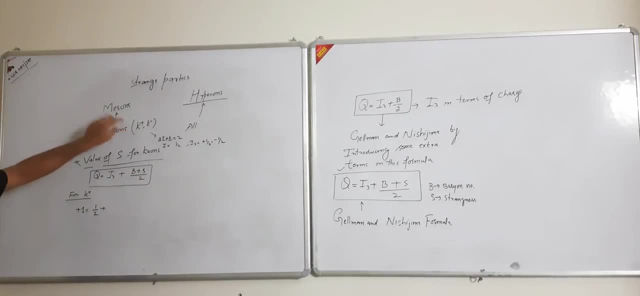 is the baryons, b is the baryon because this is the family of k positive or the family of mesons, then value of b is equal to 0 for mesons. okay, because only value of b is equal to 1 for only baryons. 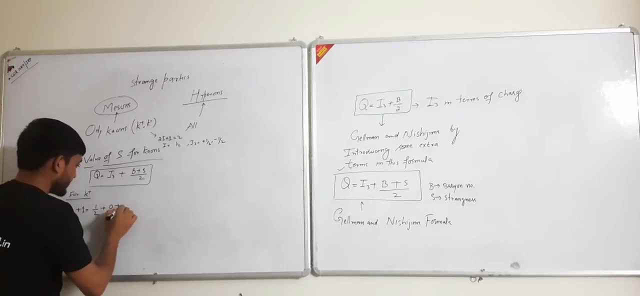 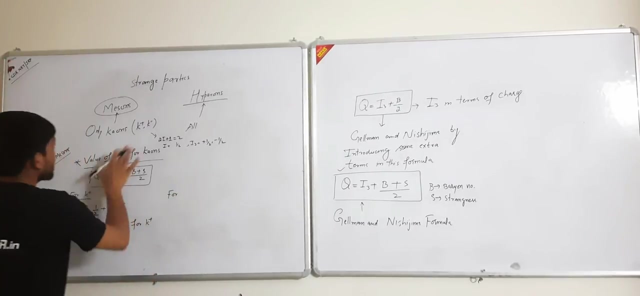 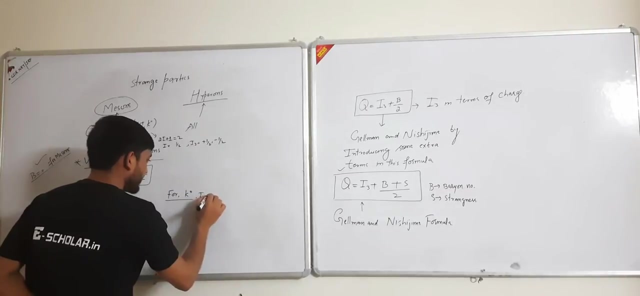 then value of b is equal to 1. for k baryons are of 0.. 0 plus s1, 2, s1- 2 and value of s is equal to 1. for this is the strangeness: value of s for k positive, second for k negative. sorry for k0. value of i3. here value of i3 is equal. 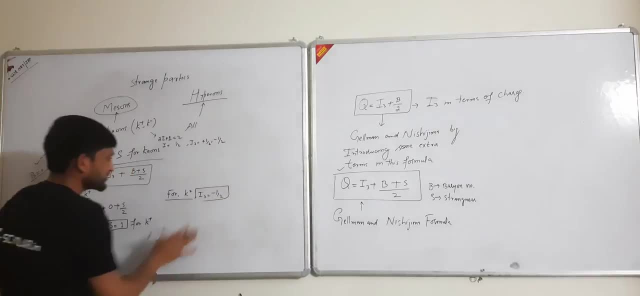 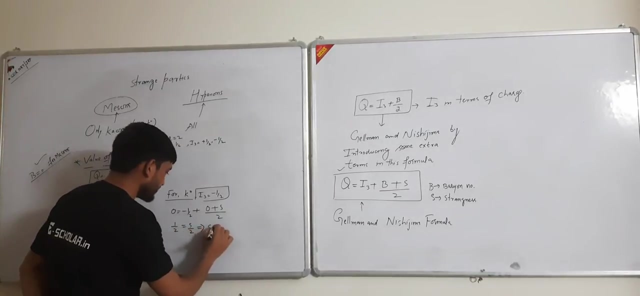 to minus 1 point 2. put these values in the in this formula. so here charge is 0 and value of i3 is equal to minus 1 point 2, plus barrier number is equal to minus 1 point 2.. 0 plus s1, 2- ok, now 1 by 2 is equal to s1- 2. and here is also s1 for k0- ok, now here value. 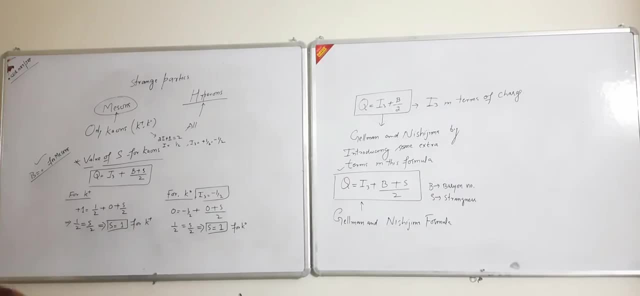 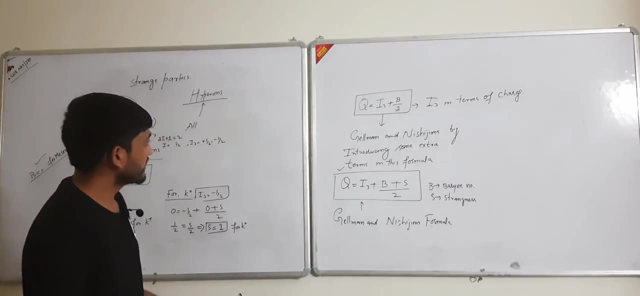 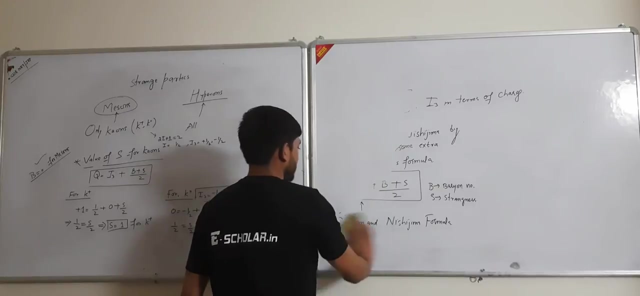 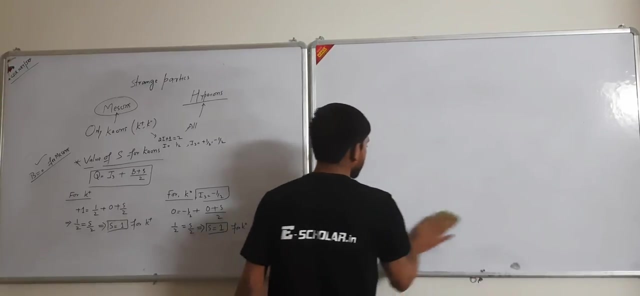 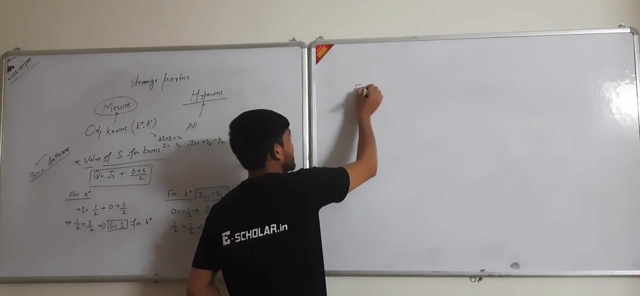 of strangeness. it means value of strangeness. number will remain positive, 1 for k0.. Now, next one is the sigma. sigma is the triplet and value of i3 for all the sigma for sigma positive value of i3 is equal to plus 1. here value of i3 is equal to minus 1 point 2 and 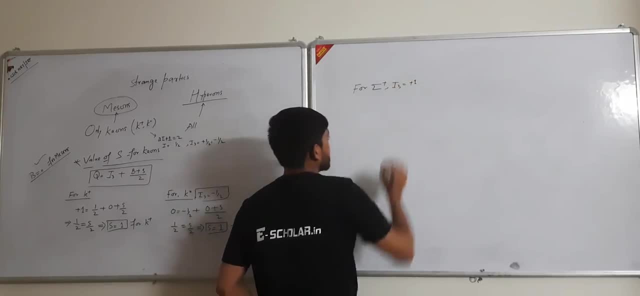 value of i3 is equal to plus 1 point 2. ok, and according to this formula, charge is here: plus 1 is equal to i3. 1 plus sigma positive is the variant 1 plus s upon 2. 1 and 1 will. 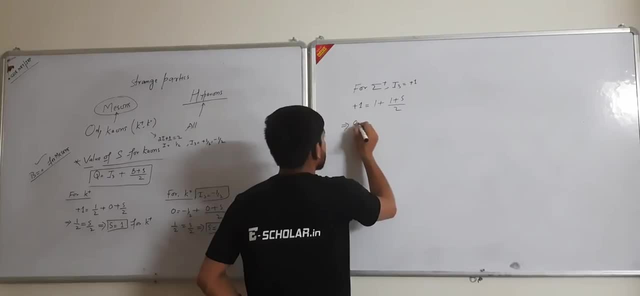 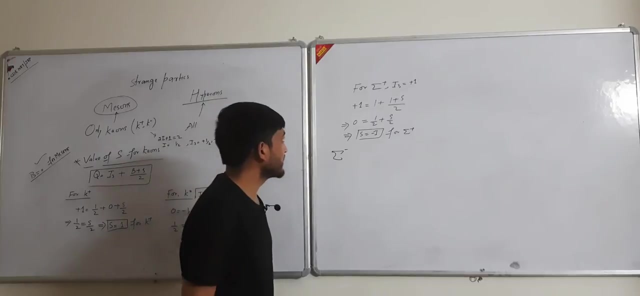 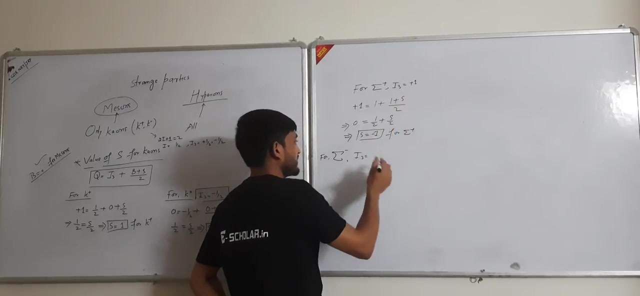 become 0.. s1, 2 and s is equal to minus 1 for sigma positive and next one is the sigma negative. sigma negative value of i3 for sigma negative value of i3 is equal to minus 1. okay, and put these values in this formula. 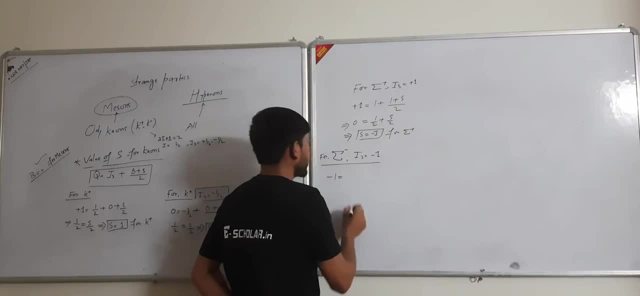 so charge is: the minus 1 is equal to value of i3, is equal to minus 1 plus 1 plus s1 2, because this is the variant on 1 and minus 1 and minus 1 cancel and then minus 1.2 is equal to s1 2. 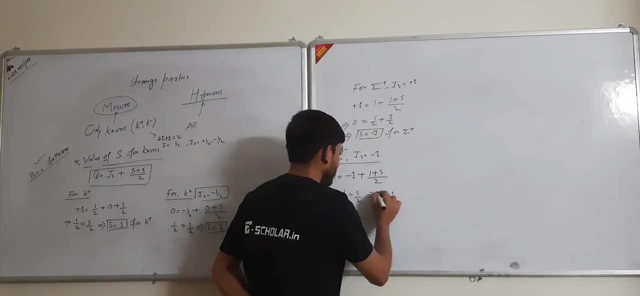 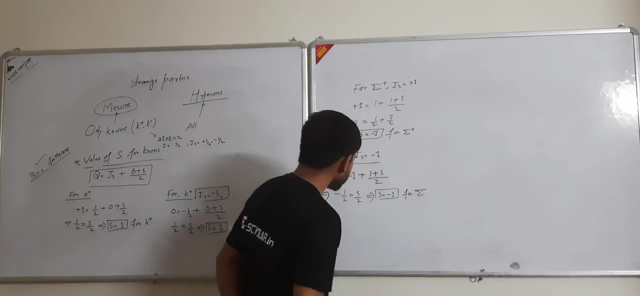 minus 1.2 is equal to s1. 2 minus 1.2 is equal to s1. 2, which implies s is equal to minus 1. for sigma negative, and then next one for sigma 0. sigma 0 value of i3 is equal to 0. here charge is also 0. 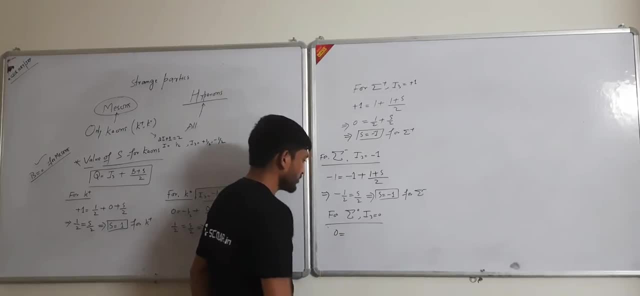 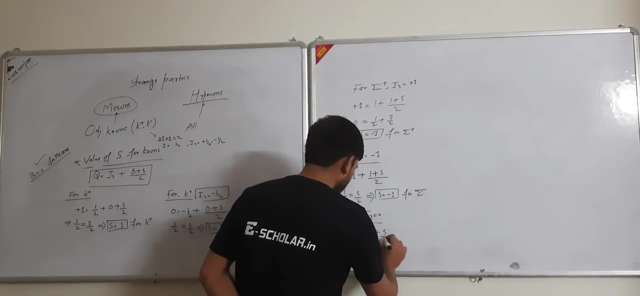 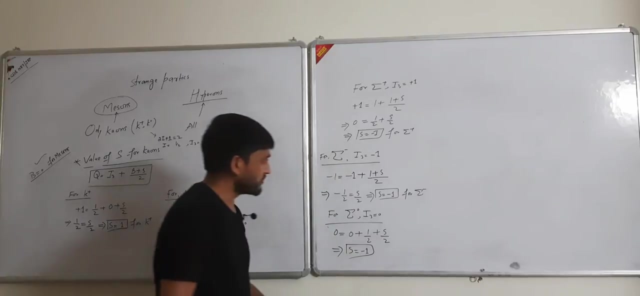 then according to formula, 0 is equal to i3 component is equal to 0 plus 1.2, and plus 1.2 s 1, 2. so here value of s is also minus 1. it means value of the strangeness contour. 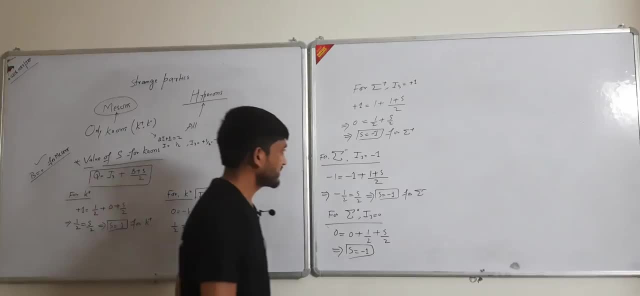 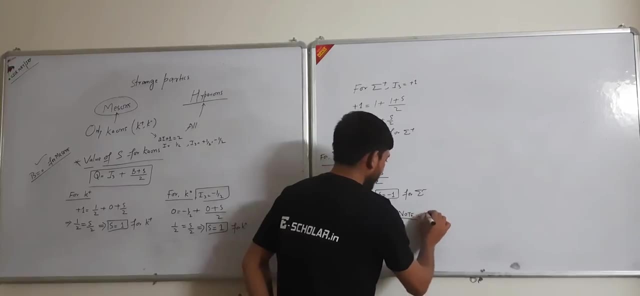 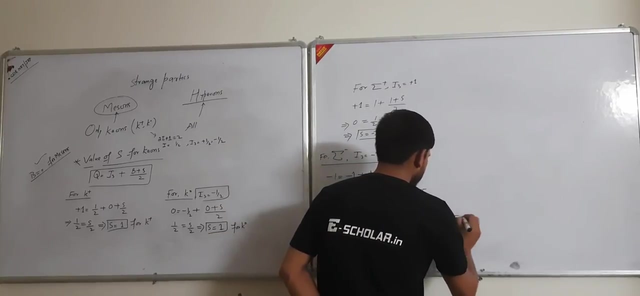 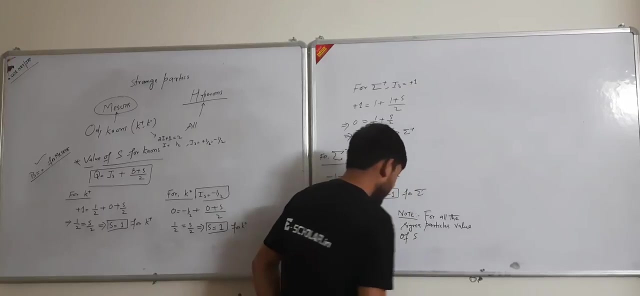 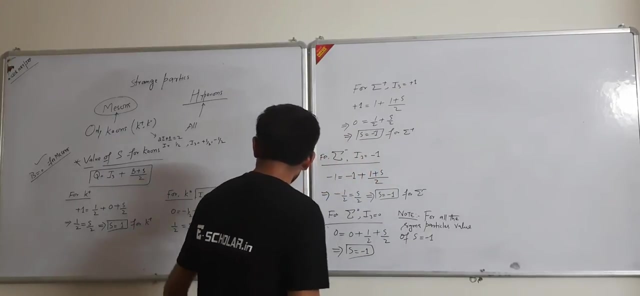 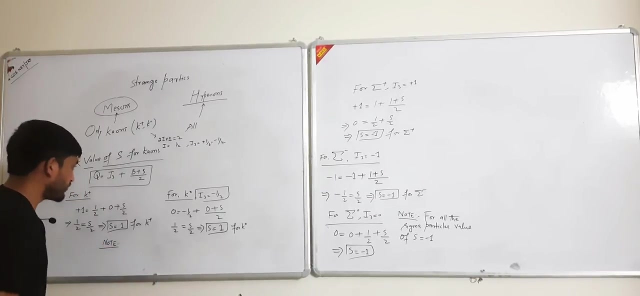 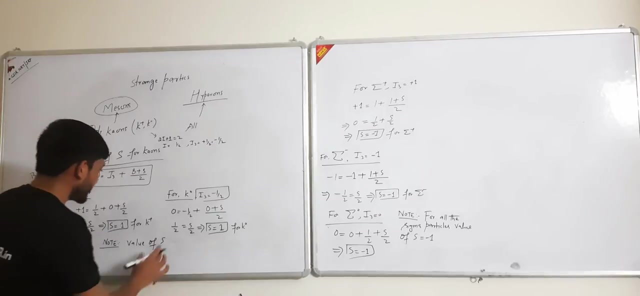 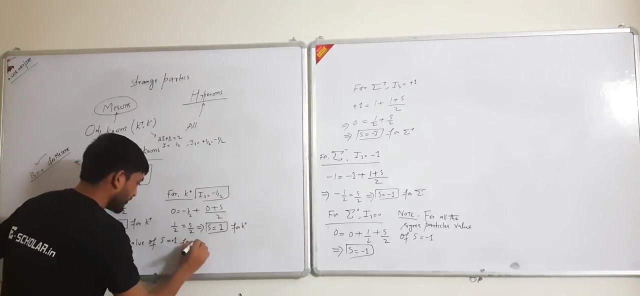 number will remain minus. 1. for all the Sigma: okay, for all Sigma node. for all the Sigma particles: Sigma particles. value of strangeness contour number: that means s is equal to minus 1. okay, and here is also note. value of s is the strangeness contour number will remain positive. 1 for all the. 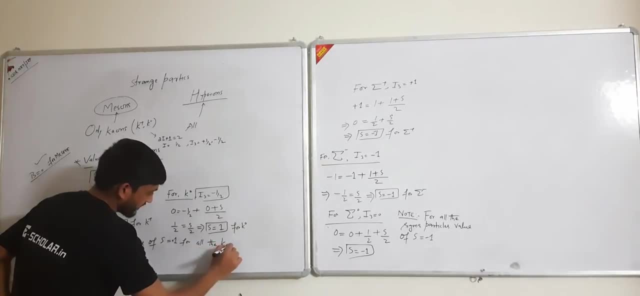 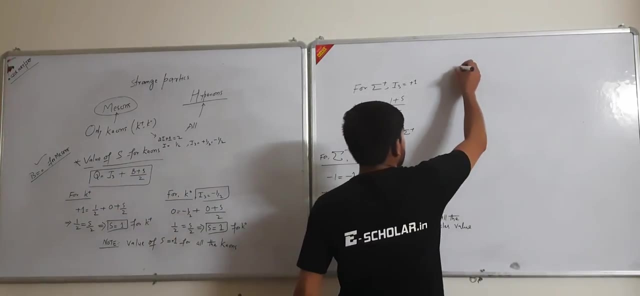 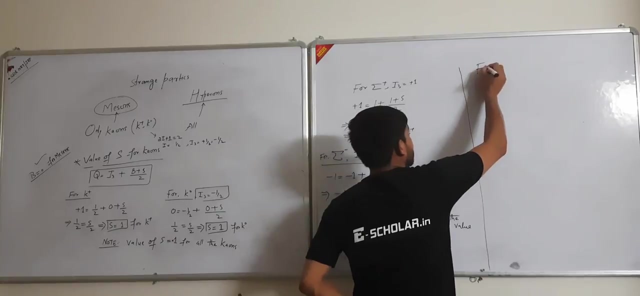 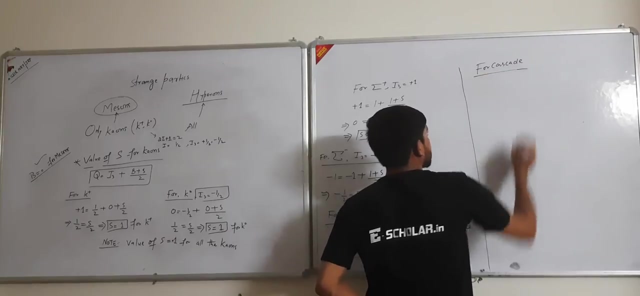 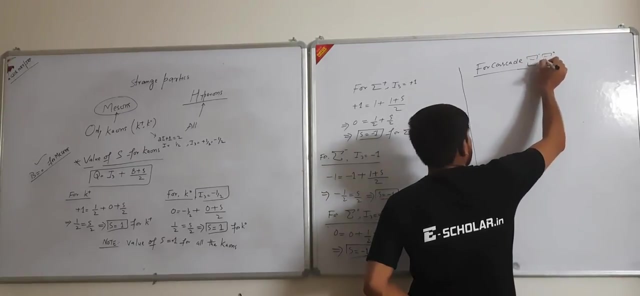 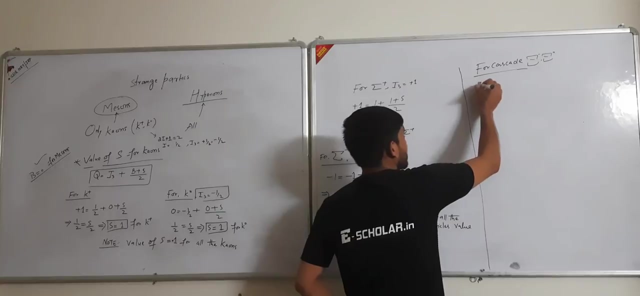 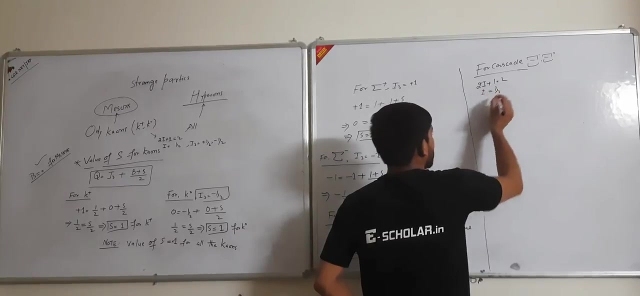 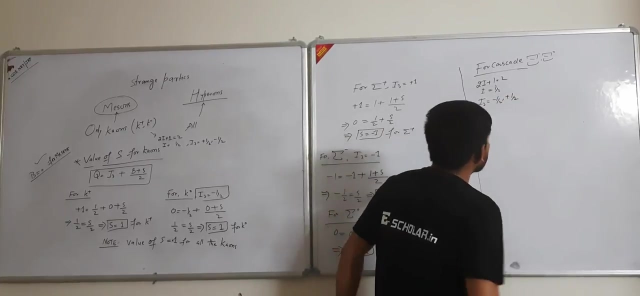 Kearns, all the Kearns now move towards for the cascade, for cascade. cascade means negative and zero. so I3 component for this cascade I is equal to two, i Heveler 1 is equal to two. doublet value of i is equal to 1.2 and i3 component is equal to minus 1.2 and plus 1.2. 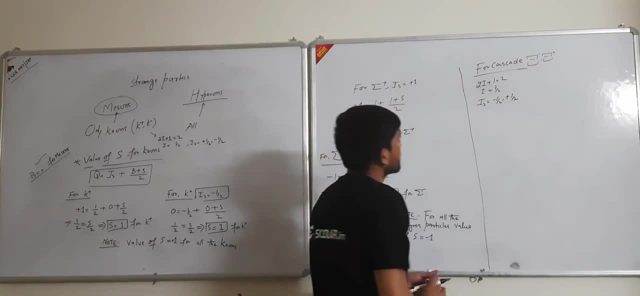 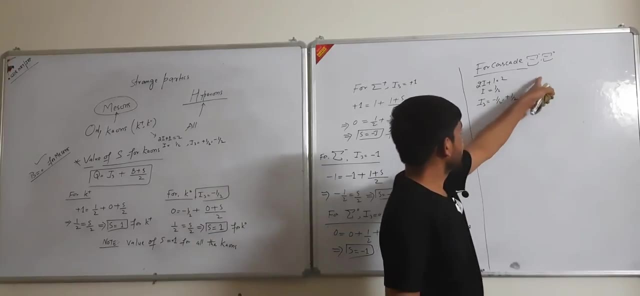 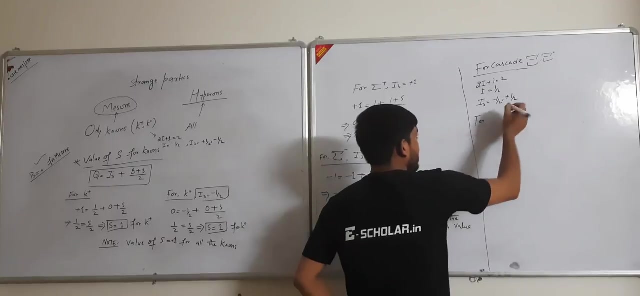 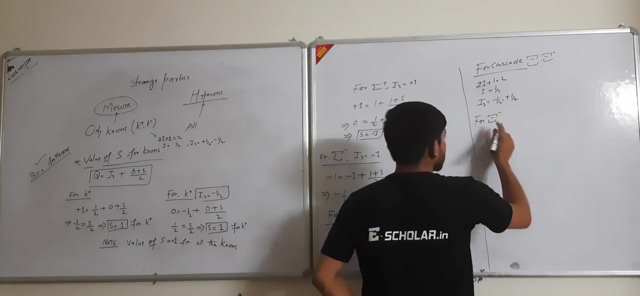 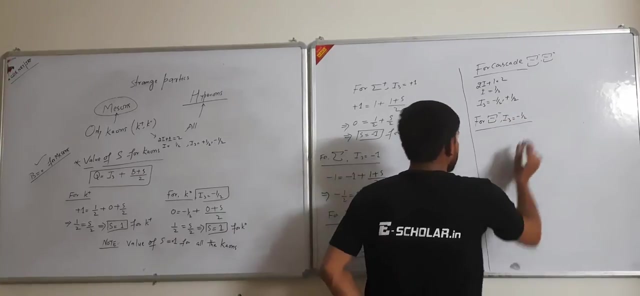 that means for negative value of i3 is equal to minus 1.2 and for 0 value of i3 is equal to plus 1.2. so for sigma negative- sorry, cascade negative- i3 is equal to minus 1.2. okay, so put these values. 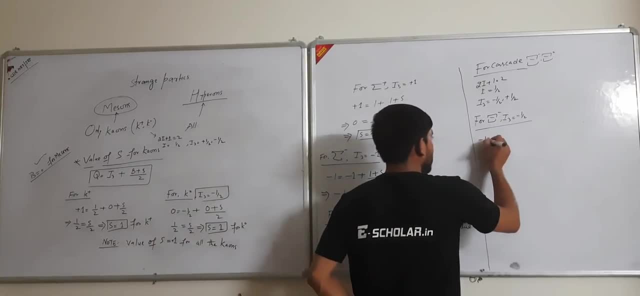 in this formula here charge is the minus 1 and i3 is equal to minus 1.2 and b is the variant. this is the variant and value of b is equal to 1 by 2 plus s.2. now value will become minus. 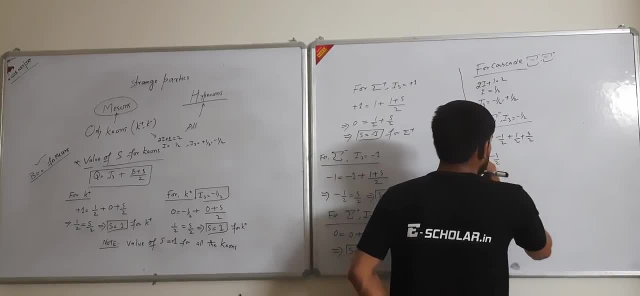 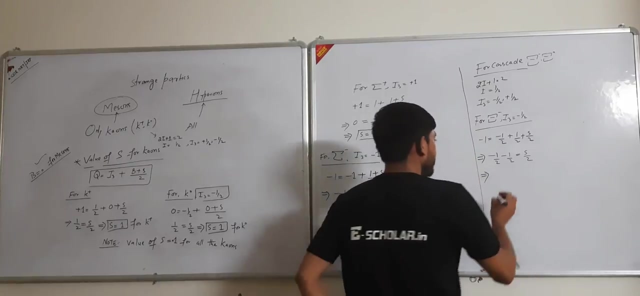 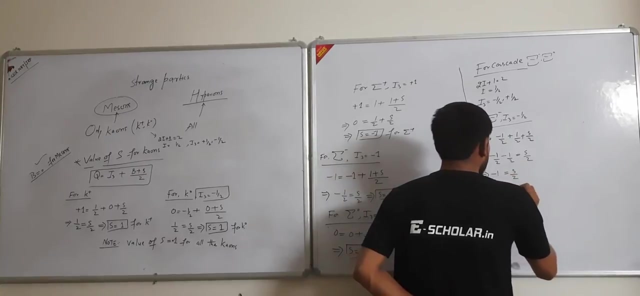 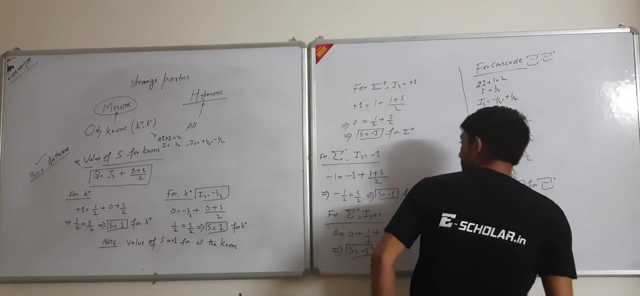 1.2 and minus 1.2 is equal to s.2, which implies value of s is equal to minus 1 s.2 and s is equal to minus 2. for cascade: okay, and then for cascade 0, i3 is equal to plus 1 by 2. put in this formula here, charge is a 0. 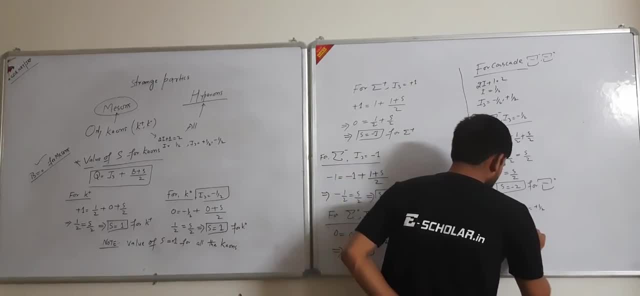 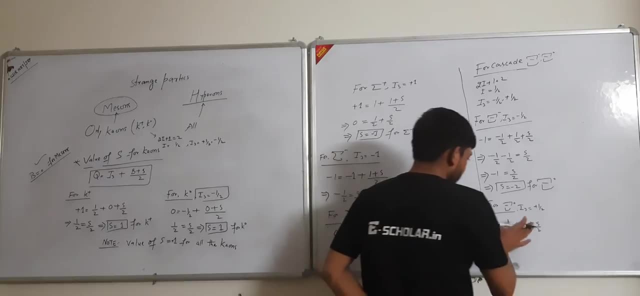 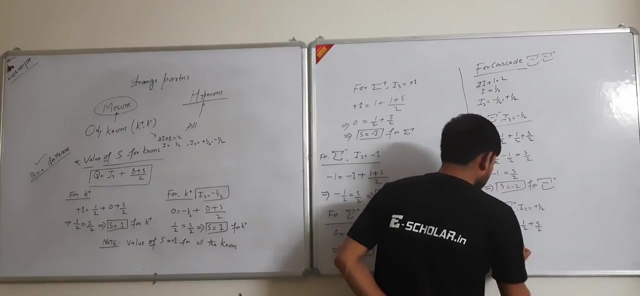 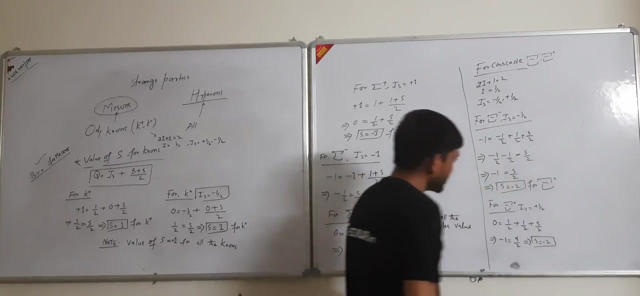 plus 1 by 2, plus 1 by 2, because this is the baryon, and s1 2. okay, so this is the 1 minus 1 is equal to s1 2, which implies s is equal to minus 2. it means value. 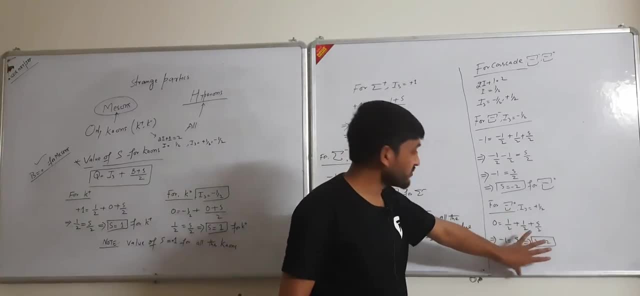 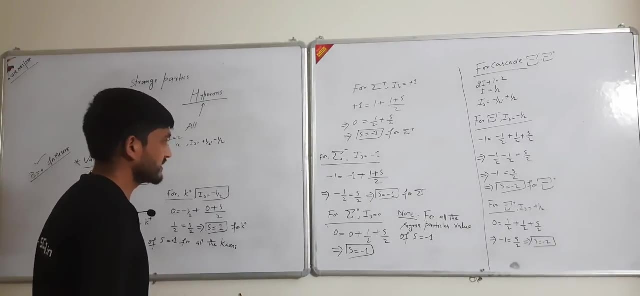 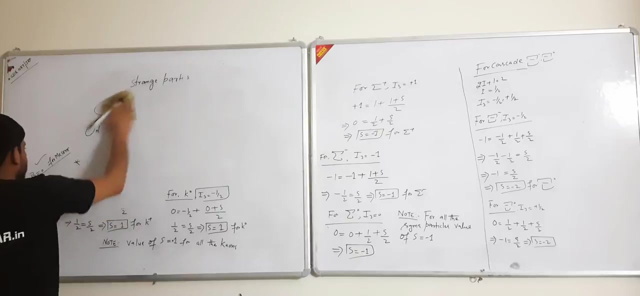 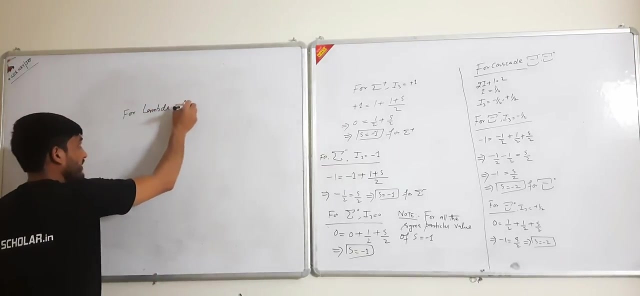 of the stangeness, quantum number for the cascade is equal to, s is equal to minus 2, and next one is the lambda, and then omega lambda, and omega lambda is a singlet and omega is also singlet. lambda for lambda for lambda, this is the singlet, and here value of isospin is equal. 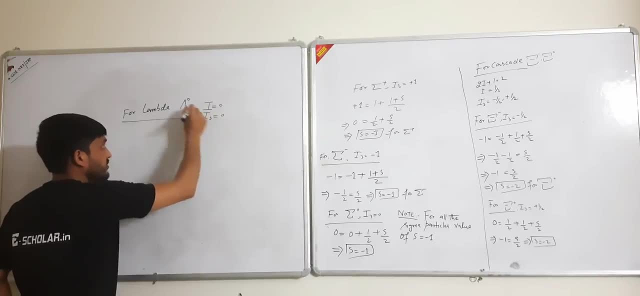 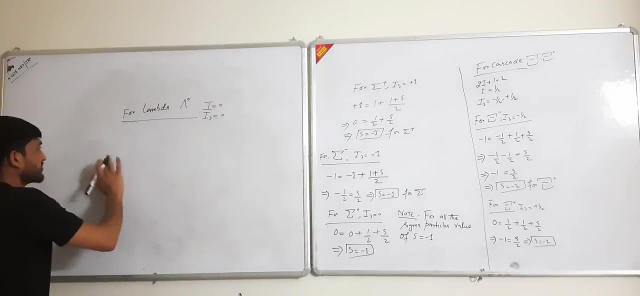 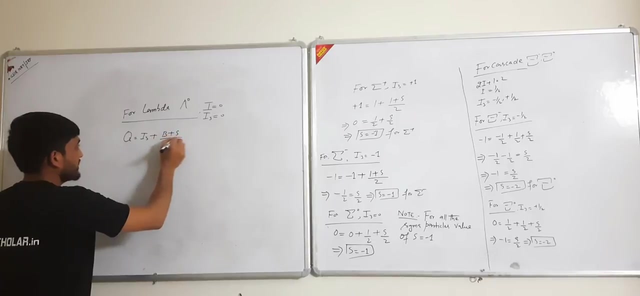 to 0 and i 3 component is also zero for the lambda. and then calculate the value of stangeness. quantum number carded to the formula. q is equal to i, 3 plus b plus e, s1- 2. this is the Galman-Allen-Neshezema formula. here value of q is equal to 0, i3 is also 0. 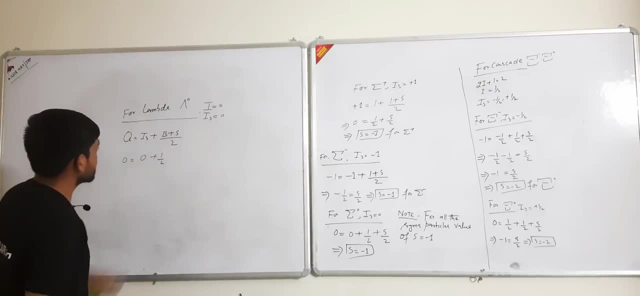 plus 1 by 2, and this one is the plus s1 2. then value of s is equal to minus 1, for lambda: 0. and then next last one is the for sigma negative. this is also singlet, and for singlet value of i is also 0 and i3 is also 0. 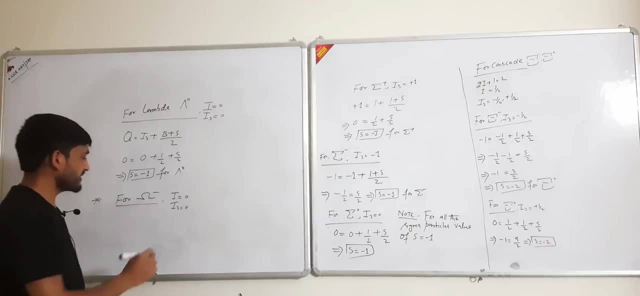 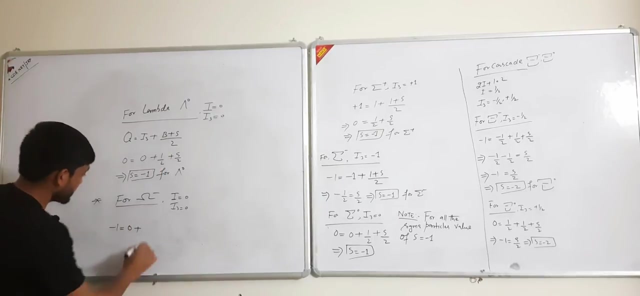 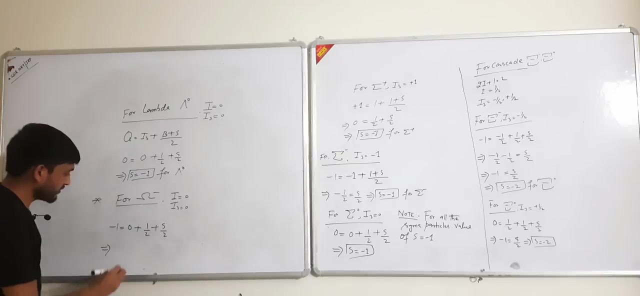 i3 or iz, third component of the isospin. so value of strangeness, contour number will become here: charge is the minus 1. i3 component is the 0 plus b. this is also baryon plus s by 2, and then value will become minus 3. 1. 2 is equal to s1, 2, which implies s is equal to. 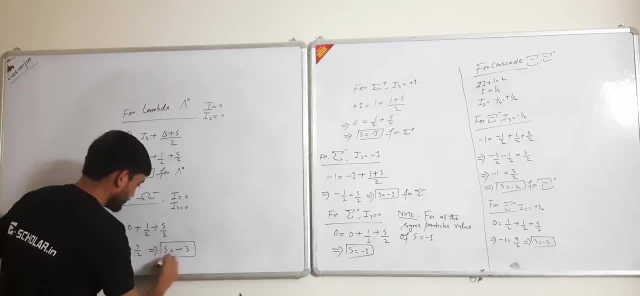 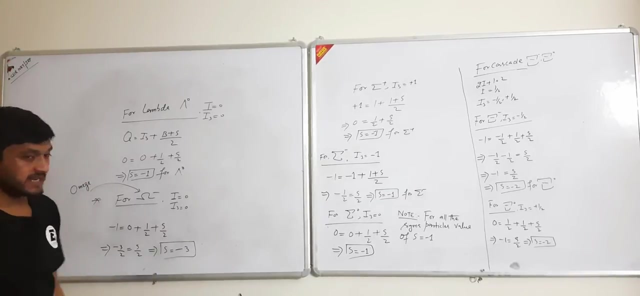 minus 3. it means value of the strangeness contour number for the- this is the i3 component- is the 0 plus b- this is also baryon- plus s by 2, and then value will become omega. nothing but a. omega. omega is equal to s is equal to minus 3. it means value of s is equal to minus 3 for omega. 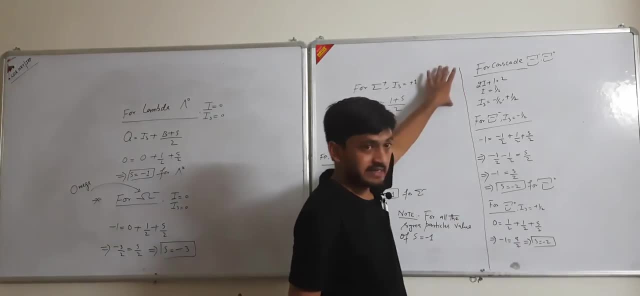 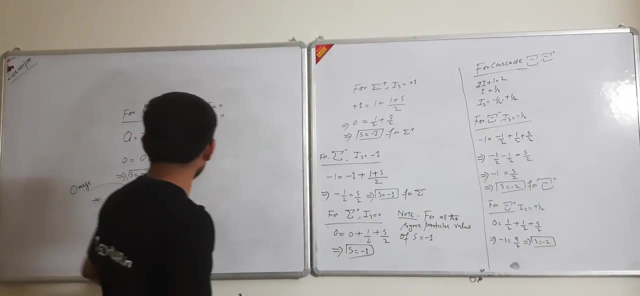 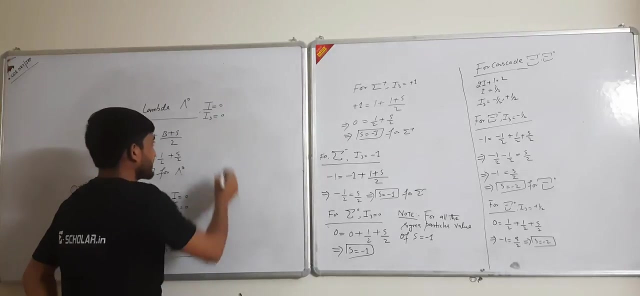 and value of s is equal to minus 2 for the cascade and the value of s is equal to minus 1 for the sigma and second one is the lambda okay and value of k is equal to. that means- it means note- s is equal to plus 1. 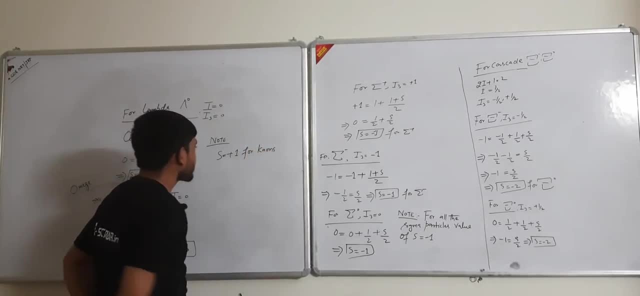 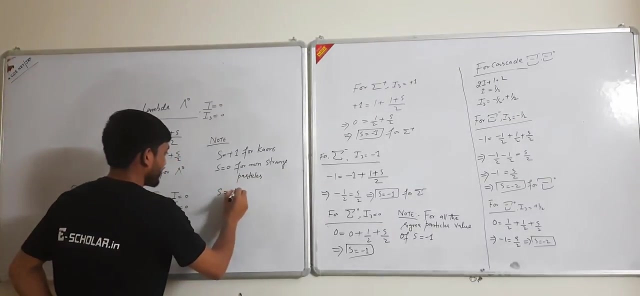 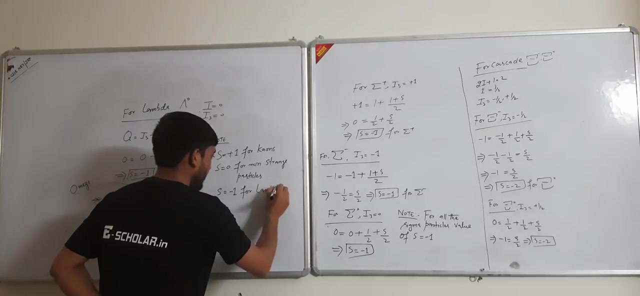 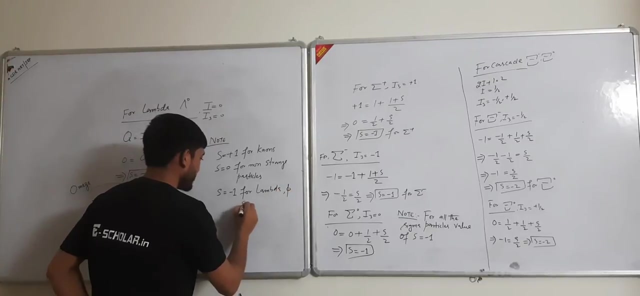 for k conventions: s is equal to zero. for non-strange particles: for non-strange particles: for non-strange particles and value of s minus 1. for first one is the lambda and second one is the sigma lambda and sigma, s is equal to minus 2. for which type of the particle s is equal to minus 2? 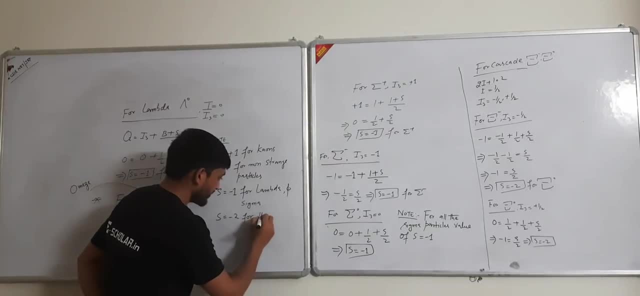 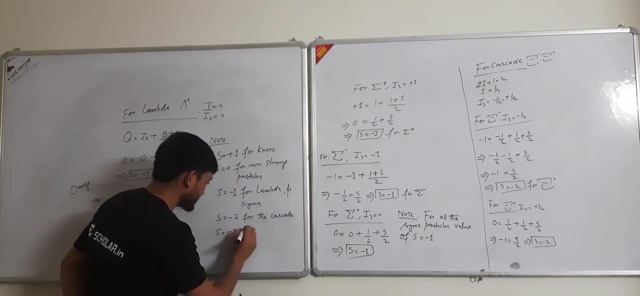 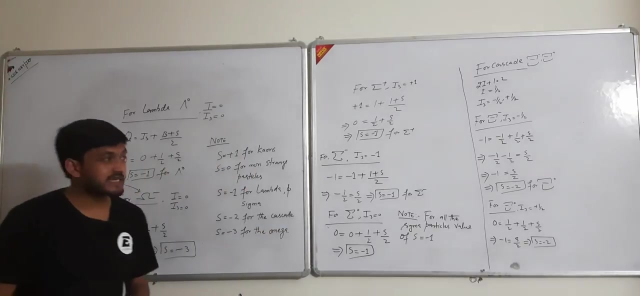 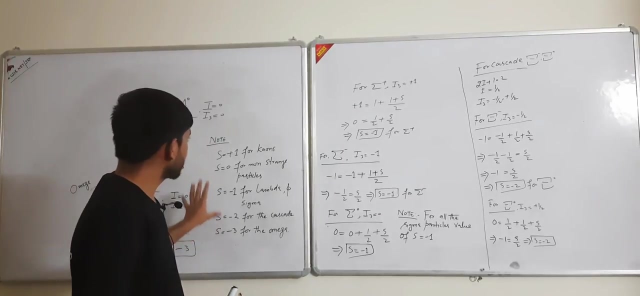 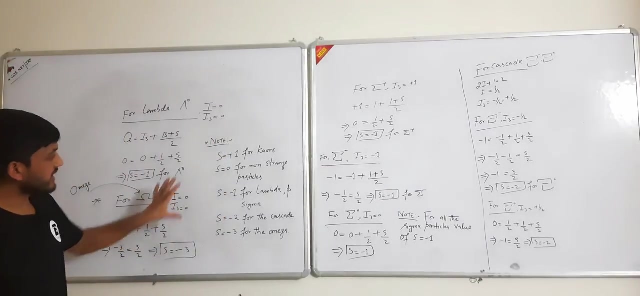 for the cascade. for the cascade and s is equal to minus 3 for the omega. so this is the method how we can calculate the strangeness of the strange particles. and isospin are third component of the isospin. so these are the basic method to calculate the isospin and remember these. 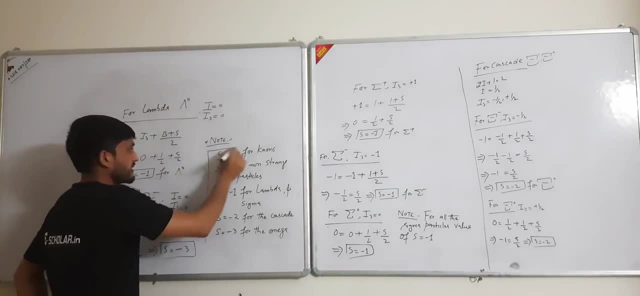 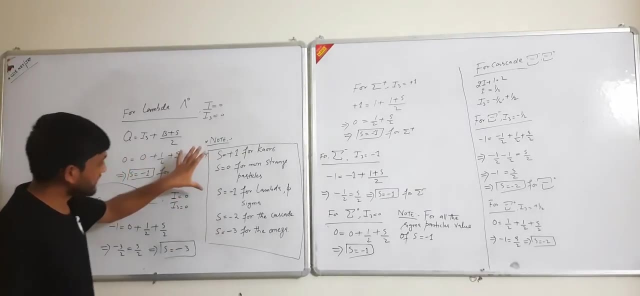 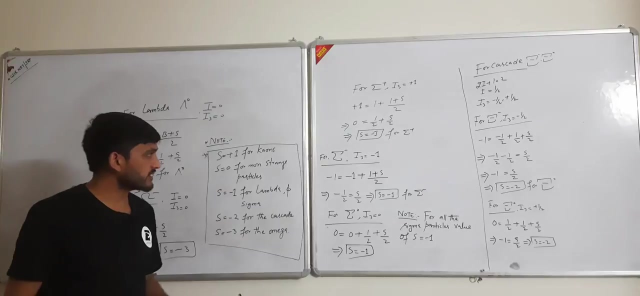 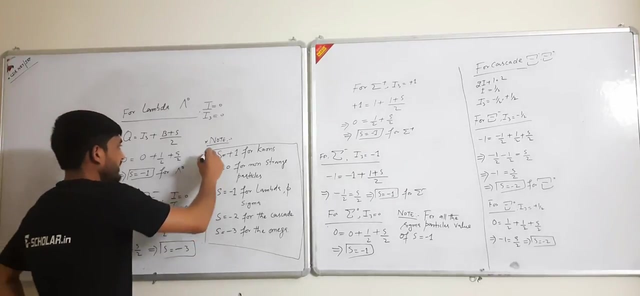 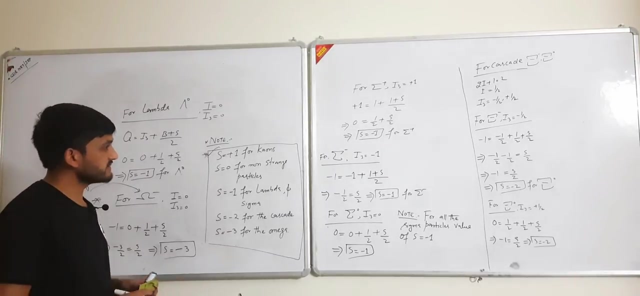 remember these formulas, because if we remember these you can calculate all these calculations. then it mean we can easily calculate the numerical problem. then we have no need to calculate all such mathematical calculations. you can shortly put the values of s for the different particle directions. okay, now next one is: 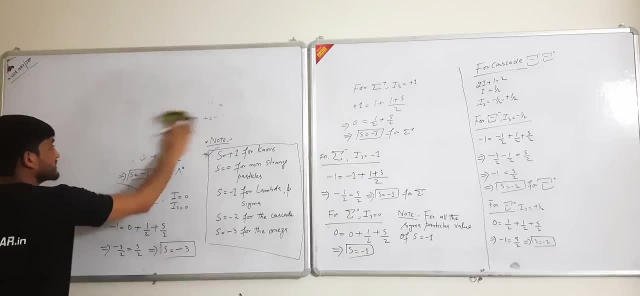 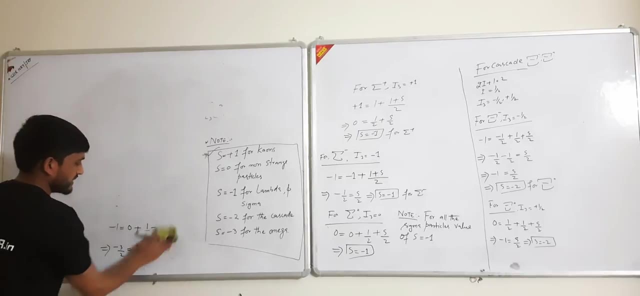 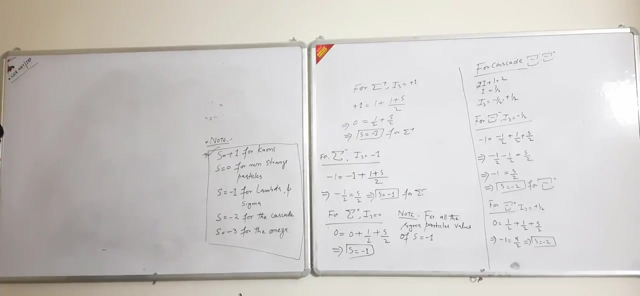 some selections rules. which type of selection rules or applicable topic is that select его? which type of selection rules or applicable topic is that convey all theseedes of the constant ahl mixedh of theи are applicable in the elementary particle reactions. so note these selection rules, these. 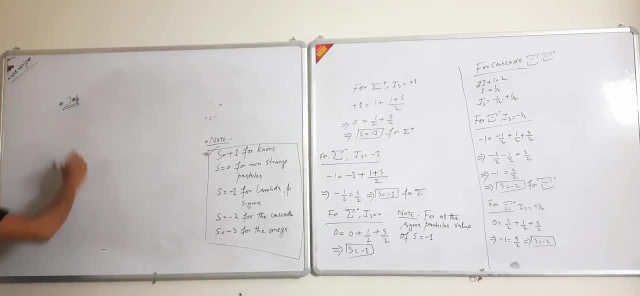 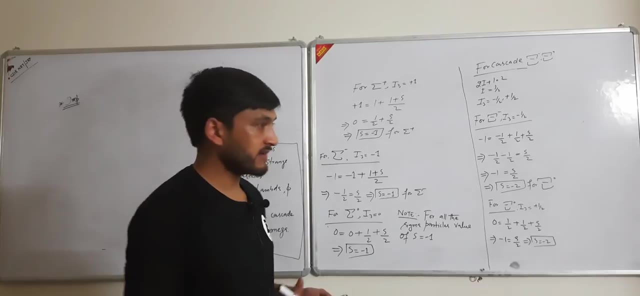 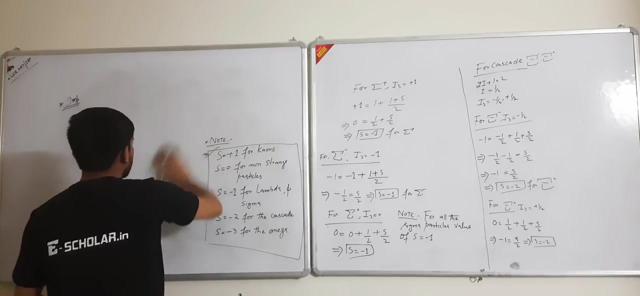 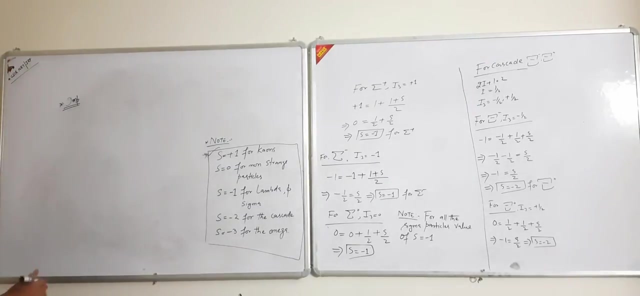 are the most important selection rules to check whether the reaction is allowed or whether the reaction is electromagnetic or strong type of interactions and which are B type of interactions according to isospin, third component of the isospin, and then the strangeness contour number. so first selection rule on the basis of strangeness contour number. if 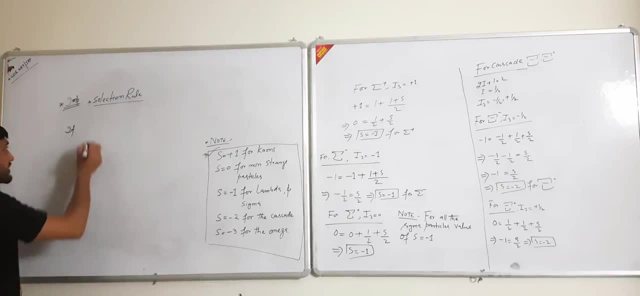 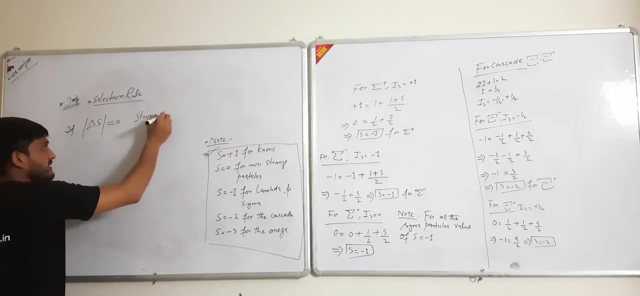 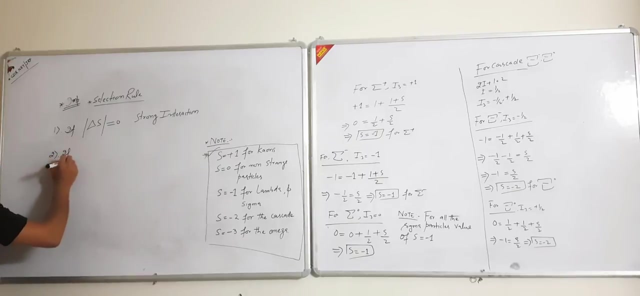 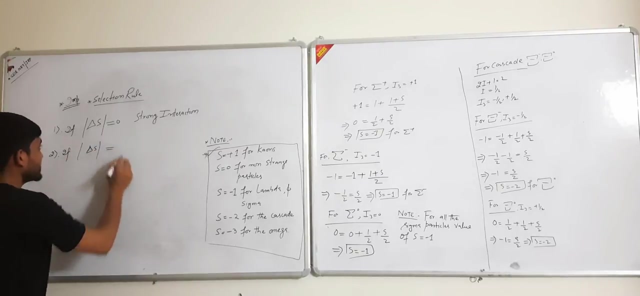 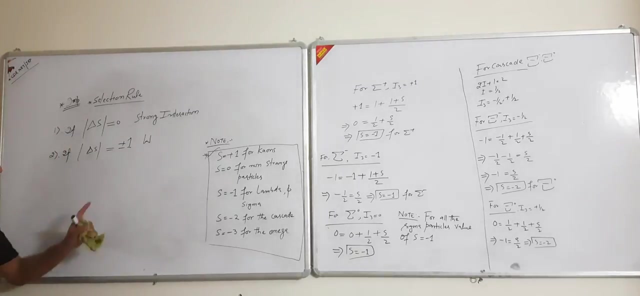 we have a change in strangeness. number is equal to zero. strong interactions will occur. follow strong interactions. strong type of interactions are introduced here. strong interaction, second one. this is the first one. second one, if. if ientôt now change in theホmee 相 lower.